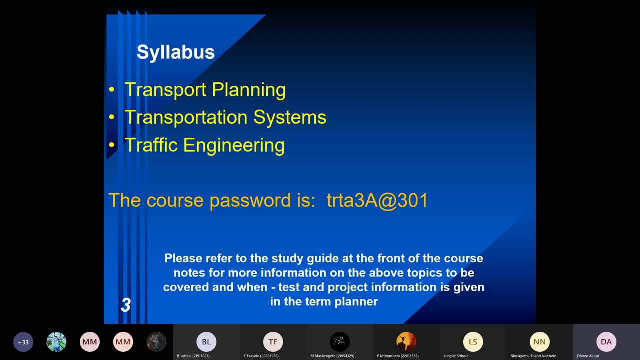 been loaded onto MS Team as well. With regard to the three main chapters, that's reflected here. transport planning covers theory aspects, so the theory is covered in transport planning. Transportation system also covers a fair amount of theory. with some calculation And you will find that your first 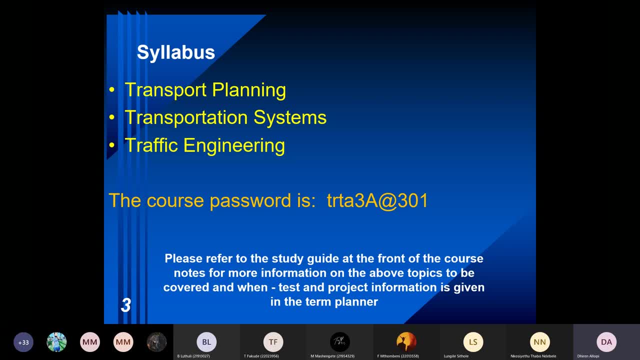 test then will cover transport planning and transportation system. So with regard to the first test, you will find there is fair amount of theory, could be anything up to 60 percent, with the balance made up of calculations: transportation systems, calculations. the third chapter, traffic engineering, is mainly calculations. 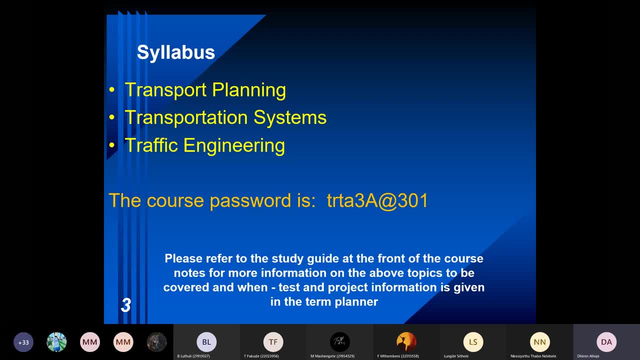 mainly calculate calculations. of course some theory, and your test too will cover traffic engineering only okay, and you all know that at the exit level you have to satisfy engineering council of south africa. that's exa's graduate attributes, ga. now, if you went through the study guide, you will find that not all but many of your exit level subjects cover a particular 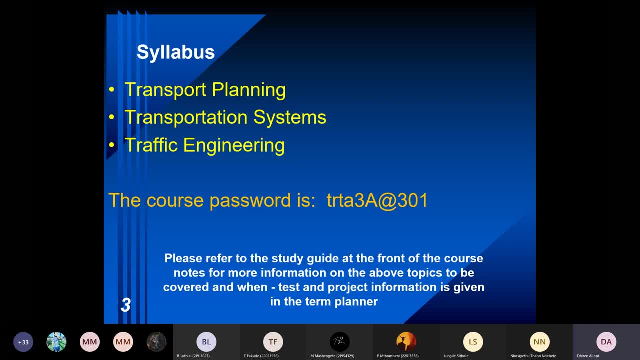 three a, you need to satisfy graduate attribute four, ga4, which deals with investigation, data analysis and so forth. so that is covered in test two. so test two basically assesses your graduate attribute ga4. okay, what is also very important to note with regard to test two, you must achieve: 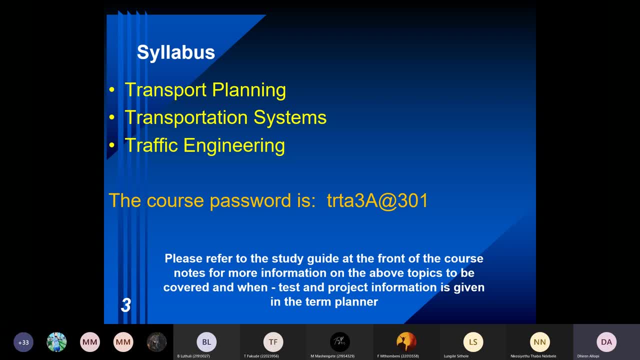 a minimum of 50 percent. so sub minimum rule applies: you must achieve a minimum of 50 percent in your ga test, which is test two. failing achieving 50 percent, unfortunately that means you will not be granted a dp, a course mark, to write the final exam. so please take note of that. and there is more. 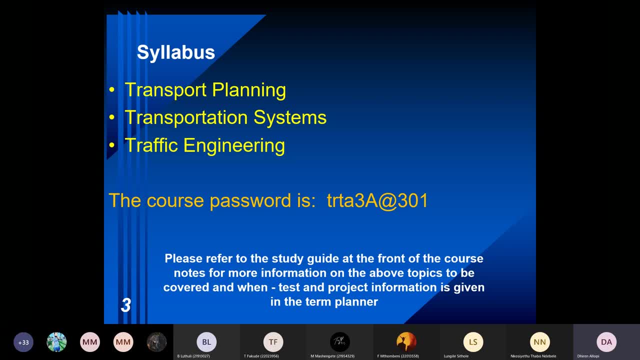 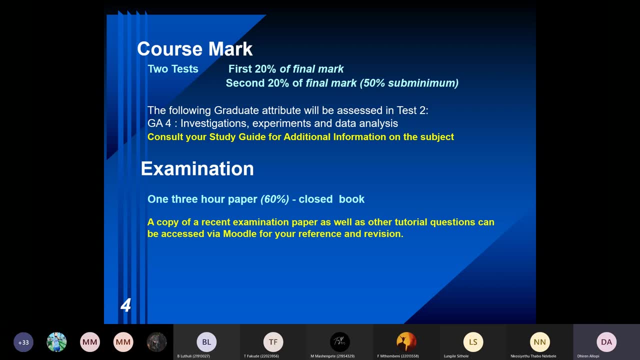 information in your study guide with regard to your graduate attribute and assessment. so your course mark, then, is based on two tests: first test we spoke about, which covers your chapter one and two, transportation planning and transportation systems, and at this stage, i also want to mention to you that it would certainly be in your best- 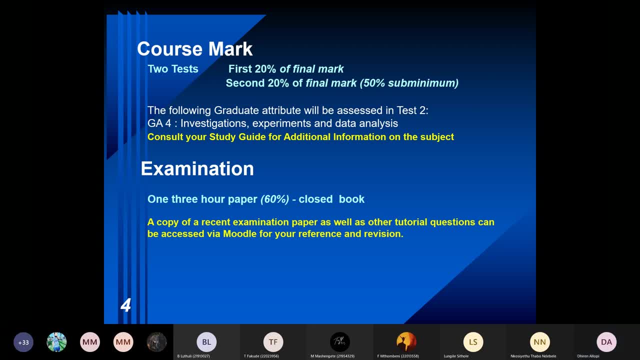 interest to write the schedule test. we all know it's so easy to get a doctor's certificate: any spaza shop will give you a doctor's certificate. but be in mind, if you don't write the schedule test- which means yes, with the doctor's certificate, you're now eligible to write the special test. 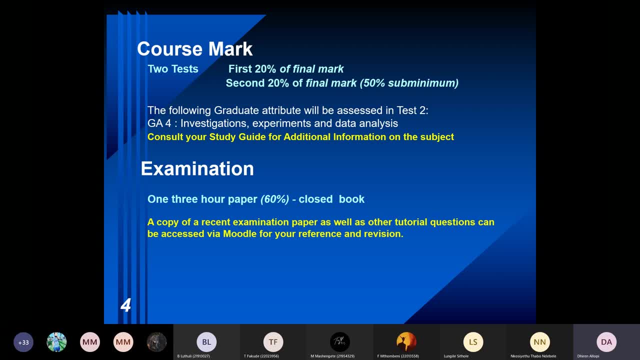 that special test is set at the end of the semester and could cover any aspect of your degree, of the syllabus, the whole syllabus and from past steps which, if you want, i can share with you. pass rate in the special test is in between five to ten percent. i don't think you want. 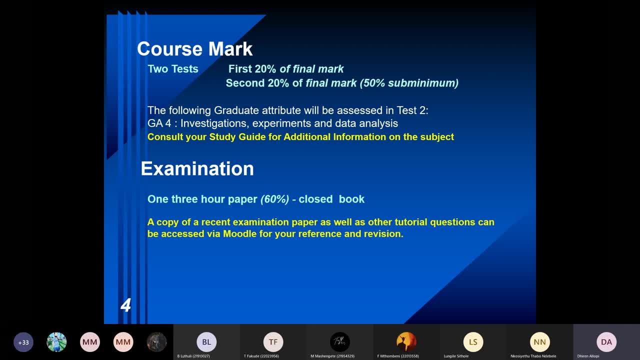 to be exposed to that. by writing the schedule test, you're only covering the first two chapters and the pass rate in the schedule test is always above eighty percent from past stats, so something for you to take note of. same obviously applies to the second test, so you can. 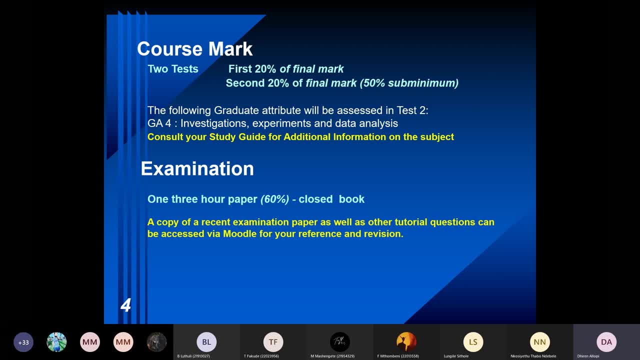 see the note, the graduate attribute ga4, which deals with investigation experiments, data analysis, and that will be then assessed in test two. so at the end of your program you should have satisfied all of xr's graduate attributes. previously there were 10 gas. we have now added the 11th ga, ga11, which 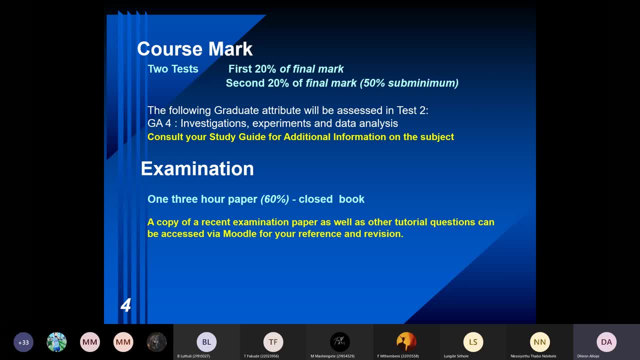 deals with management, engineering, management. so if you go through all your subjects you can pick up where the various gs will be assessed. i know in your design project a couple of ga's are assessed in your design project, more than one. so that's basically in terms of the assessment examination. yes, we, at this stage we are looking at. 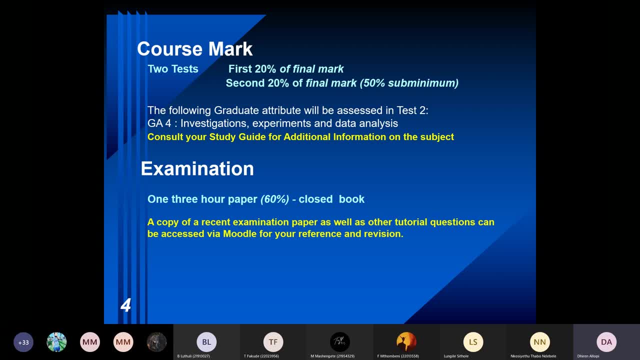 an exam on the site exam, like your test. three hour exam that will constitute 60. it's a closed book exam. an annex chair will be attached to the question paper and if you go on to moodle you will see a copy of the annex. chart model. 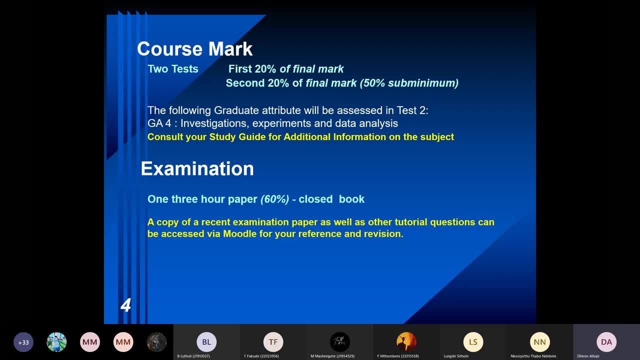 and i suggest that you look at that annex chin, get familiar with that annex chair, so that you know exactly which formula will be given in the test on the exam and which will not be given, which you will need to know. so, therefore, get familiar with the annex term. 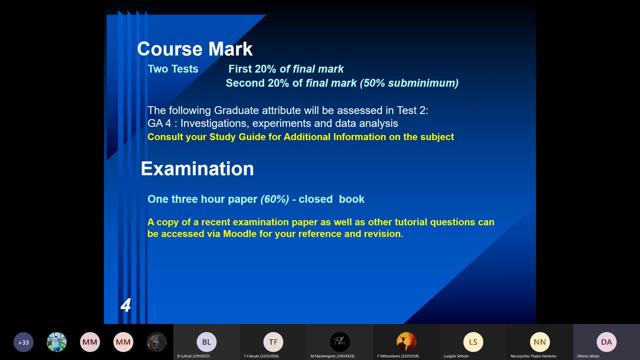 so, at this stage, yes, we are looking at an exam but, like i said, it could change depending on the academic situation. it could change to ca continuous assessment and it could even change to an online assessment. for now, yes, your test and your examination is online. sorry, face to face on campus. 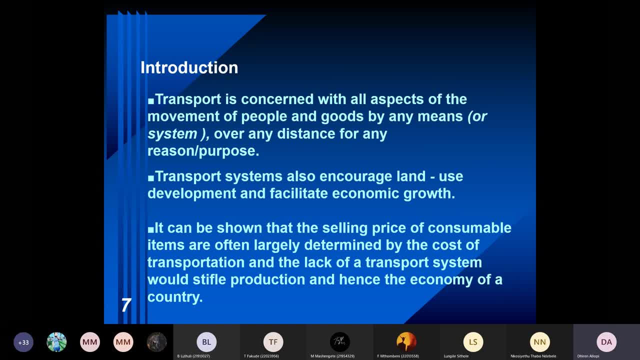 so we then look at the first chapter, then transportation planning. so what is transportation planning? so you can see very self-explanatory- concerned with all aspects of movement. we're looking at movement of not only people, but goods as well. your freight also falls under transportation planning. 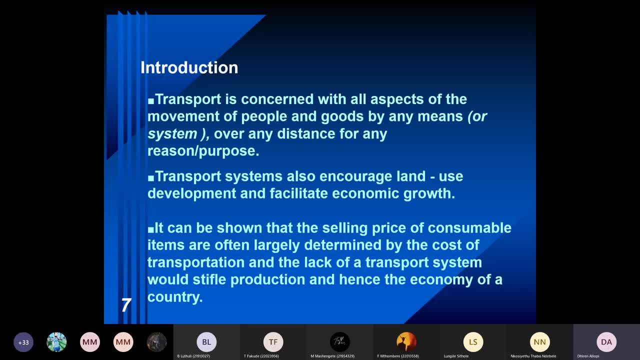 by any means. when we talk in terms of any means, what system so? whether it's by road, is it by rail, by water, by air? so that's your transportation system over any distance distance: yes, you could expect shorter distance maybe with road transport compared to, say, air transport, longer distance. 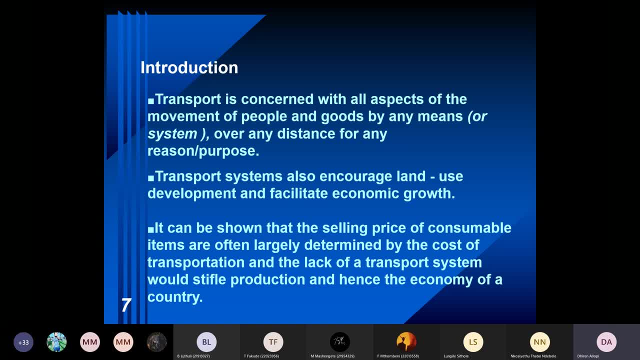 and it has to be for some purpose, some trip purpose, some reason. so if you were going to campus then your trip purpose will be education, transportation. so basically, if you were going to a casino, then obviously it's recreational gambling enjoyment. so those, so you can see, your trip purpose can change: going to walk, so trip. 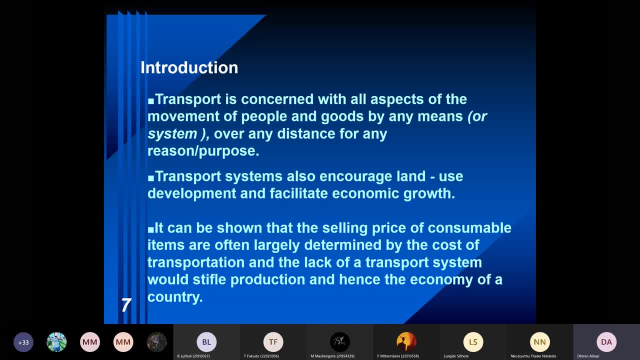 purpose could be walk. so that's in a nutshell, and you will find that there is a direct link between your transport systems and land use. when we talk in terms of land use, understanding transportation is also things in terms of transportation. well, Ergebnis depends on transportation, land use as me. 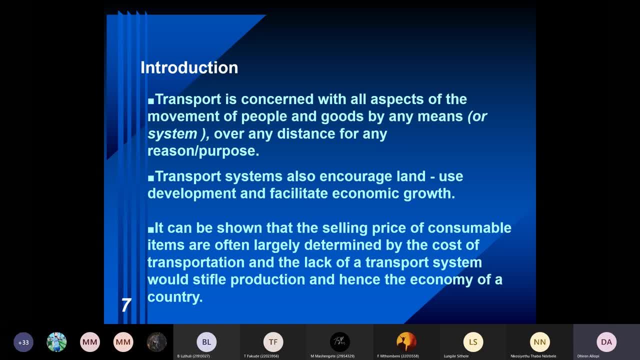 and if i could relate you to typical examples, consider the gateway complex. can you imagine the gateway, gateway complex standing there with no proper transportation network to link you to the complex? so you can see the direct link and how it has an impact on the value, the economic growth. 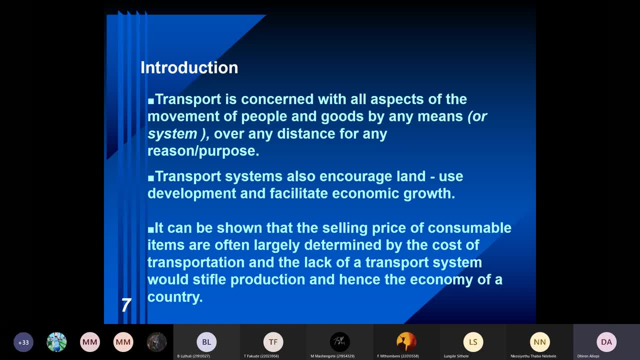 look at all the buildings that have come about around the gateway complex, the flats that have developed around the gateway complex, and the value, the cost- single bedroom flat in that vicinity cost you more than a million. so you can see the direct link there between the transport system and 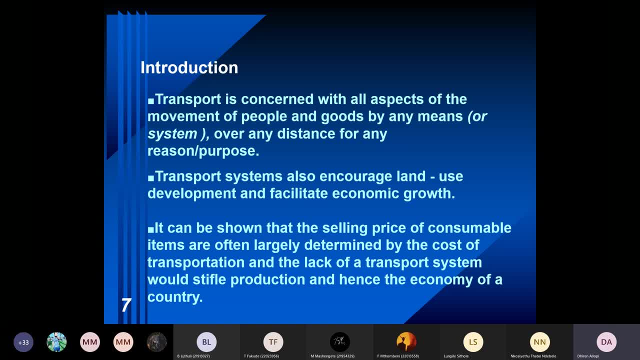 your land use. and if you look at the last bullet there, you can also see how the cost of transportation impacts. so you know, the moment there's an increase in the price of fuel, the price of bread, the price of milk or other food items goes up directly. 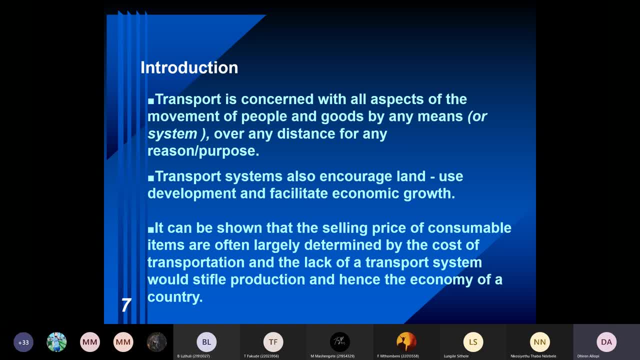 linked to transport. now can you imagine you were a farmer in billyburg and you needed to sell your product. you were planting cabbages in billyburg and you needed to sell the cabbages in the marketplace which is in timbuktu. and if you didn't have the transport to transport your 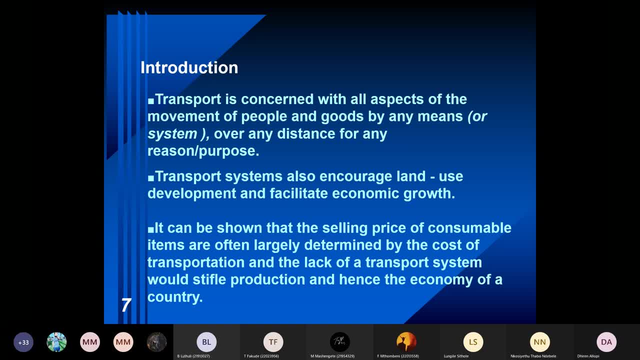 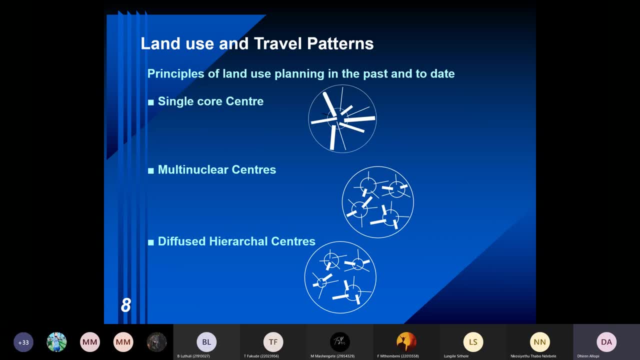 products to the marketplace. what a waste. so you can see the direct link, a lot of the information here, the theory information, i must say, is not far-fetched. if you read through it it makes sense. and the other point i want to mention, a very important point, is that the intention is not 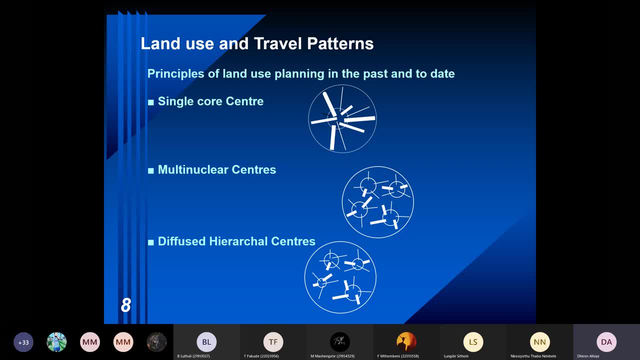 for me to read through your notes, page by page, and put all of you off to sleep. the main purpose of these lectures is to give you an overview of what's in your notes, to highlight the key points, the keywords, and also to bring in industry relevance. that's the main, primary objective of these lectures. but the onus is then on you. 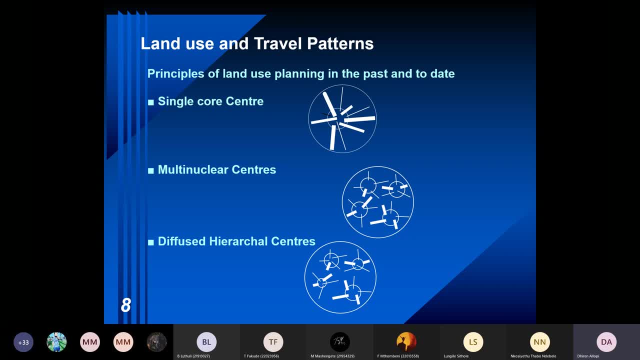 to go back and look at the notes that's posted on moodle. go through the notes, read through the notes, but do not forget to subscribe to the channel to follow the next videos and also remember by attending the lectures. you can see from the presentation what is important. 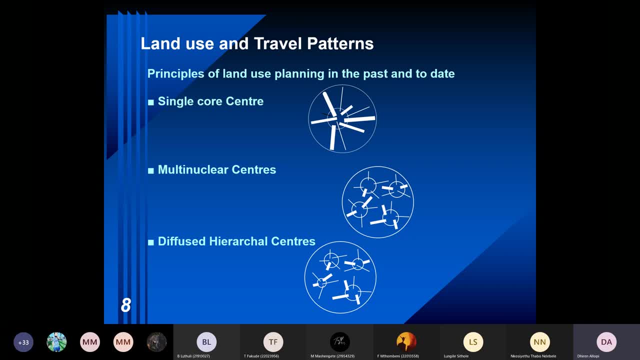 and you can then go back to your notes and relate to this information in your notes. okay, sorry sir. yes, sorry. so just to clarify, the powerpoint is just a summary of the notes and the notes are just are more in depth. uh, look into the topics. okay, yes, you will find that the note sometimes 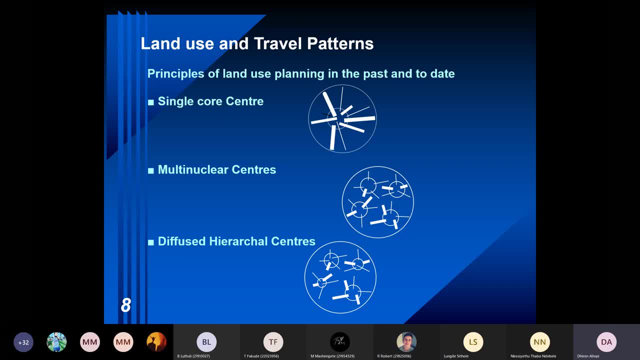 the notes also have some additional information and that's not to waste a lot of. some of the additional information will certainly come in handy when you do register for the advanced program, the honors program. so that is why, again, i'm coming back to the lectures. when you go through the lectures and you identify what i am presenting at the lectures, 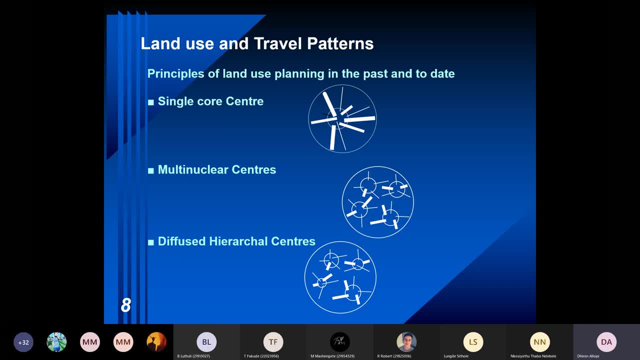 and then find that in your notes and relate that to your notes. you will then be able to pick up what is important for the test and the exam with regard to the theory. so again, another important point why you should be attending the lectures. so coming back then you will find that in your notes you do. 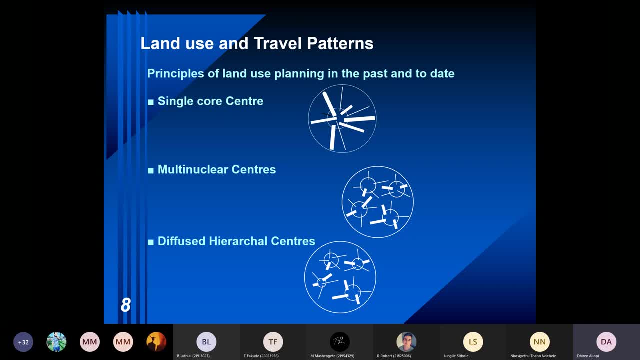 have some information on land use and travel patterns and you can see from these few simple sketches or diagrams how your planning has changed over the years. i've had to go back many, many years and if i took any city, whether it's durban, pmb, escort, newcastle- you will find that all these 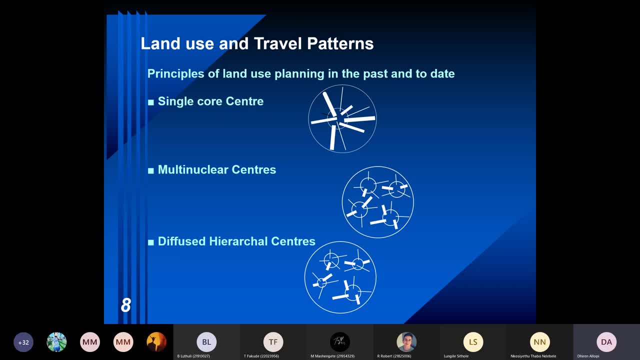 cities had a single core system, that's your cbd and all your roads linking to your cbd from the various residential areas. so the cbd was a hub. that's where the employment took place, that's where you did your shopping. okay, but compared to current cities like newcastle or newcastle or newcastle- 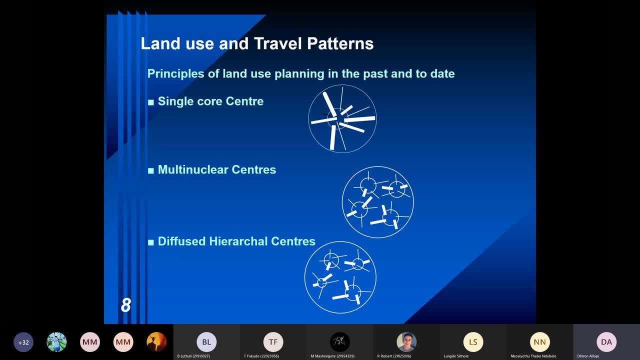 it's a different situation now. you have so many different centers, whether it's a gateway complex, the pavilion complex, the brit city complex or the ushaka, whatever you will find. now you've moved away from the single core center system to a more multi nuclear system. 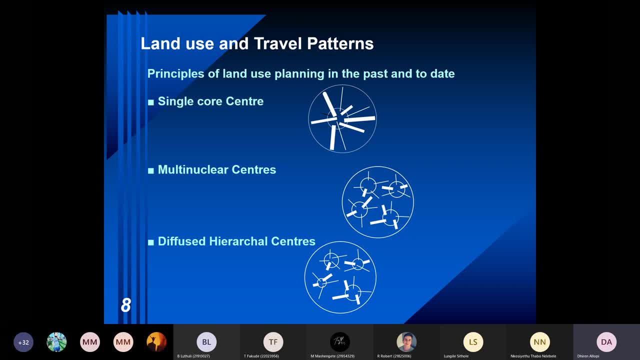 the basic difference between those two is that here you can see that your circumference are the same, so we're looking at equal attraction, whereas here you can see the circumferences are different, so we're looking at unequal attraction with the diffuse centers. okay, so one could be maybe the suncoast complex, the other one could be the gateway complex. 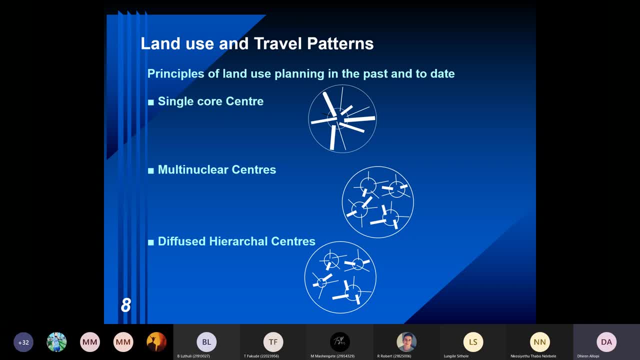 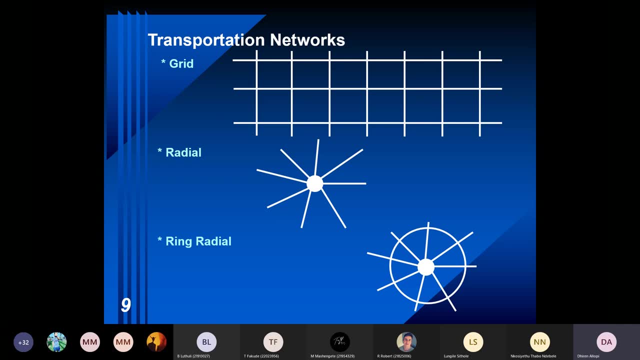 you can distinguish so you can see how the situation has changed. the same applies to your transportation networks again. if you look at the cbd, you can see that the cbd has changed. the same applies to your transportation networks again. if you go back many, many years and still up to date, many of the cities have this grid system. 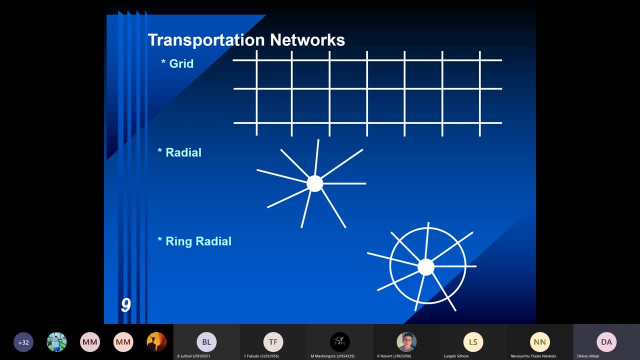 if you had to take an aerial photo of, say, um s quad, you will see the typical grid system: your streets running parallel, cutting across. but over the years, yes, there have been some improvements, some changes where you could, moving from a radial to a ring radio. so here in in durban, 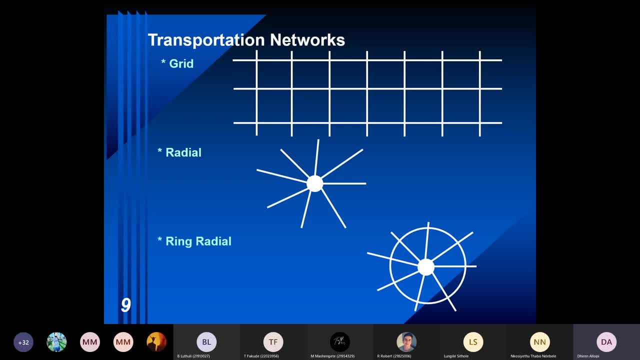 In Durban. now we have the ring road, the N2 ring road. In the past, if you had to get from Durban to Pietermaritzburg, you had to pass through the city centre, get into Smith Street and whatever. or if you were in Pietermaritzburg, 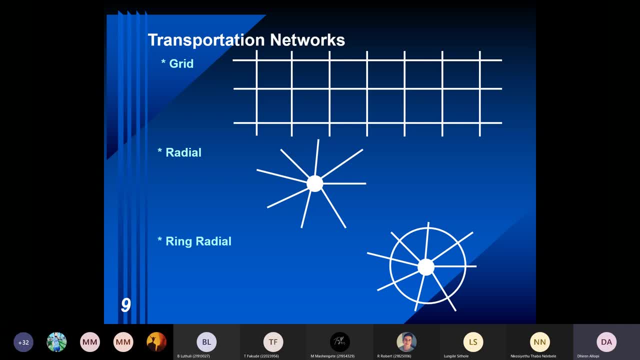 you had to get into Longmarket Street or Church Street to get through to the next town if you wanted to get through to, say, Escort. But that has now changed. We have ring roads that allow you to bypass the CBD. So now if you are perhaps going to PMB, you don't have to go into the CBD of PMB. 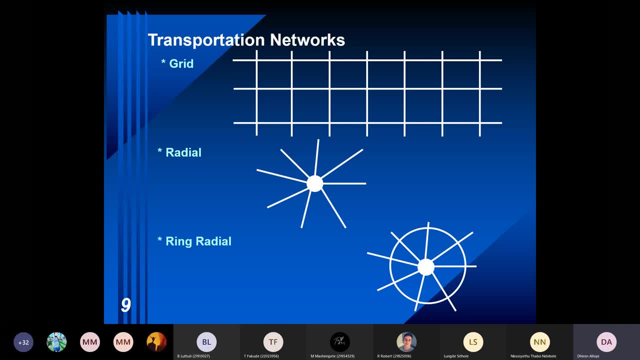 You have the N3 or the N2 or the N1, I'm not referring specifically now to a particular area, Whether it's Kauteng, Whether it's Kauteng, Whether it's KZN, So you can see from there how your transportation networks have changed. 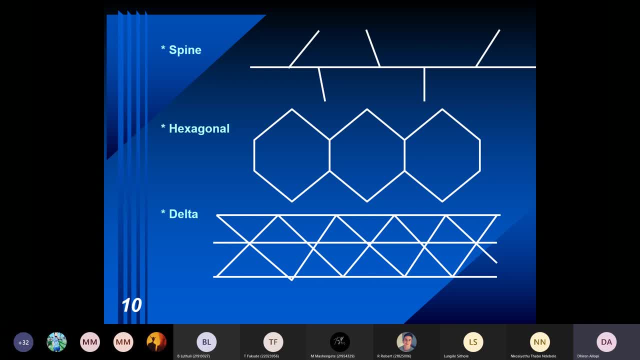 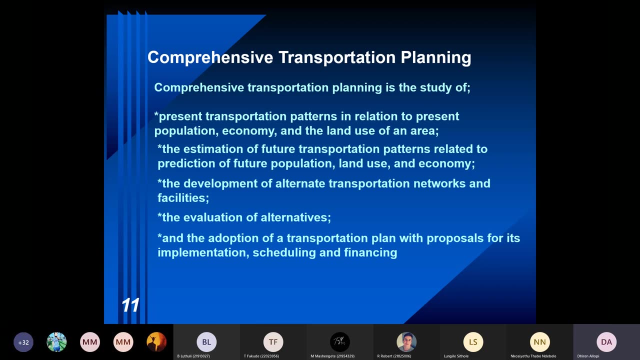 And these are just different forms of transportation network where you have the hexagonal hexagonal spine and delta and so forth. So you can look at your notes. There are diagrams of these in your notes. So, coming on and moving on to comprehensive transportation planning, 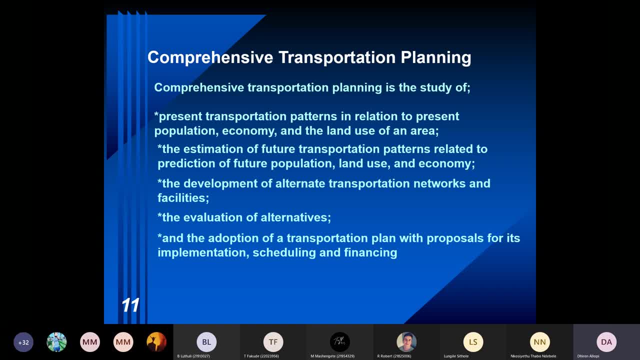 What do we mean by comprehensive transportation planning? So that is simply. It's simply a study. study firstly of keyword, of course, being the present, present situation, Estimating the future From the future, looking at the various alternatives, evaluating the alternatives and then based 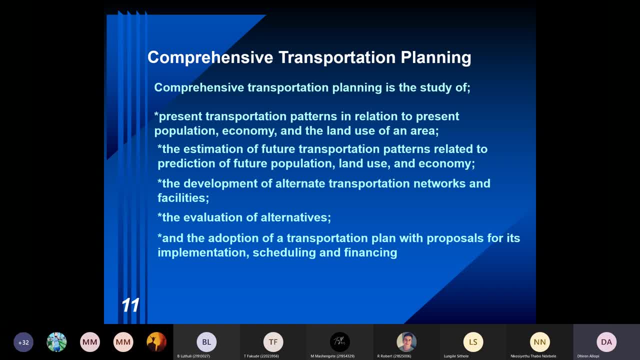 on the alternatives doing your final implementation. Okay, so those are. you can see the keywords. So- and this could Relate to any situation- So, in the past, when transport technology Had a, A geometric design project attached to it, Then students were given a plan of an area and they were then required to choose the. 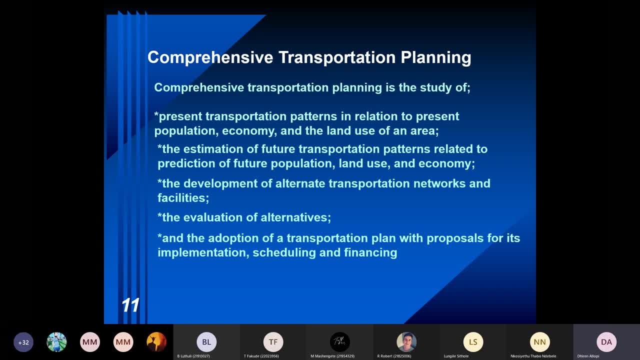 best alternative from point A to point B. So the group then had to look at A and B, Look at the contours, Look at The river crossing, Look at other physical features like pipelines, roads etc. And check, Maybe come up with three, four, five different alternatives. 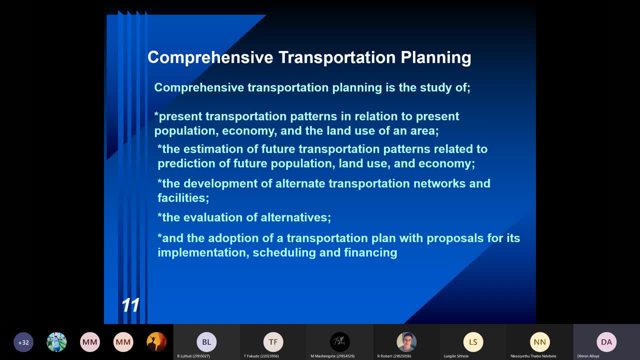 And weigh each alternative. Maybe alternative one. Maybe A river crossing, So there's an added cost in terms of building a bridge. River two. Alternative two could be through a marshy area, So there's a problem With drainage, Provision of culverts. 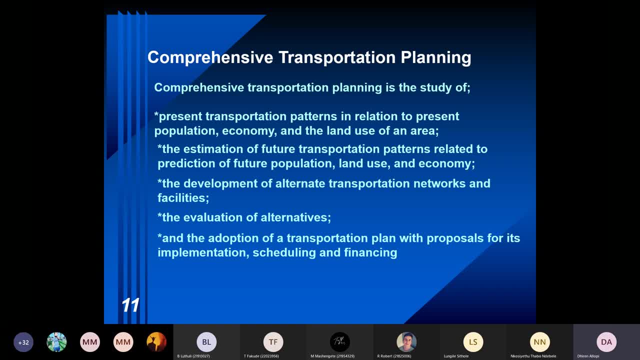 So one could then go through each alternative And some they decide which is the best alternative is very often the best alternative relates or linked to the money basket economic factor, But not- but being my not- always the lowest cost is the best alternative, So that's something you might also take into account. 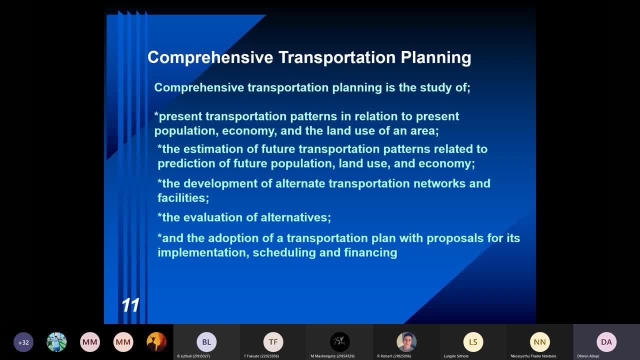 So you can see from the The various Steps Where you are. firstly looking at the present situation and If I could also relate to a practical situation, good, few years back the Tiquini municipality ran a project On demographics, on the car ownership population, so it was a forecasting project and I had 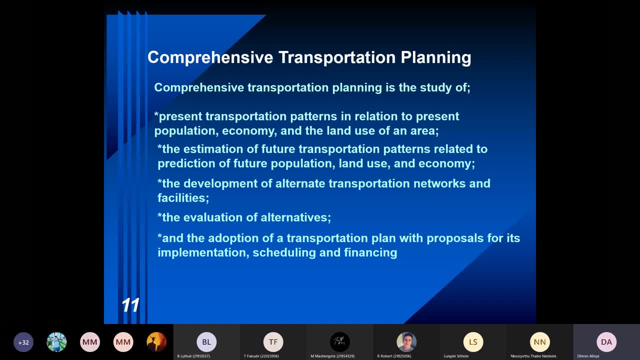 the privilege To have completed it, To be the head of that project for Tiquini municipality, and we had to then look at Which sectors are areas in the Tiquini municipality are expanding, progressing. so they took. any municipality will split into the southern region, the central region, the outer west. 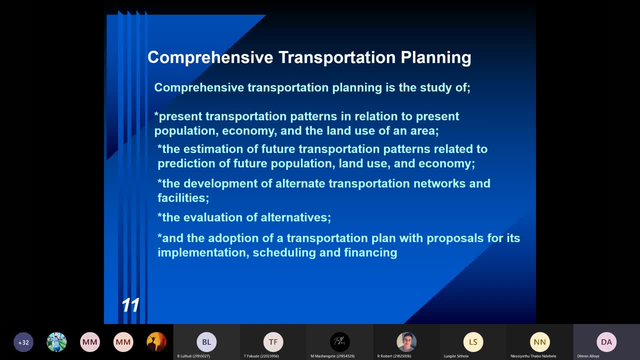 region and the northern region, And from your observation you can also see which Region Is expanding More, A lot most. Take the central. it's virtually exhausted. not much Outer West due to the undulating terrain, steep terrain, not much going on in the outer West And you can see a lot of 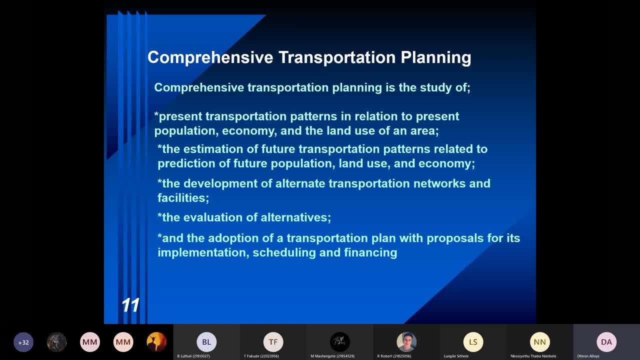 the developments taking place in the north Canoe: beer, housing projects, your new airport that came up there, trade port. So you can see a lot of the developments are taking up in the north zone. So one could then split the Chikwini area and then look at the employment. 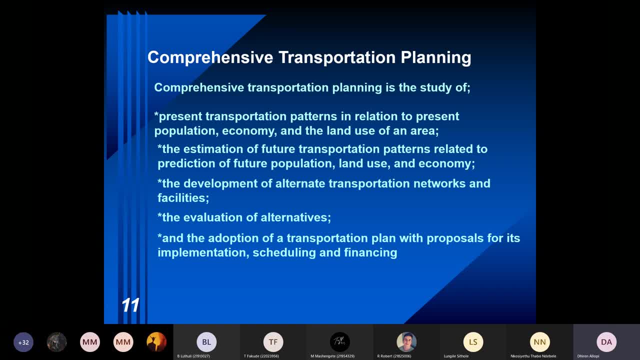 rate, the population, the car ownership rate and so forth in the various zones. So the same applies here. where you're looking at the present situation, you're estimating future transport patterns, basing it again on your population, land use and so forth, And then 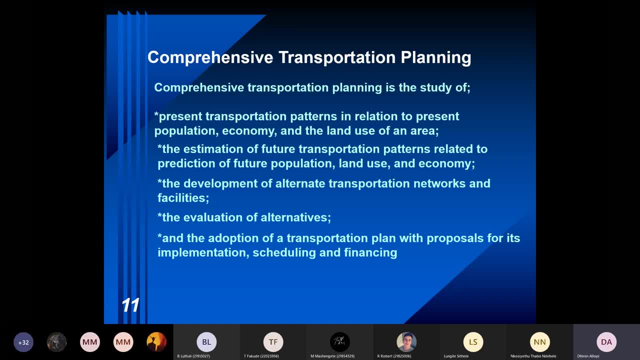 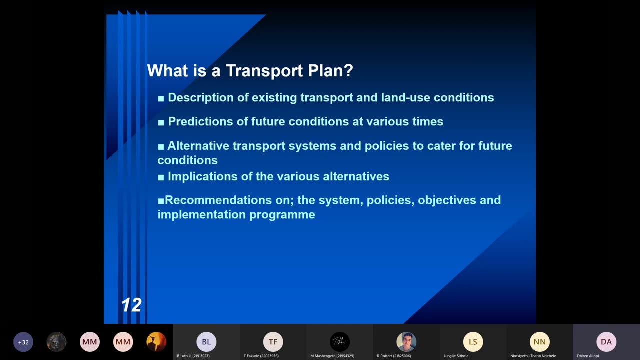 you look at the different alternatives And evaluate the alternatives and from there come up with proposals for implementation, for financing, for scheduling and so forth. So, in summary, what is a transport plan? A transport plan? firstly, you're looking at the description of the existing conditions. 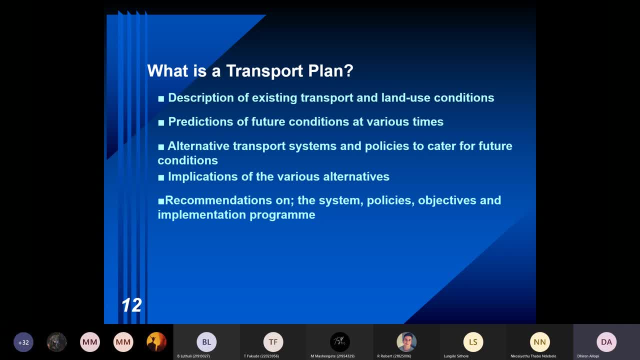 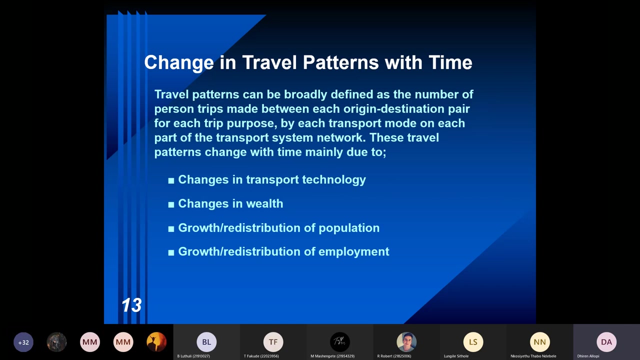 existing transport conditions, existing land use conditions, predicting future conditions, looking at the alternative systems, Implications of the various alternatives And, finally, from there, basing your recommendation on the best alternative and implementing the program. Change in travel patterns over time. Now we're talking in terms of travel patterns. what 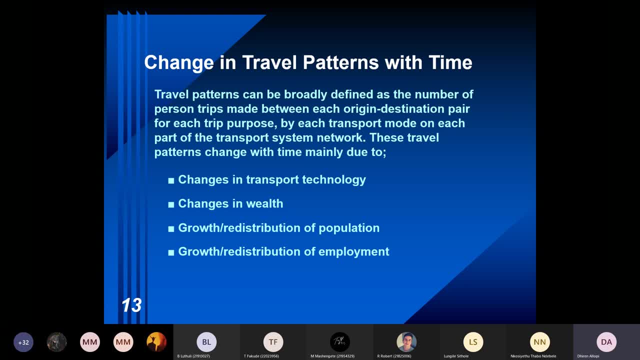 do we mean by travel patterns? And you can see a broad definition here of travel patterns. So travel patterns is defined as the number of person trips that's made between each OD. These are the 2 A's, So the number of people that make the long distance trip that are bought at a specific 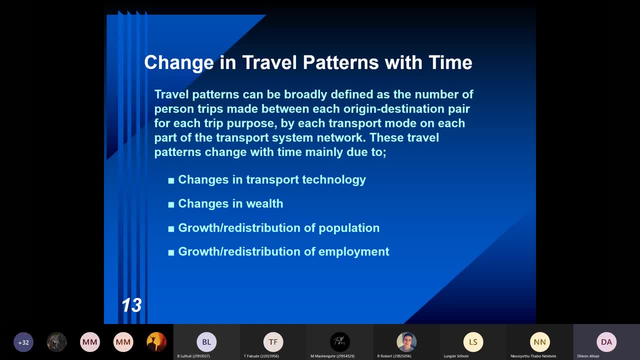 location. and then the 3 A's is what the number of people that are bought on the island, in the island, is. So that's the 3 A's. So travel is your destination, you're calling it your destination And, for example, you're calling it your home, your destination or your city. So travel. 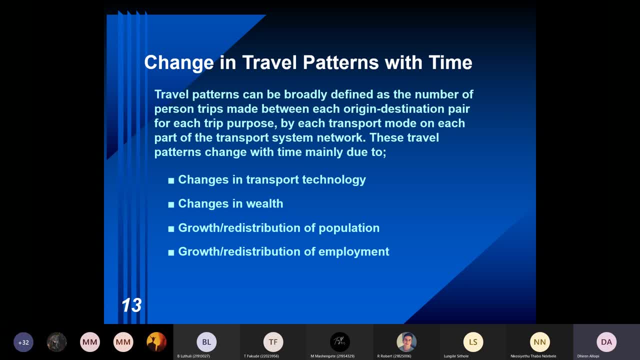 going from home to campus. your trip purpose is education. you're going to work. your trip purpose is education by each transport mode. so, by each transport mode, was it by motor car, was it by bus, mini bus, taxi, rail? okay, so you can see, and these travel patterns then change, mainly due to. 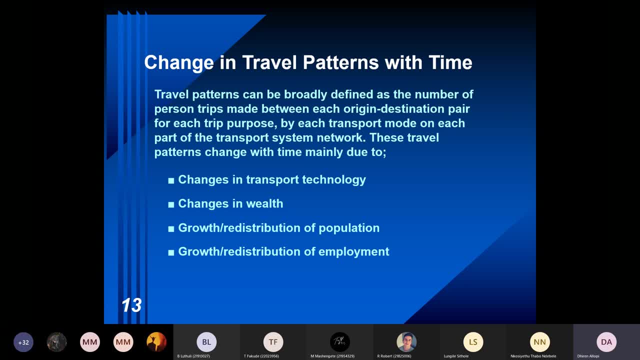 certain factors. so if you had, for example, changes in transport technology, so looking at transport technology, the changes, and if one had to go into the history of transport, you will see how it has evolved over the years. now, if i had to go back, maybe you can answer this for me. 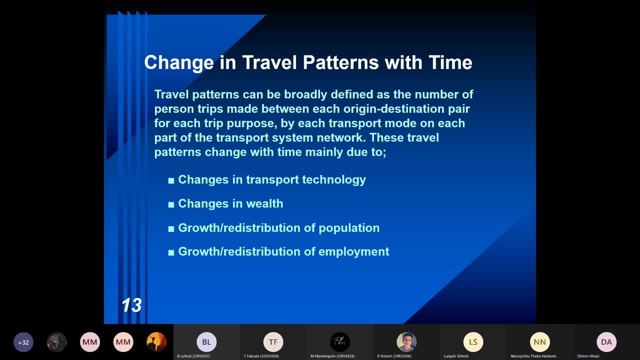 what was the first form of transport? anyone? first form of transport: walking. sorry, robert, walking sir. yes, certainly walking. so you can see from walking we moved on to animal drawn vehicles: horse and cart or on horseback down the river on a log. so compare that to now with the motor car, the invention aircraft. 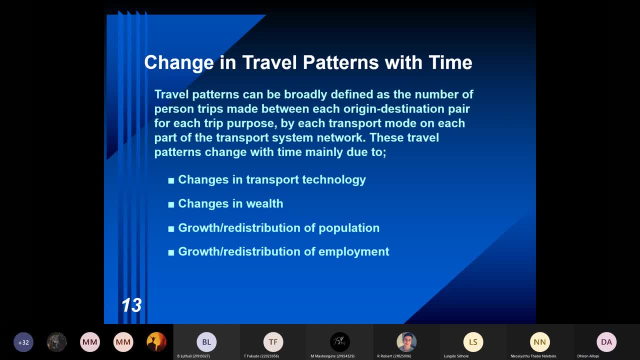 ships, hovercraft, various forms of transport. so would the changes in transport technology. certainly, travel patterns have changed as well. today, so many people are catching a flight to work morning and afternoon. wasn't there many, many moons years ago? changes in wealth: the moment you have a few extra bucks in your pocket, you want to buy a motor car, isn't it? 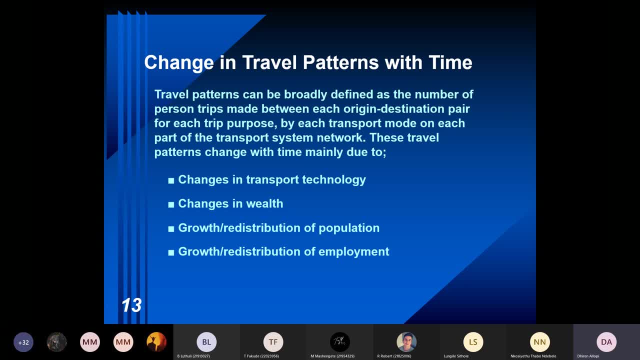 and add to the traffic congestion on the road. okay, so we'll talk a little bit more about traffic congestion and, yes, i think some information on traffic condition. you did do in 2a as well- factors affecting capacity. you must have done that. prevailing traffic conditions rings about. 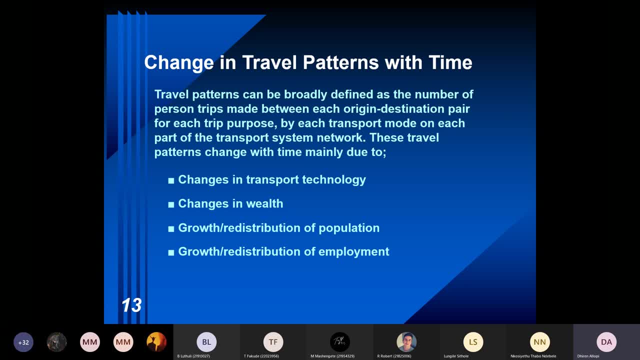 how your traffic varies from hour to hour. on the road, a peak traffic in the morning, all your peak traffic. many years ago your peak traffic was perhaps half an hour, from maybe 7- 15 to 7- 45. today your peak traffic is expanded to maybe two hours, from maybe 6- 15 in the morning to 8- 15.. 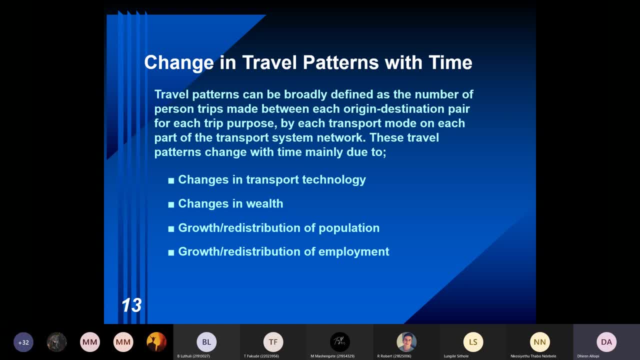 so you can see in the same applies to your pmp peak, the afternoon peak And then other factors that has an impact on your travel patterns, like growth, redistribution of population, redistribution of employment. here's the moment there's an increase in population. 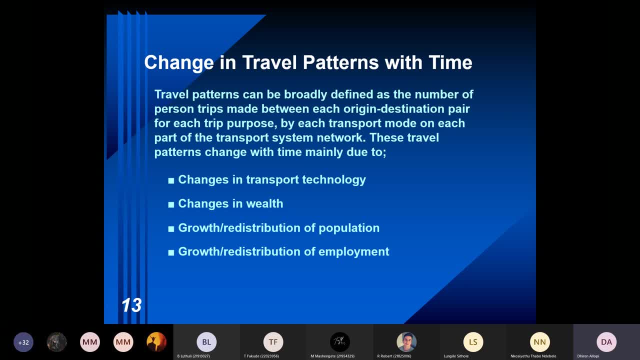 one could link that to maybe an increase in car ownership, which will certainly then have an impact on your travel patterns. If you're looking at employment, take, for example, the Nandi Industrial or the River Horse Valley Industrial Complex. you all know where Nandi Drive is- new industrial hub that. 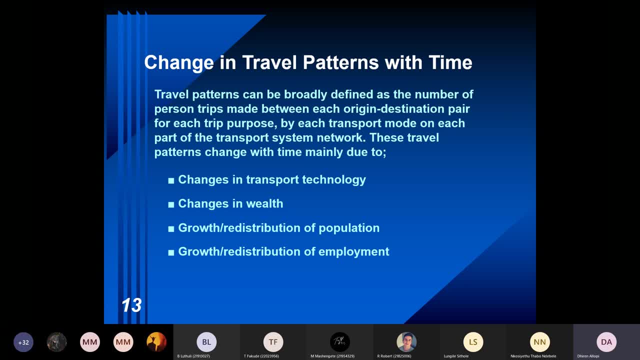 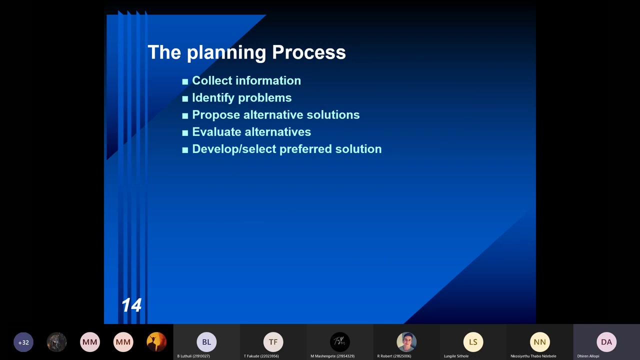 has come about. So certainly a redistribution of employment to that area from other areas, which certainly then impacts on your travel pattern, change in travel pattern. So one could relate this to reality, to typical situations. So then, the planning process, then, is simply collection of information, identifying problems. 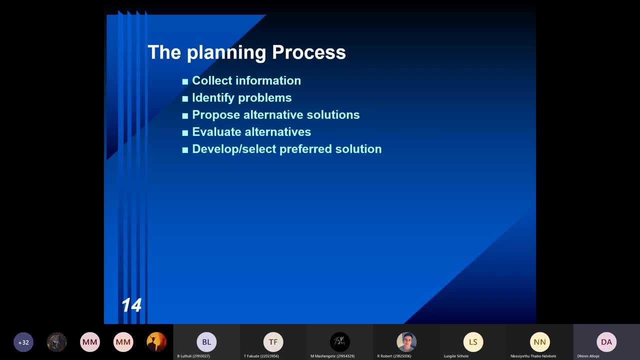 looking at alternative solutions, evaluating the alternatives and then selecting the preferred solution. Like I said very often, is the money basket that dictates, but not always. One has to look at all the factors, And this again could apply to any situation. 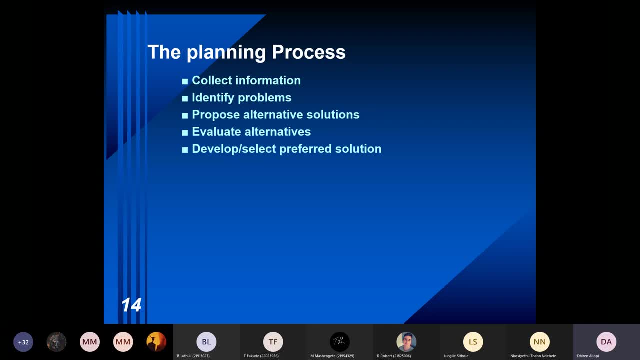 I could give you a project and tell you the Warwick Avenue Triangle. you all know where the Warwick Avenue Triangle is, below campus, where the rail station is the Biriyar Rail Station, the bus and minibus taxi terminals. So I could tell you that the intersection. I could choose one of the intersections there. 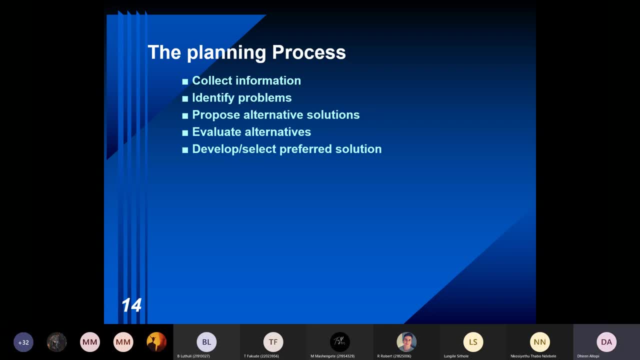 and say to you that this The backlog of vehicles wanting to turn right at the intersection, And please try and investigate why there's a queue of vehicles wanting to turn right. Obviously they can't turn right because of oncoming traffic, And that then creates a typical point for a head-on collision at that intersection. 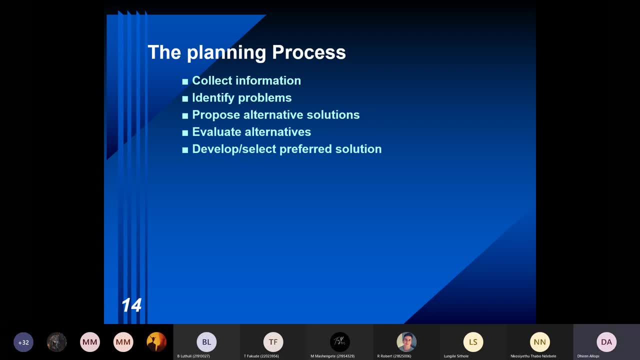 point of conflict. So you will then need to go, So you will then need to go, So you will then need to go And collect some information pertaining to that intersection. Look at the past vehicles in the different approaches right turning. Look at the signalization of that intersection. 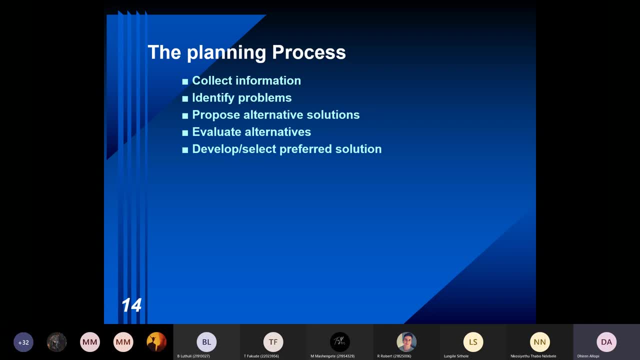 So there's various information you can collect. You can sit at that intersection and do an observation vehicle count right And then you can then check why perhaps there's so many vehicles now, increasing the number of vehicles that want to make the right turn. 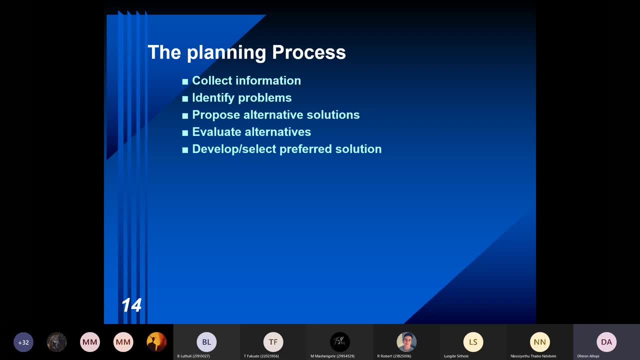 And perhaps you may have identified a new industrial area that has come about in that, So more people are now redistributed, employed in that area, which has now created a backlog traffic jam at that intersection pertaining to right turning movement. So you could then propose alternative solutions. 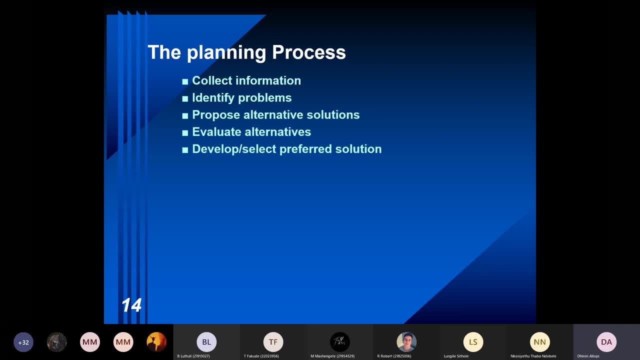 You could look at various alternatives. You could consider: Uh, the city Signalized Interchange, or intersection in this case. so look at the traffic lights, look at the amount of green time allocated. Perhaps that traffic light did not even allow for right turning, so you need to change the 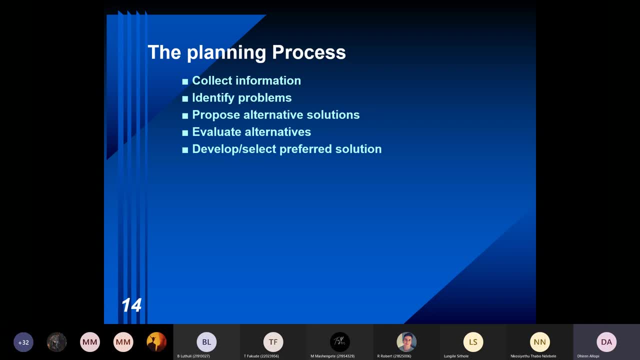 signalized setting to maybe give priority, a green arrow, priority for right turning vehicle. Allow X amount of time for vehicles to turn right. Stop the oncoming traffic. You travel on road, so you've seen these arrows right turning or whatever, so that 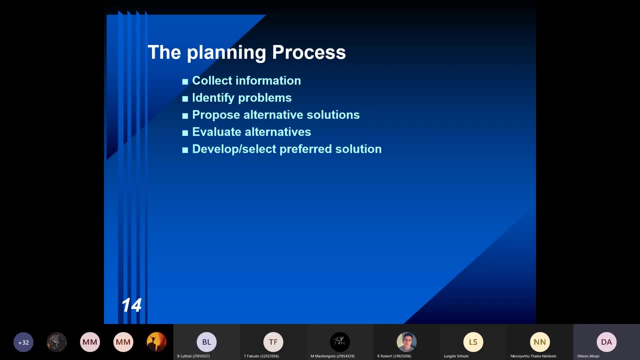 way you can then clear the backlog at that intersection. So by simply so this falls under traffic management techniques where you simply readjust the traffic signal setting at that intersection and you can solve the problem. You could have maybe considered great separation Interchange. 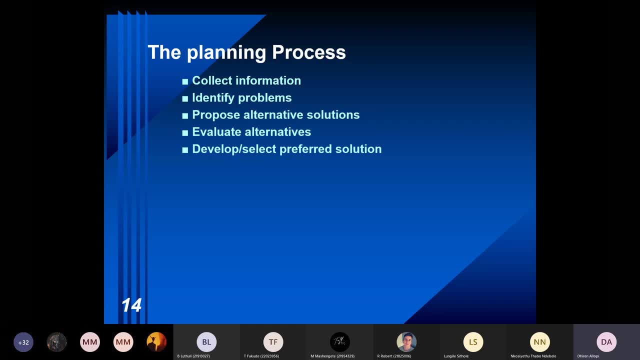 Where you then Prevent Conflict at that intersection by having great separation but then be in mind the cost of great separation To maybe simply doing a signalized resetting at that intersection. So there's various alternatives. one could think of having a dedicated right turning. 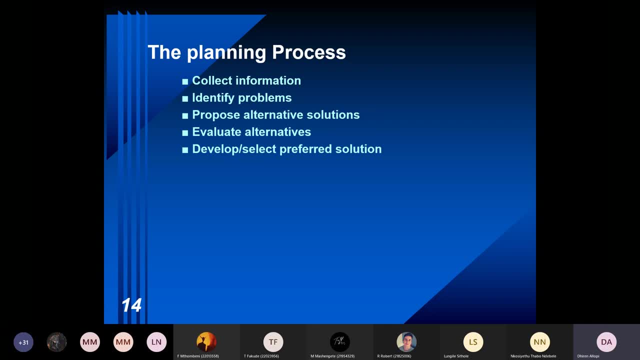 lane by means of channelization, painted arrows. so there's various alternatives one could think of, and from there you can then select which is the best alternative. I mentioned the word intersection and interchange Short while ago, And my question to you is: what is the difference between an intersection and an interchange? 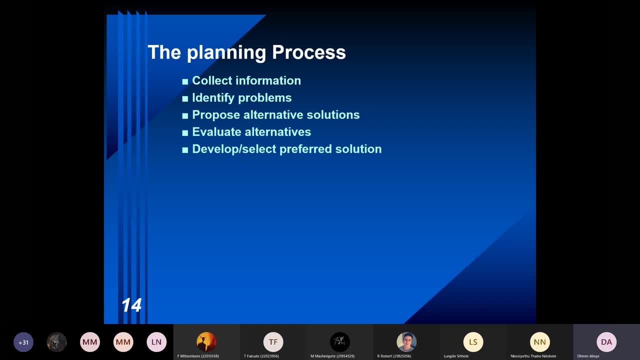 What is the difference between an intersection and interchange? Perhaps you did this in two way. Anyone Like to have a go at it? Difference between an intersection And interchange. Anyone Try Take it. Yes, Sir, Yes, Yes, go for it. 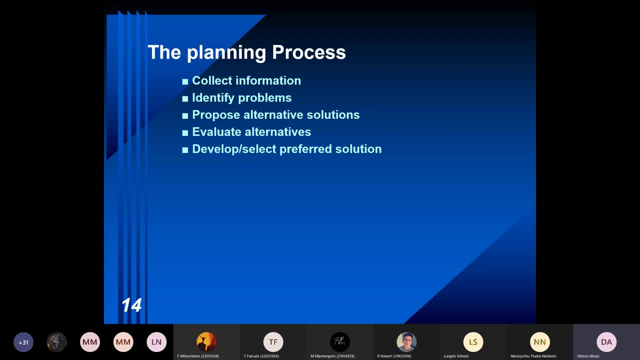 Interchange is like great separated intersection: One road passes over another. Intersection is. Interchange is when a a in the intersection, an intersection, passes over another intersection and then another, And then you change it. Interchange is, Interchange is. 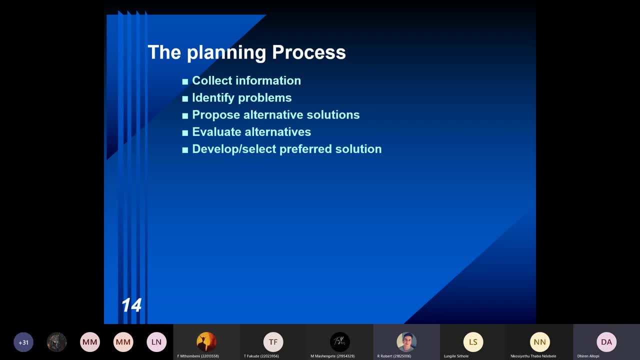 Interchange is So, in fact, it's a. it's a change is when? uh, isn't it? when one road passes over um over another, with ramps and connections? okay, an intersection. intersection is two roads connected, same level. okay, yes, you're 100, correct? 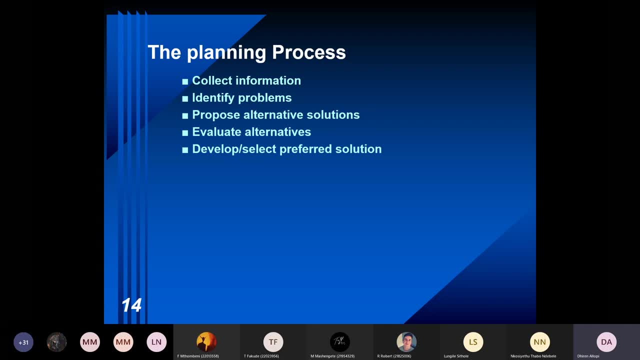 yes, an intersection is where roads cross at grade. the word is 80, 80 at grade at the same level. that's an intersection. so you got roads crossing intersecting at the same level at grade was interchanges where roads cross grade separated different levels so you can see from there when. 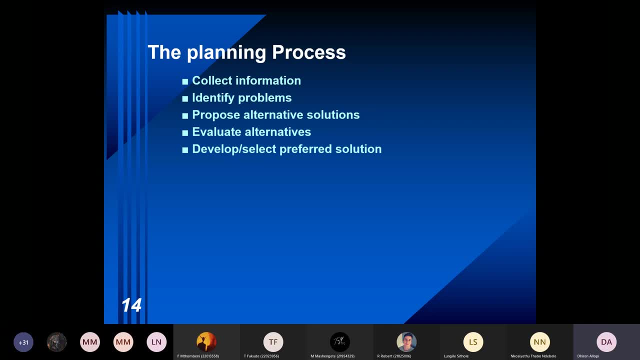 it comes to an intersection, certainly one needs to have some sort of a system to control your traffic at the intersection. they are the same level at grade, so it could be via a stop sign, a yield sign, traffic signal, okay, whereas with an interchange, because your roads are crossing at different levels, at different 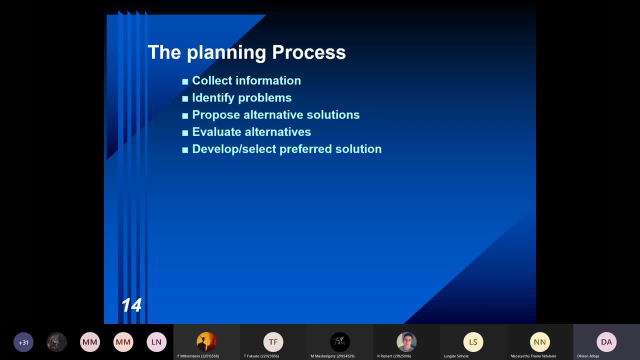 grades. you can maintain uniformity in speed. you can maintain the capacity on the road. now use the word capacity again, and i'm sure it's not a terminology that you haven't come across: capacity. so capacity is the maximum number of vehicles passing a point per hour. 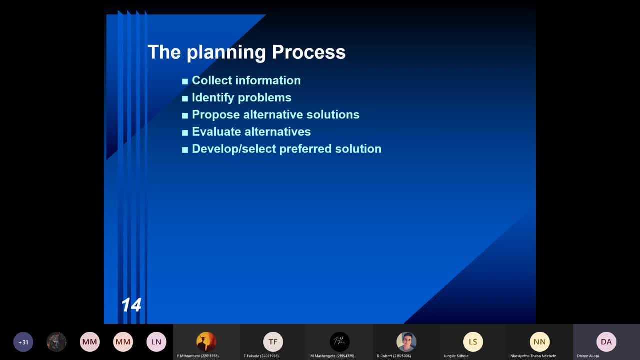 normally it's per hour for given time per hour. so any traffic engineers, uh goal is to achieve maximum capacity, maximum number of vehicles passing a point per hour. so how do you do that? and you've done. you've had to look at various factors that affect capacity, like your road with your shoulder, with potholes, geometric restrictions. 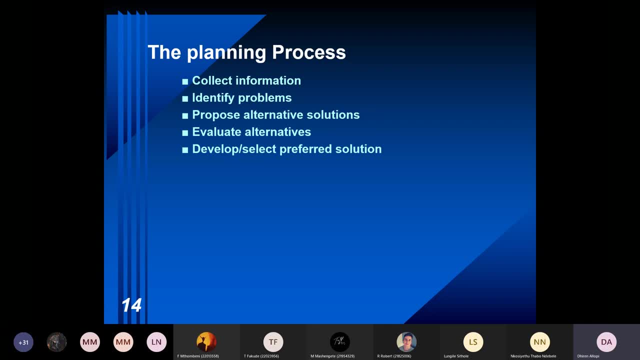 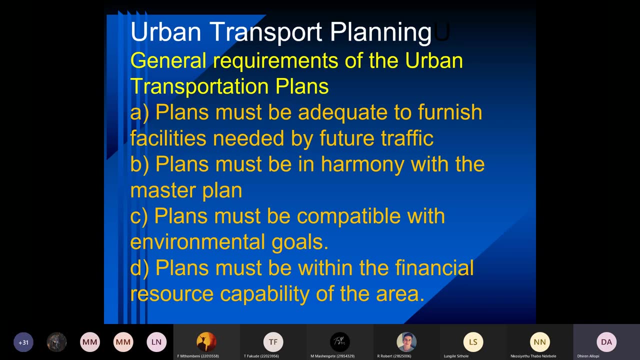 sharp curves, poor sight, distance covered, all those aspects. so it is important that one can achieve its maximum capacity. but bear in mind that this is dictated by your prevailing condition, by your prevailing road conditions, by your prevailing traffic condition. as much as, ideally, you would want to achieve high capacities. so, ideal situation: you would love to have three lanes in each. 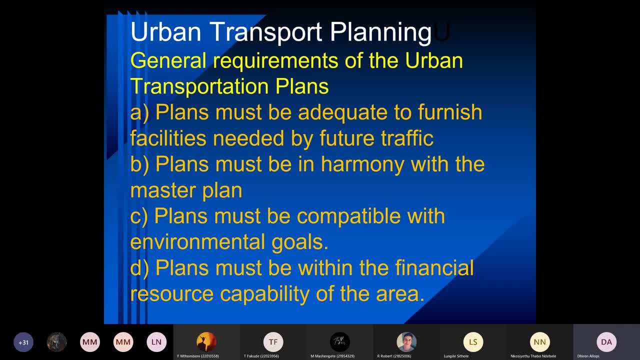 direction. low commercial vehicles, no heavies on the road- okay. good sight distance. flat curves okay. large radius of curvature, good super elevation. but it's not always possible. so one has to look at the economic factor, one has to look at the terrain and so forth. so urban transport planning, then general requirements for an urban transport. 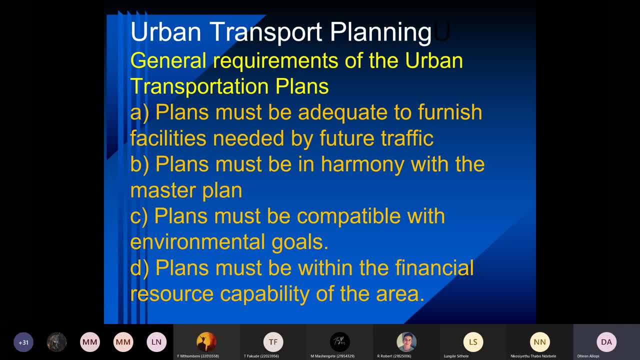 plan. you see, firstly that the plan must be adequate and you must cater for future traffic must be in sync with your blueprint, your master plan. so any plan that you come up with must be in sync with your master plan, must be compatible with environmental goals. you know, with environmental aspects is certainly a buzzword. 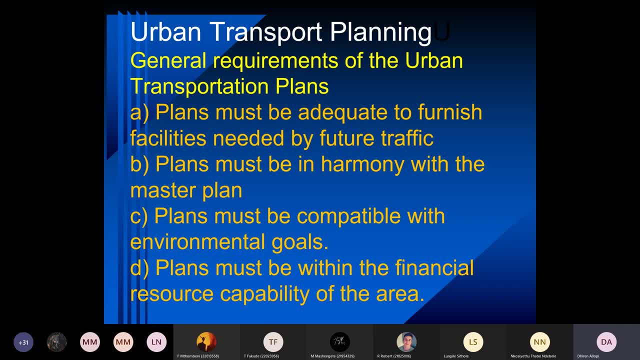 in recent time. in the past, exactly a transportation planner could quite easily design a road and mow down a hundred indigenous trees. you can't do that today. today, every proposal has to be supplemented with an environmental impact assessment, and there's many examples to this if you even look at your 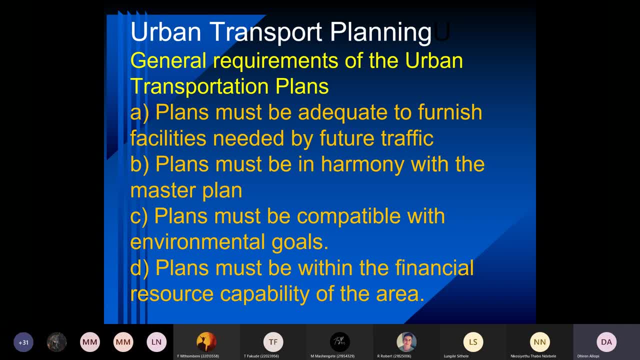 new airport, the king shaka airport. there was the issue there with the flight of bird flights that interfered with your airstrip runaway and a lot of was done to divert the flight path of your birds. if you look at um, the new brit city complex that came about and the rail 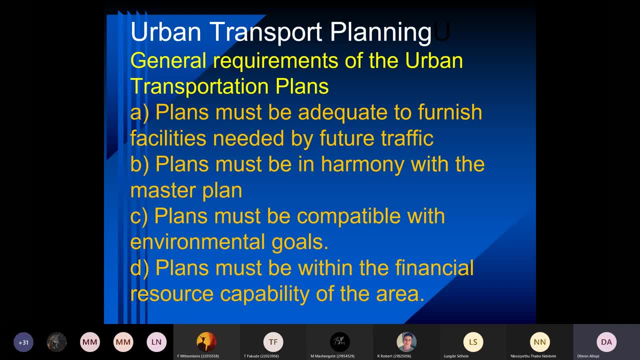 spur that linked to the new brit city complex from duff's road station, that crossed through from the port of salta uh, to the port of salta, into the port of salta, and how the transit was them사�IGH, Pointless at all coming up with the plan and you don't have the budget. 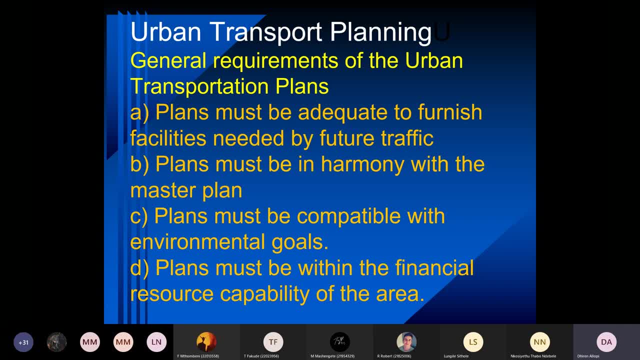 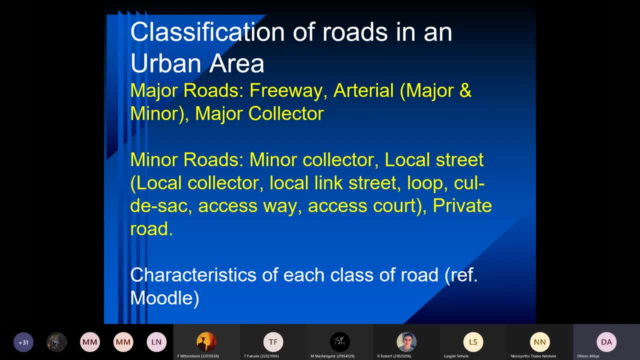 budget to meet that. So certainly the financial resource capability is another important factor to take into account. And then, finally, if you look at your notes, you will find there's some information at the end of this chapter that deals with classification of roads, And you'll see the 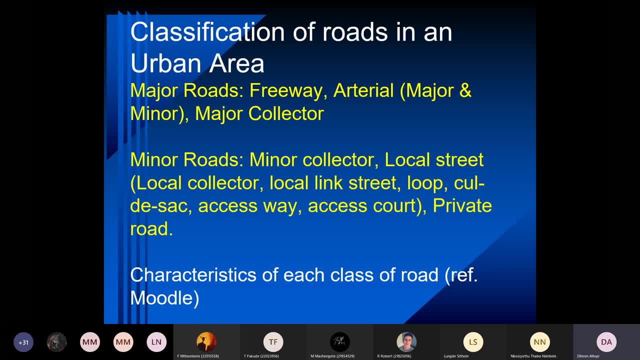 main two categories. that relates to major roads and minor roads, Your major road being your freeway, all your major collectors. your minor roads, like your local streets, your private roads, your access roads and so forth, So you can read through a point or two on each of these. 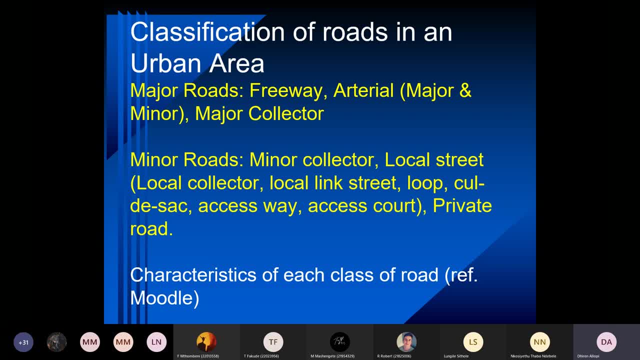 class of roads characteristics and that you could refer to Moru. So you see why I say again why it's important, then, to attend these lectures, because you should have a highlighter with you, you should have a notepad and making notes refer to Moru for characteristics of each class of roads. 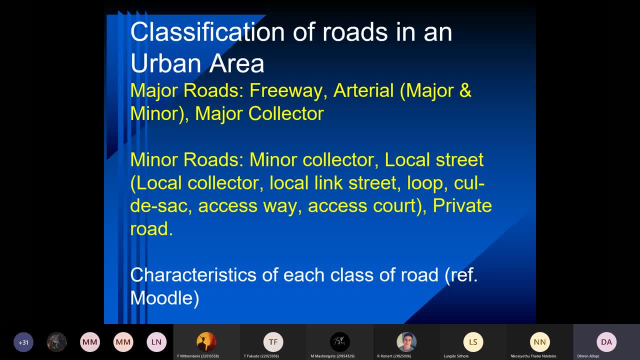 And, for that matter, all the other slides that we've been through. we should be making a quick summary of what's required of you and where you need to make reference to. Okay, so that then brings us to the end of transportation planning. So I'm going to stop this presentation and try and 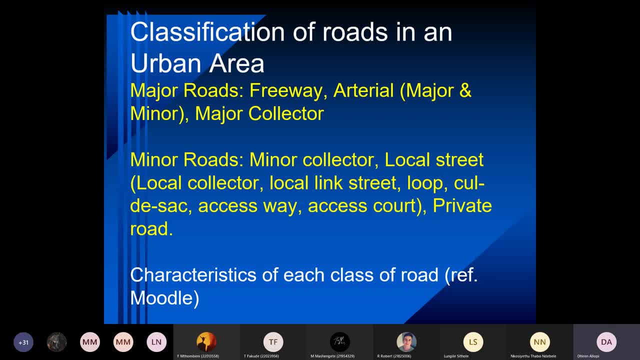 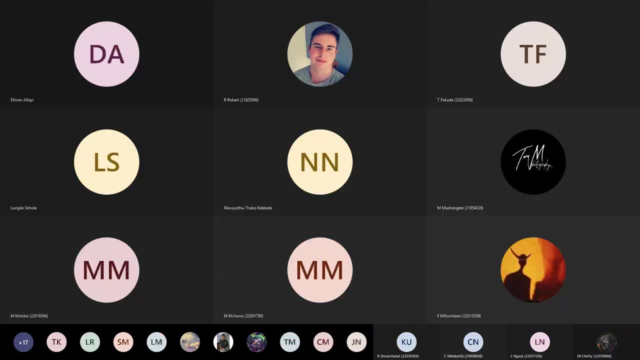 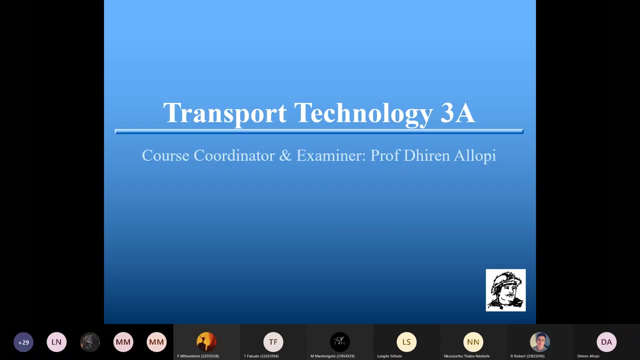 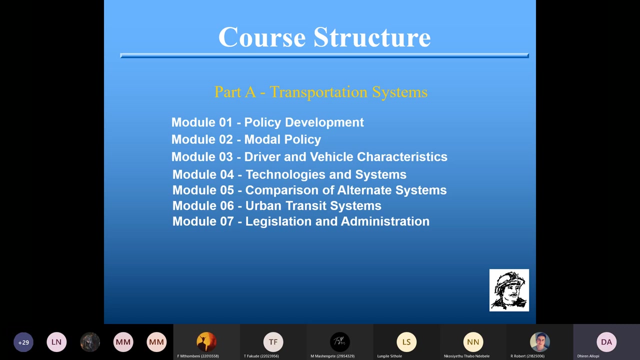 load module, one of transportation systems. Let me load it on from here. We should still be in full screen, Okay, Okay, Okay, Okay. so we're looking at transportation systems And in this subject, 3A you will be dealing with. 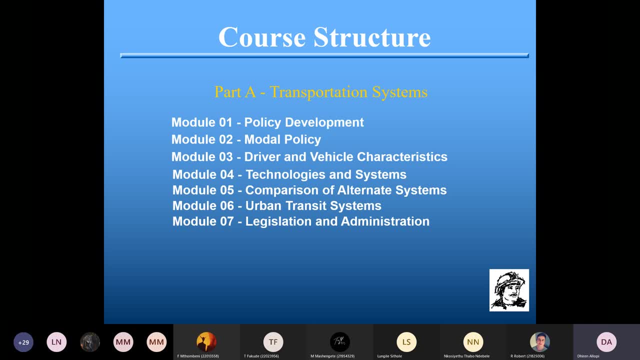 the A part of transportation system. There's a B and C part as well, which you will perhaps cover in the honors program. So, looking at transportation systems, you will see there's some information pertaining to policy, legislation and so forth, And then there's information pertaining to driver and vehicle. 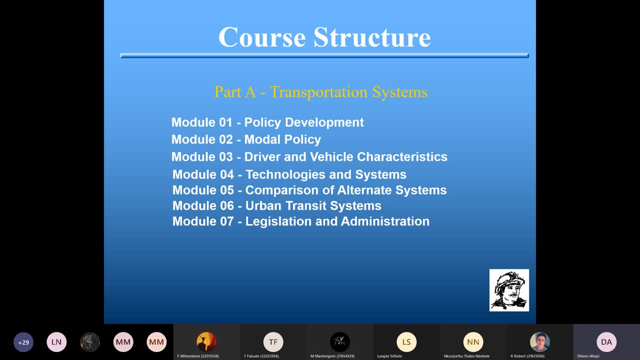 characteristics. When it comes to driver and vehicle characteristics, I could spend a whole semester only on driver and vehicle characteristics with you. All the physiological elements, the psychological elements comes to visual, visual equity, vehicle characteristics. and then there's some information pertaining to the driving and vehicle characteristics. When it comes to the driving, 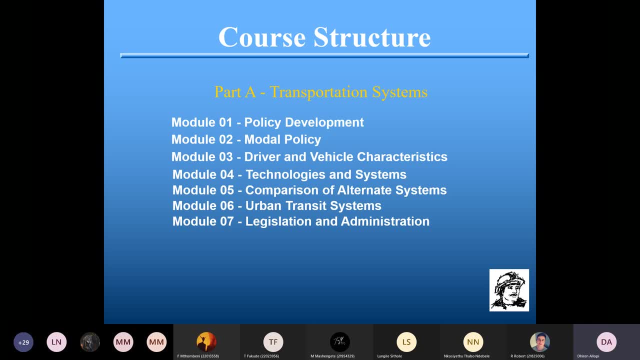 characteristics in terms of design, in terms of seating and so forth, and the calculations that go with it may be relating to side distances: stopping side distance, passing side distance, shoulder side distance, skid resistance, drag coefficient. so i could, like i said, spend a whole semester simply on driver. 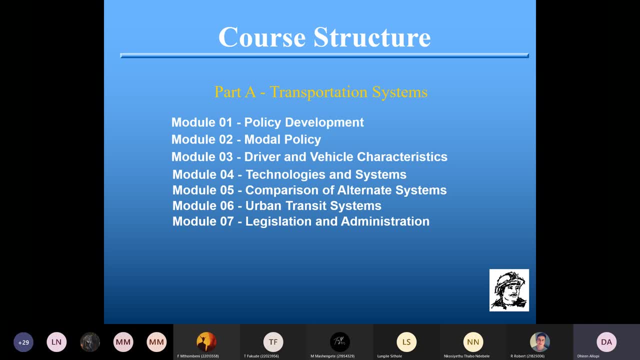 and vehicle characteristics. but that's certainly not the intention of this course. it's more an appreciation of the various aspects, with driver and vehicle characteristics being one of them, and then looking at the different transportation systems, the technologies, comparing alternative systems, like, especially when it comes to your transit systems, transit systems. 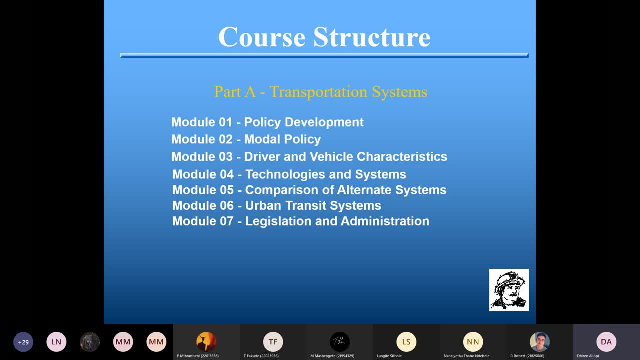 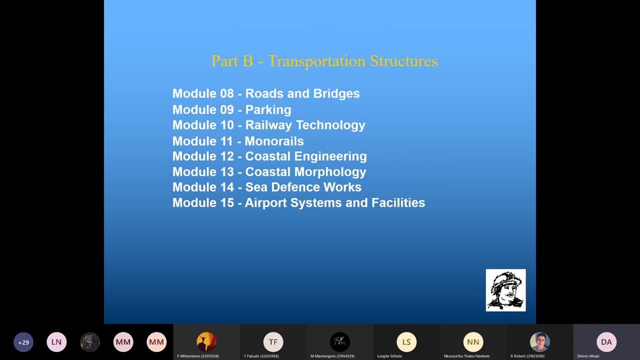 is more universal terminology for public transport, so comparing maybe, a light rail to a monorail, a minibus taxi to a bus, and so forth, so comparing different systems. so those are some of the aspects or areas that we will be covering on the transportation system. so 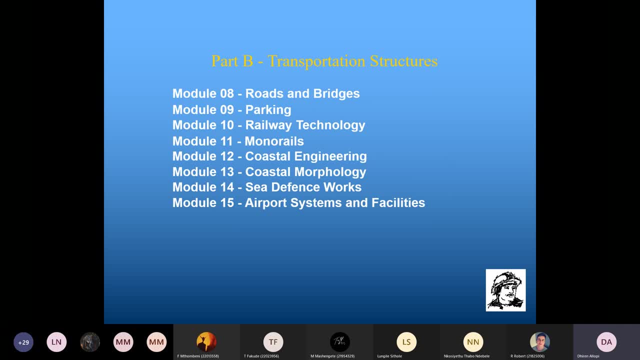 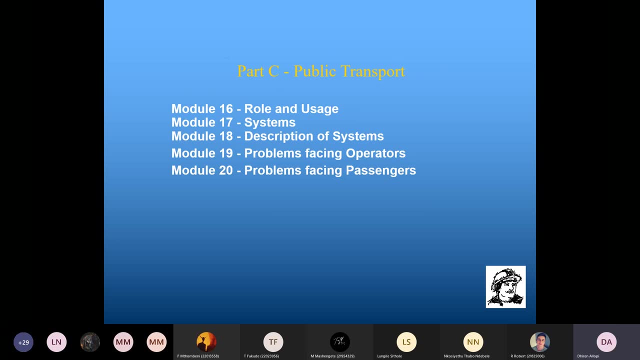 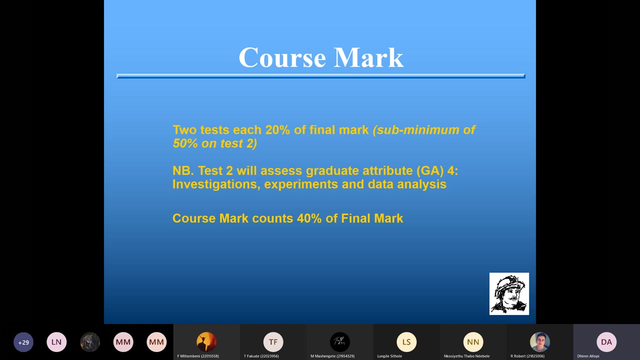 yeah, like i said, you can see from there that the b and c part that deals with structures and public transport, that, like i said, is information that will be covered in your honors program. so just to recap, then we went through the slide. previously, your course mark made up of two tests. test two, don't forget. 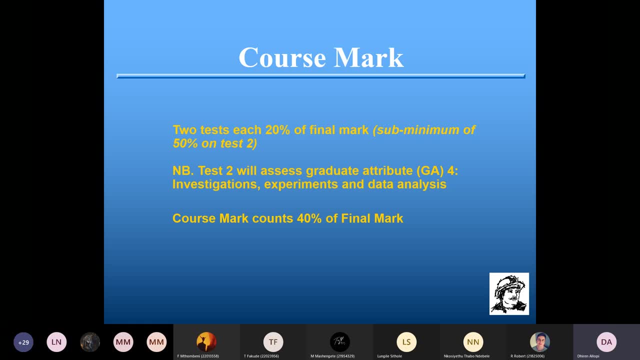 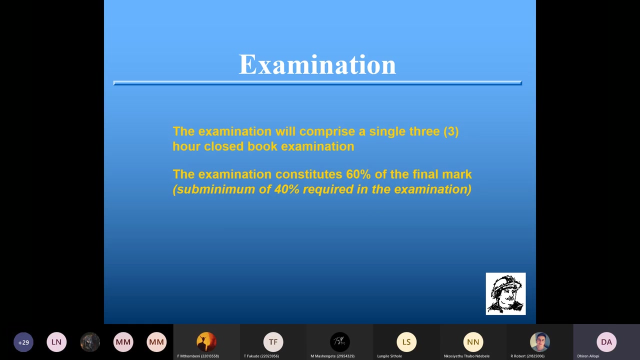 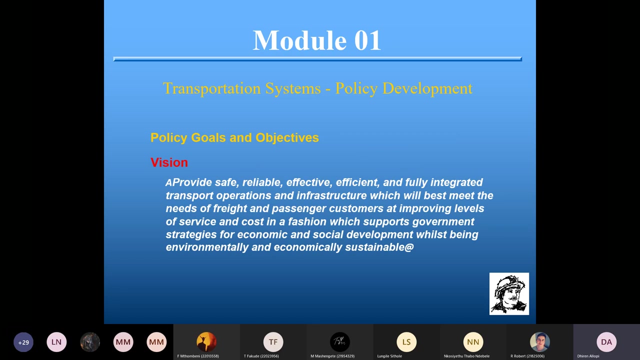 assesses your graduate attribute ga4, and sub minimum of 50 applies for test. two course mark makes up 40 percent of your final mark and the examination makes up 60 percent of your final mark. so now, when it comes to the policy aspects, the information was extracted from what we 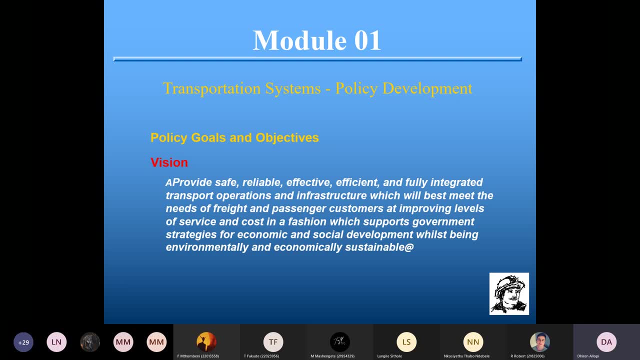 call the white paper on national transport policy. now this white paper. when the new government had taken over after 94, the um department of transport then invited invited various stakeholders from industry, from academic institutions and so forth to give their input towards the development of this White Paper on National Transport Policy. 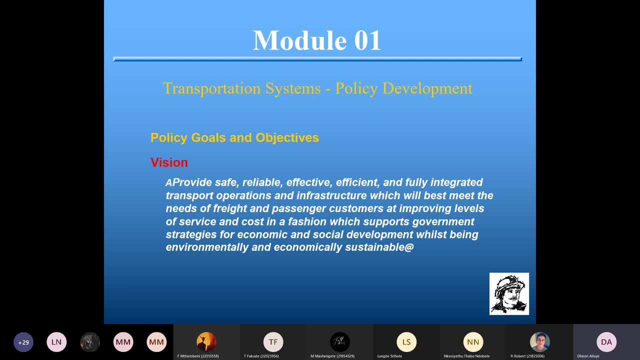 I was privileged enough to represent DUT in the formulation of this document, the White Paper on National Transport Policy. So I think if you go on to the Department of Transport, the National Department of Transport website and key in the White Paper, National Transport Policy, it will come up and you 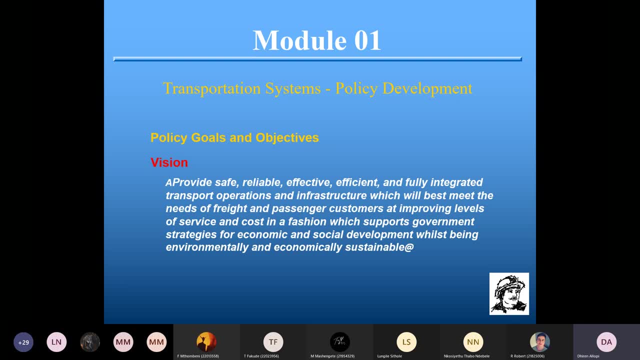 will see a lot of this information in there, like the vision, the goals, the objectives and so forth. So this is, like I said, a direct link to the White Paper And again, I'm not going to label it. You need to read through some of this information. 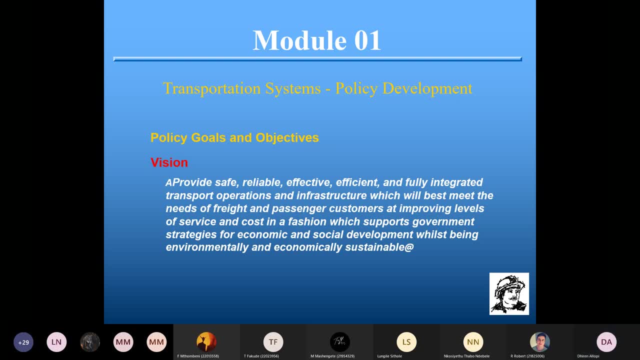 Like, for example, what is the main vision? And you can see from the key words like safe- providing a safe, reliable, effective, efficient, fully integrated system, And this is not only for customers- passengers, but also for goods or freight, something that 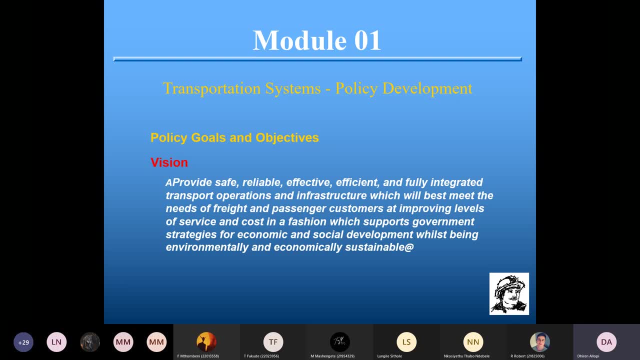 should be economically sustainable, And you can see the buzzword again: environmentally sustainable. So you can see all the necessary key words here, And one could then relate this to our public transport system, for example: How safe is it, How reliable is it? 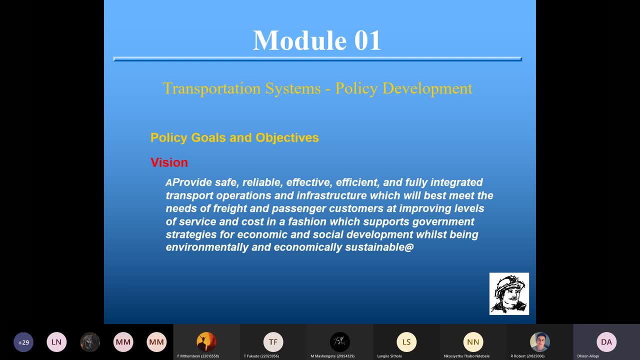 How effective, how efficient is it? How integrated is it? Can you move from one transport mode to another? Can you, for example, take a minibus taxi that will drop you off at the rail station, As an example? So that's where we refer to integrated system through ticketing system, where one ticket. 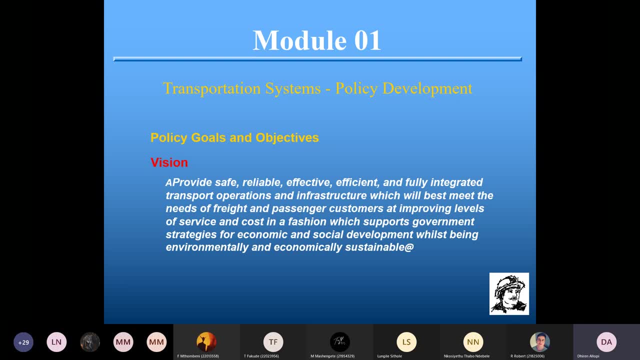 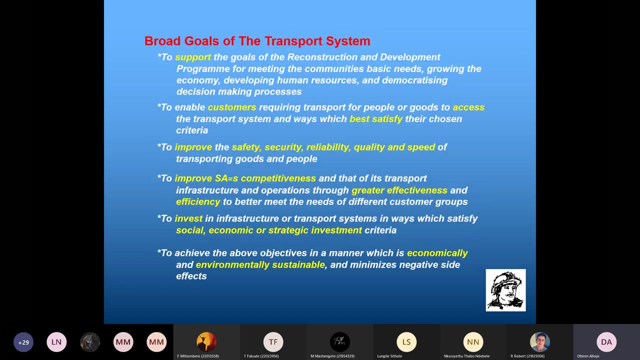 could move you from a bus to a monorail, to a ferry and so forth, And you can compare these to overseas examples as well. So we are certainly far back when it comes to- Okay, When it comes to- fully integrated transport operations. 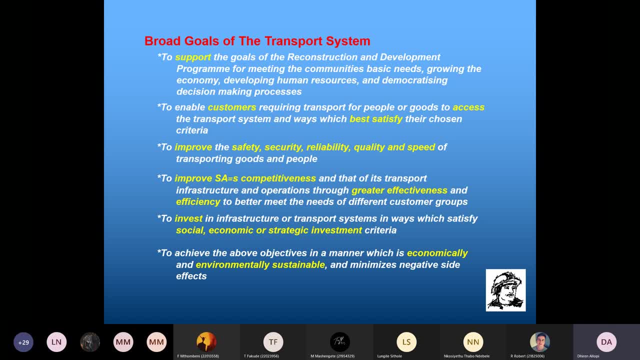 So the broad goals of transport systems and some of the keywords are highlighted in yellow. You can see that, firstly, that the goal is to support the RDP program to enable customers to access the transport system best satisfy their needs, certainly improving safety, security. 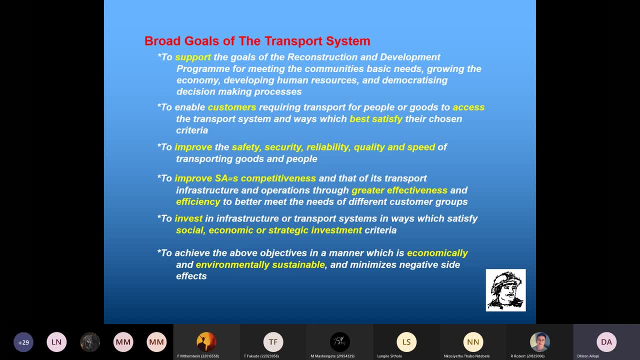 reliability. You perhaps would have noticed the steady decline, for example, in rail transport over the years. There was a time when rail was running at capacity. It was difficult for you to even get a place in a coach. Compare that to today. 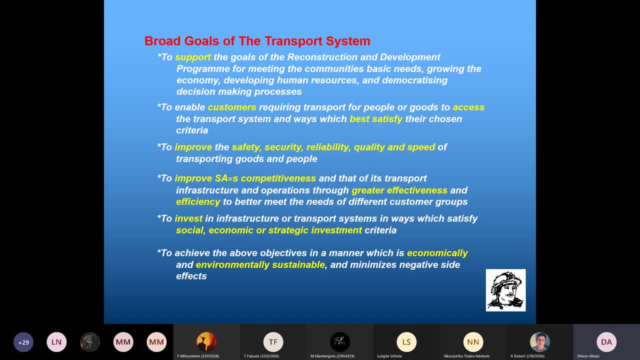 Many of your trains are running under capacity in certain areas. Okay, And there are a number of factors for that. Safety security certainly played a major role. There were times where it was okay for you to park your motor vehicle at the rail station. 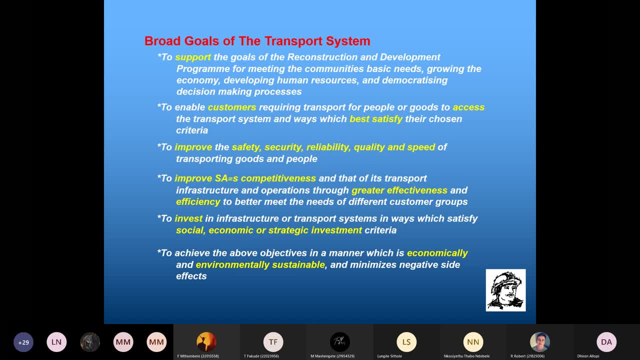 parking lot and catch a train to work, But then you come back and you find your cars gone or your sound system stolen. So you decide to use your private motor car to work and add to the traffic congestion. Basically, what I'm trying to say here is that there's a lot that needs to be done. 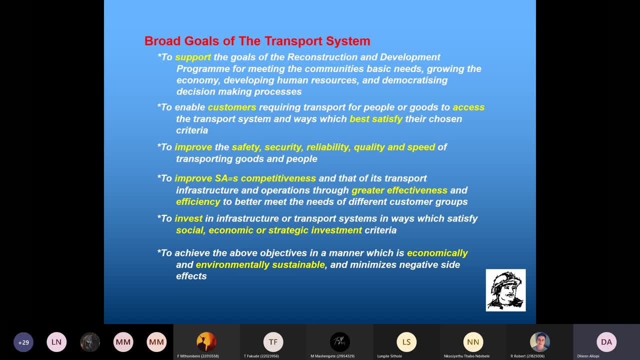 to improve safety, security, reliability, efficiency, effectiveness. as you can see in the next bullet, You must train. How long do you have to wait for another train? Half an hour, 45 minutes, one hour. So you're late for work. 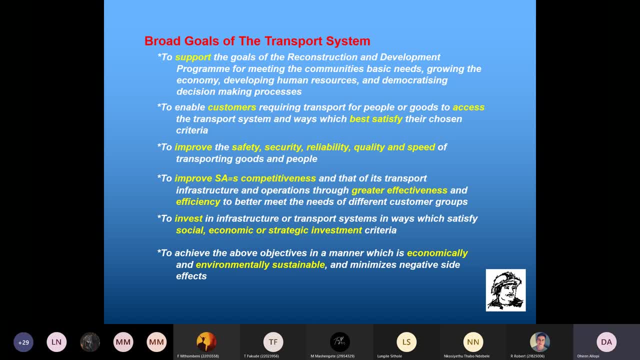 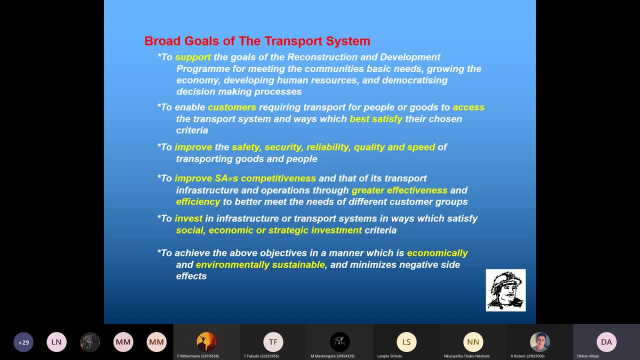 Accessibility of the transportation system. Frequency of service is what I spoke about. How long do you have to wait If you miss one train to get to another train? wait for another train Overseas if you are traveling, say, in the London subway, your rail system, underground rail network. 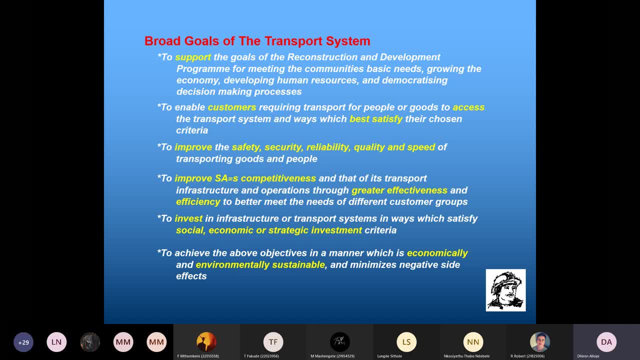 you miss a rail in a matter of five minutes. The next coach or the next train is there. So we talk in terms of frequency of service. So there's a lot that has to be done here in South Africa to improve safety, security, efficiency, effectiveness. 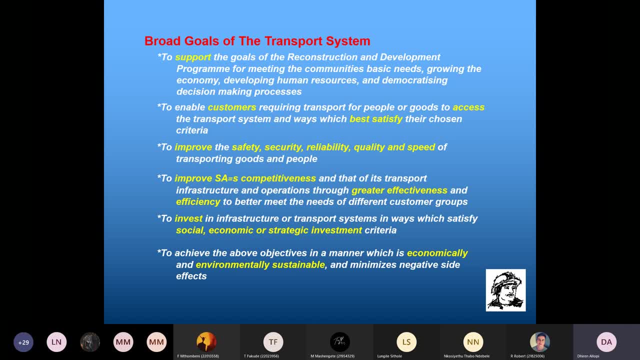 for people to switch to public transport mode. That is one of the reasons why our roads are running at capacity. That is the point I raised. your peak, AM and PMP: It has increased from half an hour to maybe two hours morning and afternoon peak. 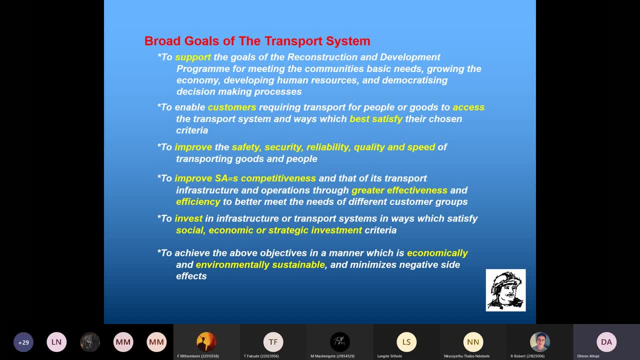 So the government National Department of Transport is trying very hard to try and improve public transport, to try and get more commuters back to rail. Just bear in mind rail has a very expensive infrastructure. The cost of building these rails are very expensive compared to the cost of running your trains. 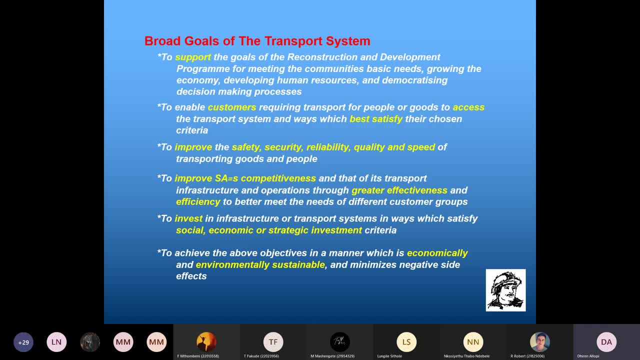 Very expensive. So you have these very expensive infrastructure that's underutilized. The government did invest lots of money in these transportation infrastructure, So one needs to get mileage out of it. Yes, and of course the last one, to achieve the above objectives economically, environmentally sustainable. 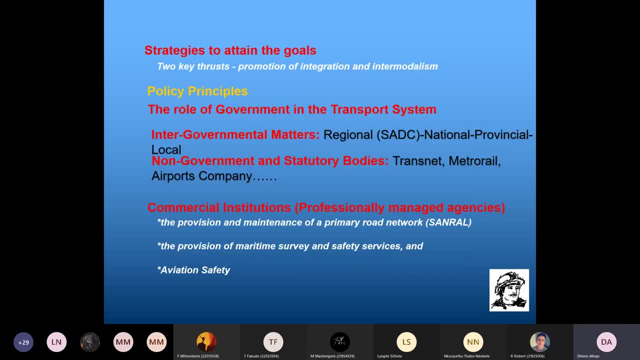 So there's some information on your note that deals with the policy aspects relating to government and the lower levels below national government. So, in terms of the strategies, you will see the key thrust there is promotion of integration and intermodalism. I spoke about integration. 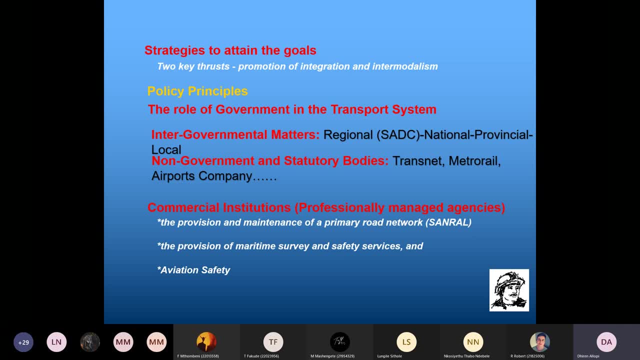 Where you should be able to move from one mode of transport to the other mode of transport without any problem. And there again we spoke about, if one has to take, for example, the rail system, certainly accessibility is an issue. Not everyone is close to a rail network or to a rail station. 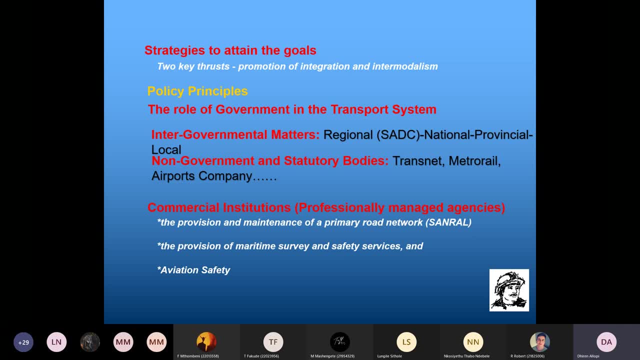 You may require, you may need to work, You may need to work, you may need to walk two, three, four, five kilometers to get to the nearest rail station. so, with effective integration, if you had, for example, an effective mini bus taxi system that could pick you up right at your door and take you to a rails station, 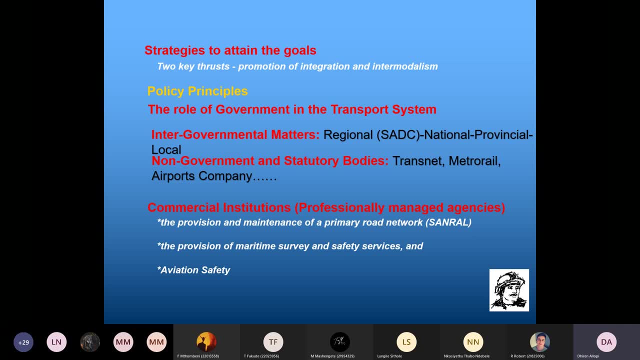 and you then catch a train to work. hopefully, on the other side you have a rail station that's close to your work. what a pleasure that would be. so we're talking of promoting integration. there has to be more buy-in between or amongst the various public transport operators, whether 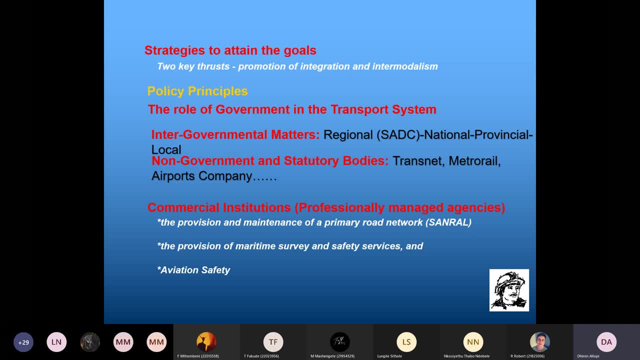 it's minibus, taxi, whether it's rail, whether it's bus. intermodalism also: if you get to the airport to catch a flight, how efficiency is it? how efficient is it for you to be able to catch that flight? was getting to the airport via the mode that you have? whether 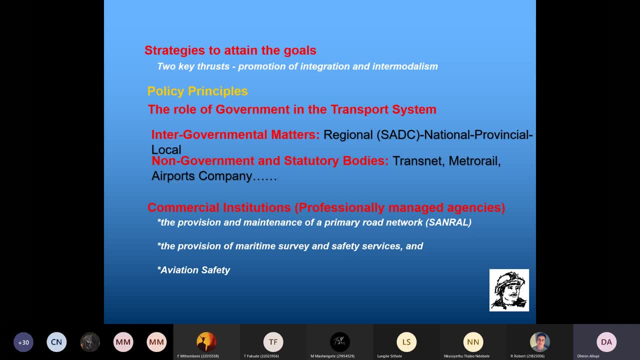 it's car, motor car or bus or minibus, taxi. so those are the two key thrust areas that we're referring to. we tell you, with regard to policy principles you will find in your notes and you need to go and highlight this information and then go to your notes and look at this information. 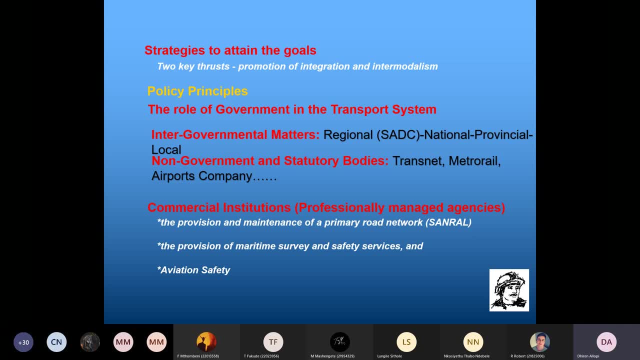 pertaining to the role of government and transport systems. so you'll see, national government plays quite a large role but, at the same time, also delegating powers to different authorities, different bodies. so you can see, with regard to inter governmental matters, right from a national to a provincial, down to a local level, and then 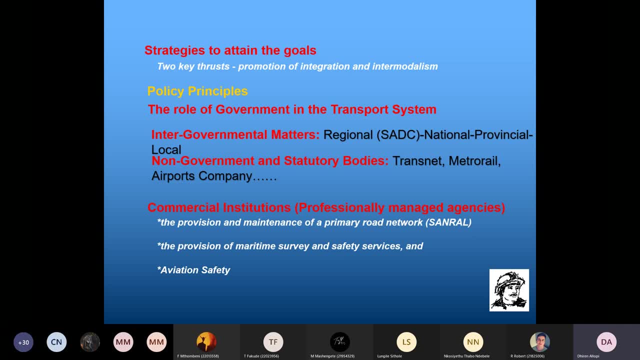 you have different statutory bodies like transnet, metro, rail, airport companies, and you can see a whole lot of them listed in your notes, okay, and then when we talk in terms of professionally managed agencies, you will see, for example, sandra. anyone knows what sandra means, stands for sandra. 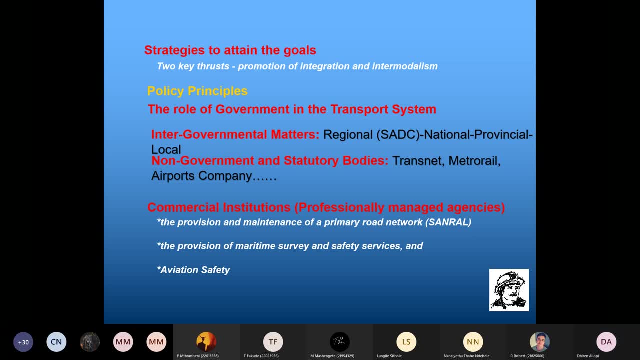 anyone, okay, so it's basically the south african national roads agency and they handle a lot of the maintenance of the road network. so they are so-called a, a professionally managed agency that that's contracted to the government. so you have similar agencies when it comes to maritime, maritime deals with water. when it comes to aviation, you have a. 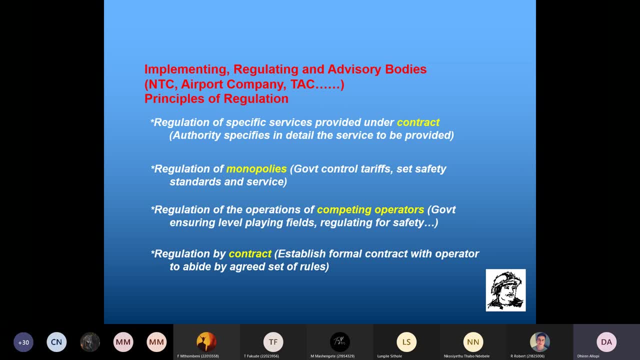 transport, and so we have then different advisory bodies and again, if you look at your notes you will see the diff: the national transport commission and the national transport commission, there's airport companies, the um transport advisory council. so there's various advisory bodies and these provide the necessary services by various elements or factors. 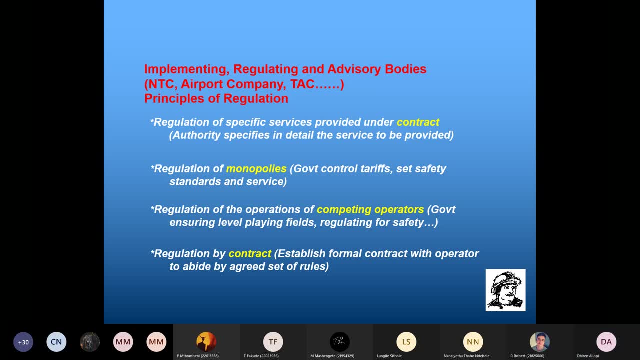 or methods means could be under contract, so it could be provided under contract. so, again, if you look at your notes and things specifically, you're looking at page eight in your notes, the section So you can see the highest form of regulation is under contract, Like, for example, 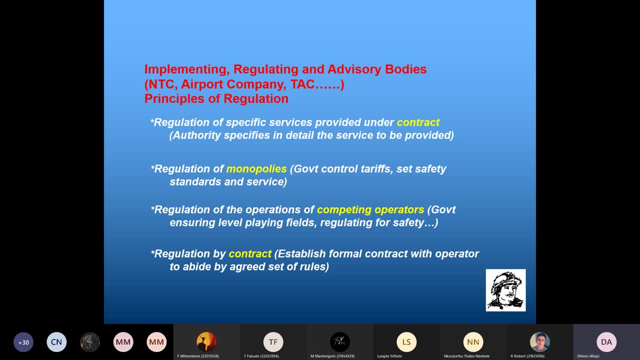 if one takes the commuter rail service that's provided under contract, and then you could have monopolies. with monopolies, you will find that the government is the main controller, controlling, for example, the tariffs, setting out your safety standards, the service for 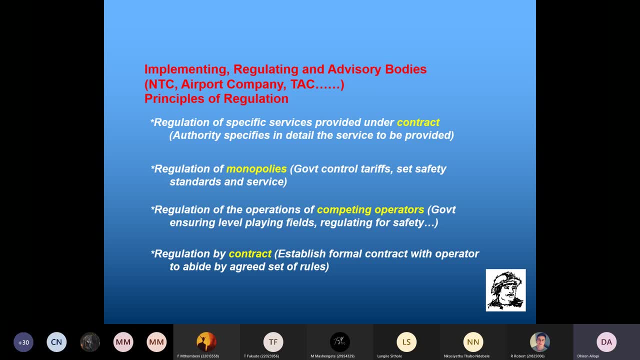 all that could fall under monopoly. And then you have competing operators And I think with competing operators it's very important to know the safety aspect, regulation or regulating safety. Very often when you have maybe two taxi operators operating on the same route, 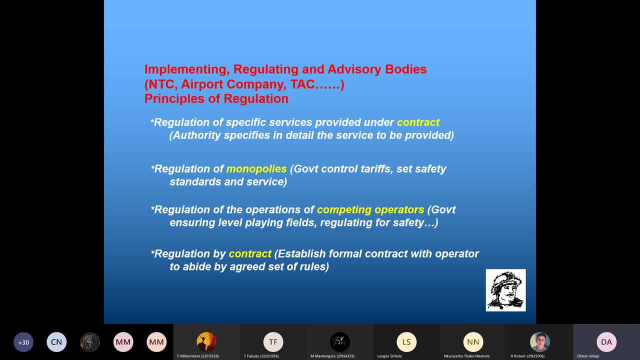 you know the problems with that- the taxi was that we experience. So it's very important how one goes about dealing with competing operators. And then, of course, by contract. and when it comes to contract, where you form or establish a formal contract with an operator, say a bus operator, and that bus operator then will. 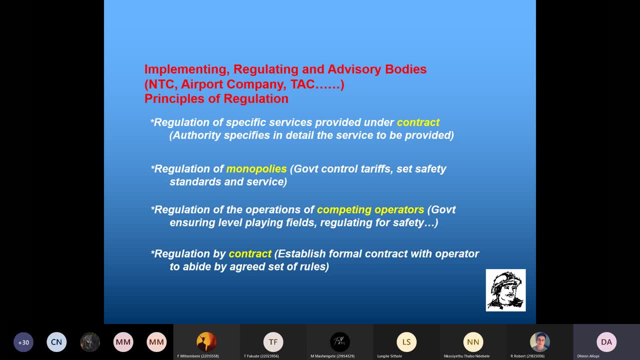 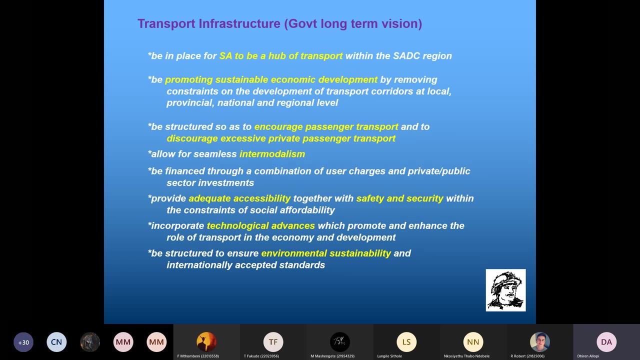 have to abide by the agreed set of rules. So, again, if you go to your notes, you will see a little more information on this. And then, finally, the government's long term vision. And if one goes through the government's long term vision, see the promotion of sustainable economic development. So at the end of the 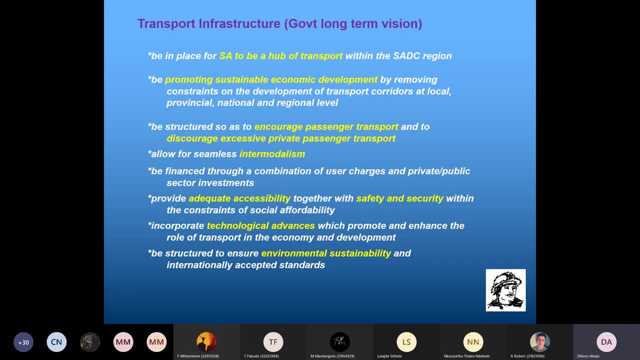 day. we all want to play South Africa in a hub of transport within the SADC, that's your South African development countries, developing countries. So we want to be the best. So in order to do that, obviously we'll need to satisfy certain conditions, That's the government's. 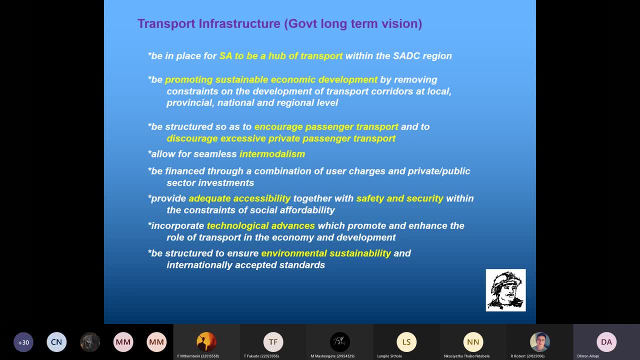 long term vision To encourage passenger transport. you can see it comes up again: encourage passenger transport. we don't want to be like the Americans that thought they will solve the transportation problem by building six lane and eight lane highways and byways and freeways and expressways. 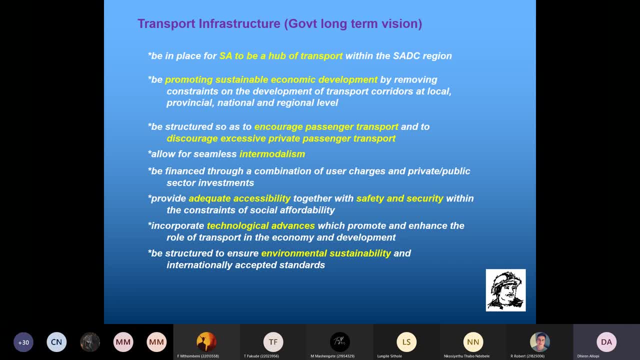 And in a matter of six months you have systems failure. your roads are again running at capacity due to the increase in car ownership, increase in car usage on your roads didn't pay much attention to improving public transport And we are also now in a similar boat. you'll be surprised there's so. 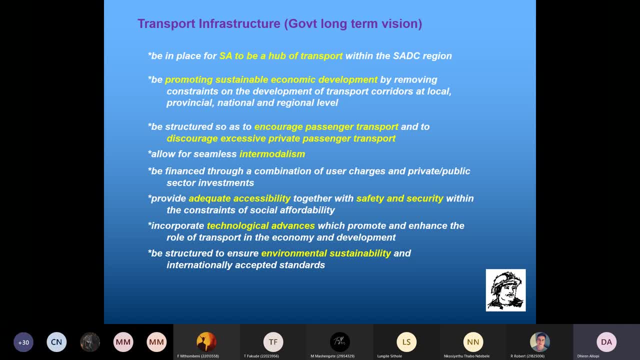 many cars on the road during the day. I sometimes wonder whether people walk. They spend most of their time on the roads traveling. I'm sure they are all not special agents, reps, that spend the day on the road. If you take 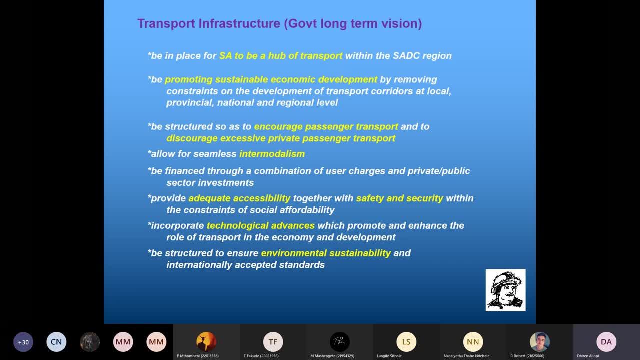 Kauteng, the Benskuman Highway that leads you from Johannesburg to Pretoria. Benskuman Highway is commonly referred to as the Benskuman parking lot. Your vehicles are more stationary than moving. That trip could take you anything up to. 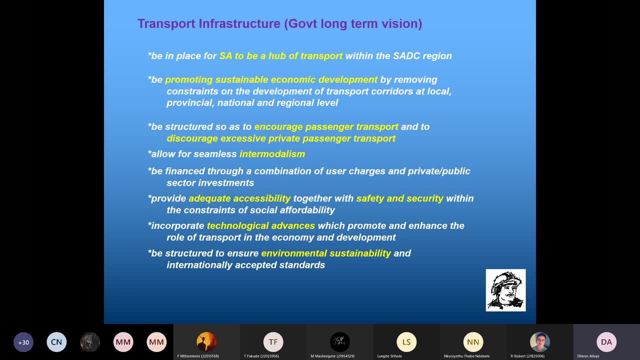 two to three hours, depending on the morning and afternoon peak, to get from home to work and back, So you spend 50% of your time on the road. That's not good, isn't it for the economy of the country? 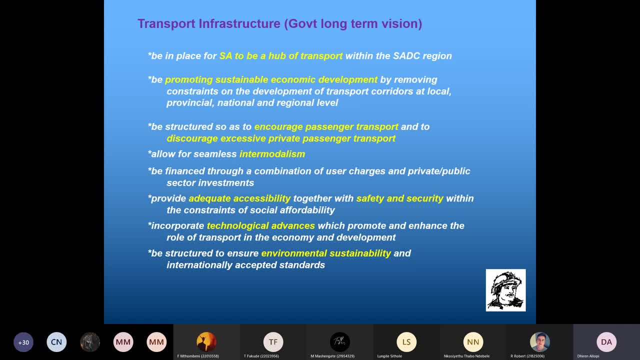 So you can see, public transport can come to the rescue And therefore the Kauteng was certainly a success project. You know, the Kauteng links right from the airport, The airport to Shantung City, all the way through up to Rhodesville, that's in. 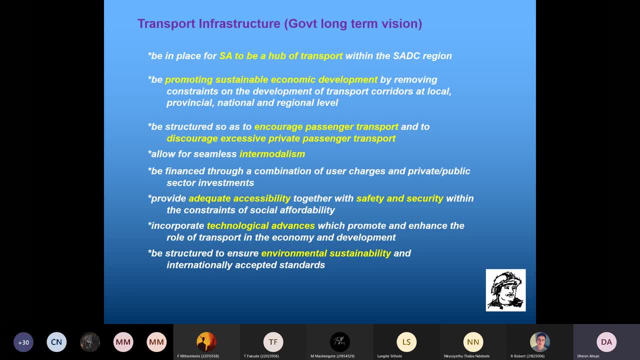 Pretoria. So many, even hi-fi, businessmen park their vehicles, Let's say maybe the Shantung Station, and catch the Kauteng to Pretoria. The trip on the Benskuman Highway could take you maybe two to three hours, whilst on. 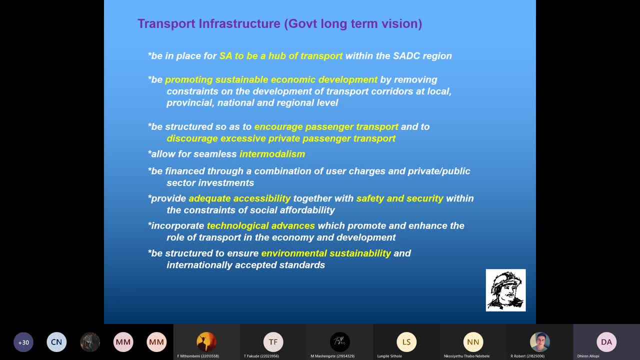 the Kauteng: 32 minutes, Big difference. So the government is trying very hard to promote public transport and, more specifically, the rail transport. Why Rail has its own right-of-way. it's separate from your road network so it has its own dedicated right-of-way, can maintain speed and, more importantly, it's a high-capacity mode of transport. 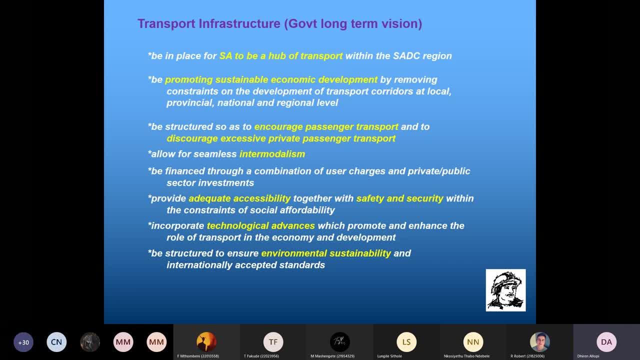 You do the math. take a train with 10 coaches, work out the capacity of each coach times 10, how many commuters you can travel. you can move, You can travel. you can move In one train And then compared that to: 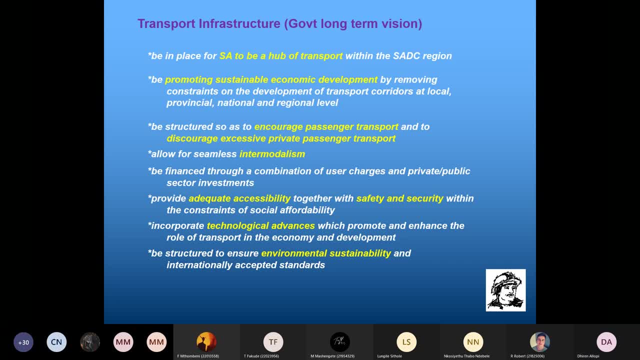 your road network. Do a little observation, little survey: See how many vehicles on the road has just one occupant: the driver. Therefore, you will find that in some areas, in terms of traffic management techniques, they've adapted a principle: HOV, high occupancy vehicles and 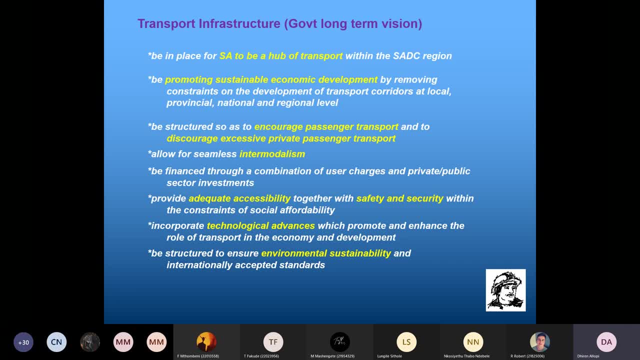 occupancy vehicle lanes. So you only allow to use that lane if you have more than maybe two or more than three occupants in the vehicle. Otherwise you join the congestion on the other lanes. So you can see some of the long-term goals: Seamless intermodalism from one mode to another. 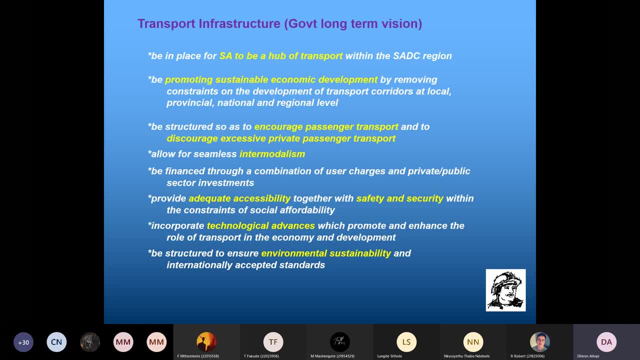 Adequate accessibility. We spoke about the poor accessibility, especially when it came to rail network. Many people may question or argue or criticize the minibus taxi industry, But bear in mind that the minibus taxi industry has played a very important role in the public transport operation. 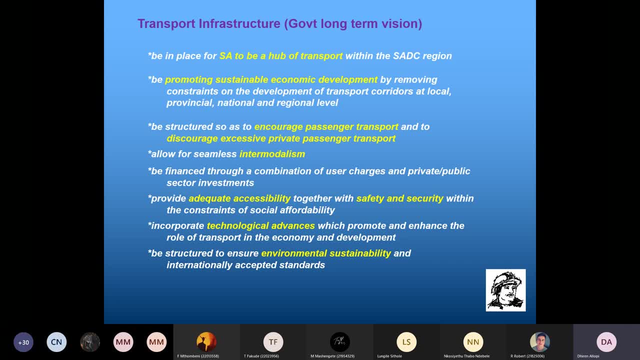 Yes, it comes with some bad, poor baggage in terms of safety, in terms of reliability maybe, But when the rail system was failing and the main reason for that was accessibility and frequency of service, there came about a public transport operator that gave you a door-to-door. 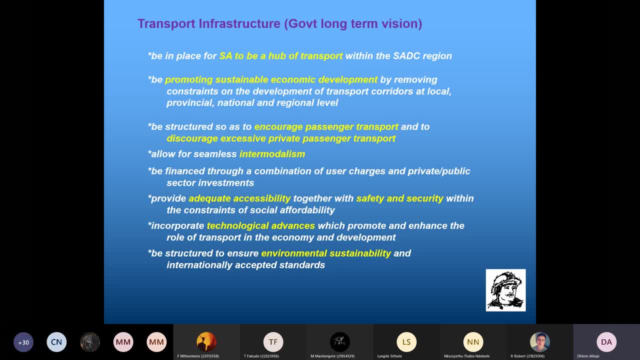 service- Minibus, taxis- picks you up at your door and drops you off at work. Obviously, people will then move to that mode of public transport, But there's a lot of issues pertaining to, like I said, the safety, the security, and also pertaining to the subsidy aspect. 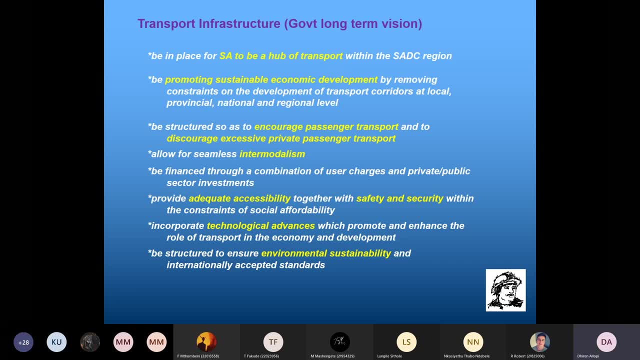 You may have heard in the news that very often the minibus taxi association they go on strike because of not getting the subsidy from the Department of Transport, Like many of the bus services do get. the rail service gets the subsidy and the minibus taxi association gets the subsidy. 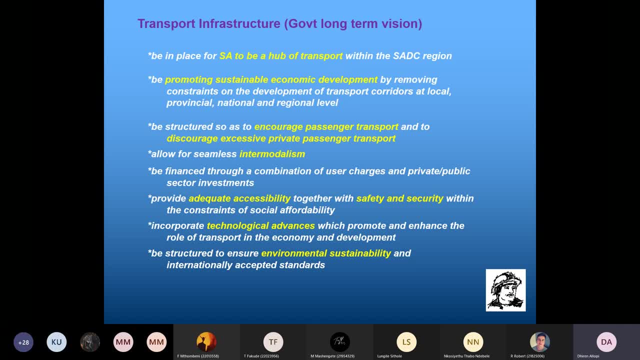 So there's a lot that here we need to do in South Africa to try and address those issues. When it came to safety and security, you know that the Department of Transport then tried to move away from the old minibus taxi to the new, safer system where an amount was given to the public transport operator. 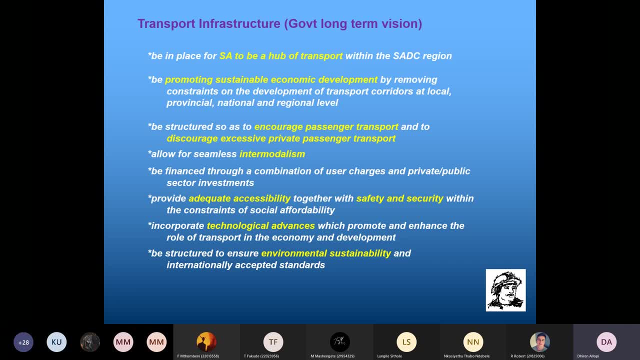 or the minibus taxi owner to move to buy the new vehicle And a certain amount was paid, And a certain amount was paid For the older vehicle. So you may have come across all these in the news, And now, of course, we have the BRT system. 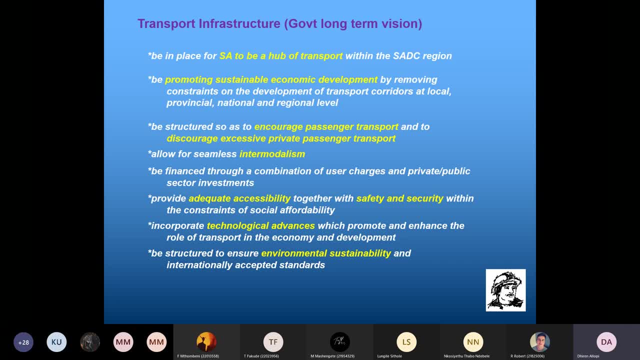 Perhaps heard of the BRT system. Anyone knows what BRT stands for. BRT anyone? Okay, it refers to the bus rapid transit system. The very first one in South Africa was constructed in Kauteng: the Riavaya system, the BRT system that linked areas like Soweto to the CBD. 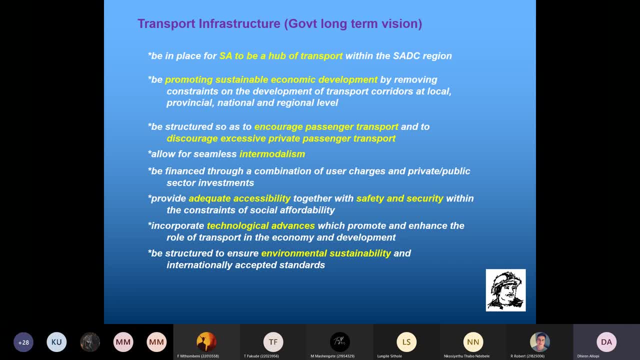 So the BRT system, where you have these specially designed buses, has its own right of way and very often given priority at places like intersections and so forth. the BRT system- And it's free of the traffic congestion, So people can then move to a much more effective and efficient system. 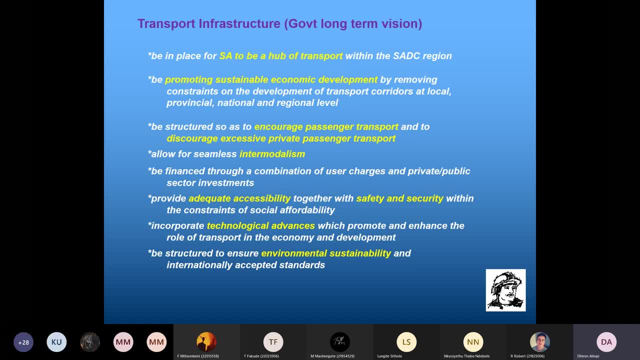 So South Africa- we have a few now. Next was Cape Town, and then KZN came about with their BRT system, And there's various routes that have been planned for the BRT system, Like, for example, from the CBD to Pinetown Gateway Complex to Pinetown. 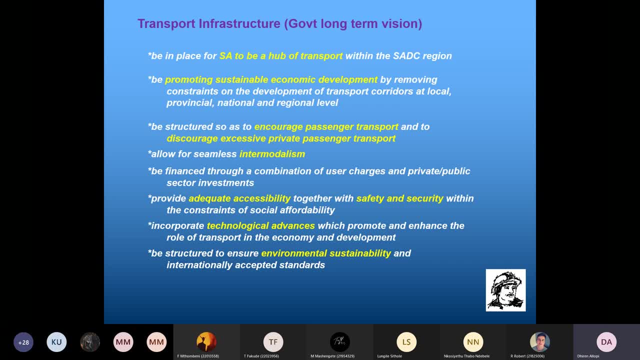 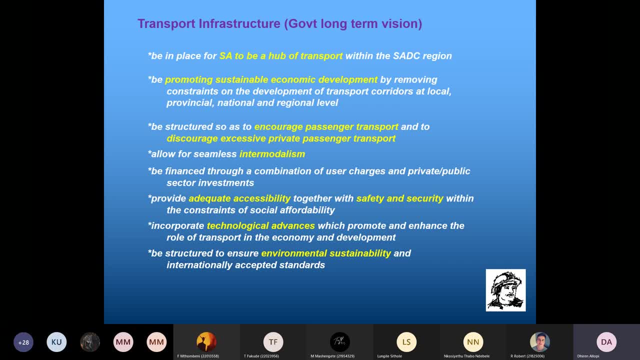 There's a lot going on. You can see, then, the government is trying their level best to promote public transport. So that brings us then to the end of Module 1.. Let's try and stop presentation And maybe we have some time maybe touch a little bit on Module 2.. 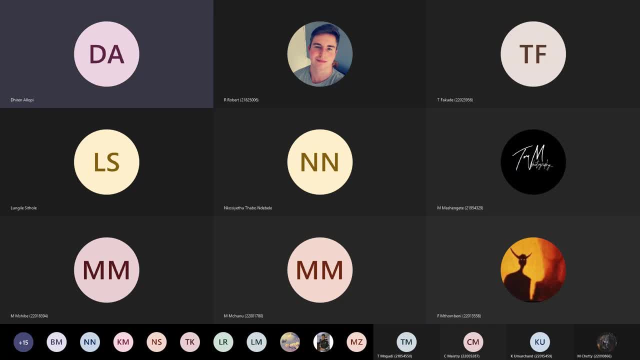 And maybe we have some time, maybe touch a little bit on Module 2.. Syllables for Transport Technology: 3A is not a long syllabus. It's not a long syllabus. You will complete the syllabus well within the time limit. 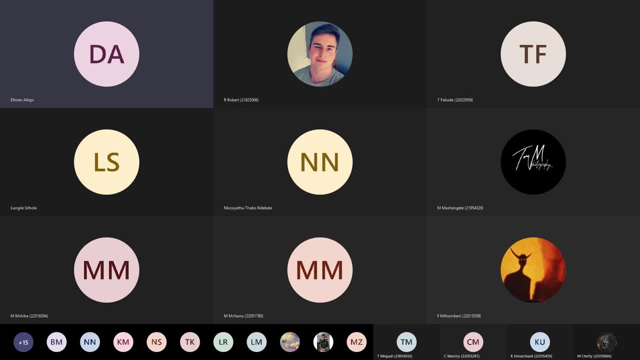 or the time factor. But, like I said, a lot of work has to be done on your own as well, So you need to then go. Your main academic hub, like I said, is Moodle right, Your main academic hub, like I said, is Moodle. 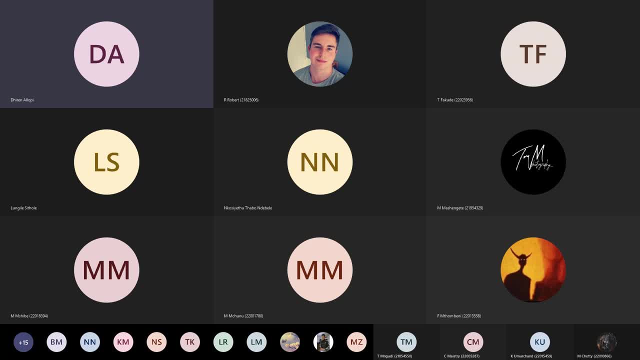 Your main academic hub, like I said, is Moodle, Then you can, like I said, when you find a job or a profession, The Moodle application model. So you need to go and cross reference what I've done with you today and link it. 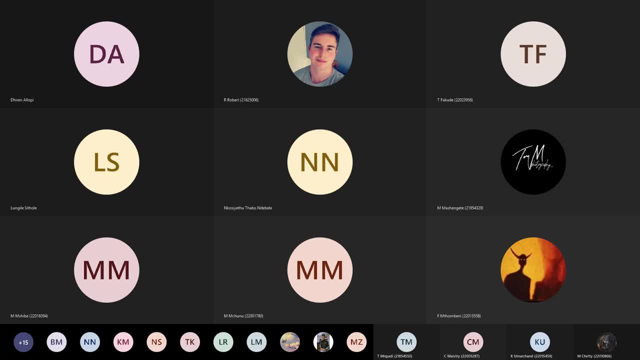 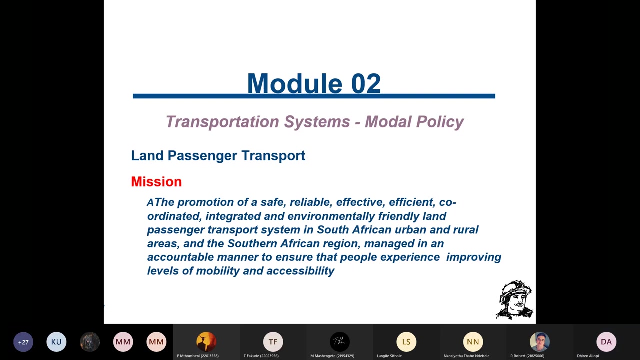 to model. Let's see if I can find it. Hopefully it will open here. Let's see Replace that. So there we have module two then, And this module again deals a lot with the policy aspects. So again, I'm not going to labor this and go through word for word. It's not the intention. 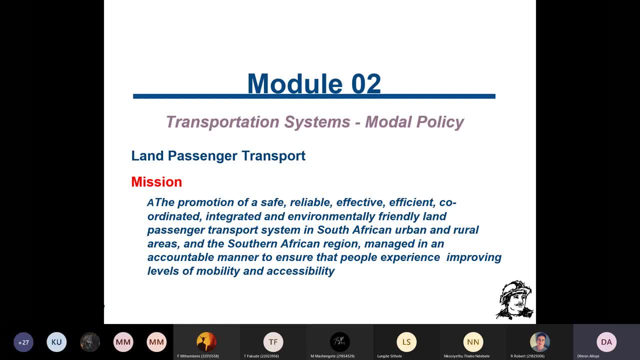 of this presentation. But to highlight again the keywords and the onus is on you to go back and read through the information And, yes, if you have any issues, any problems, any questions, yes, feel free to bring them across and you could do it at the lecture. you could post it on model email. 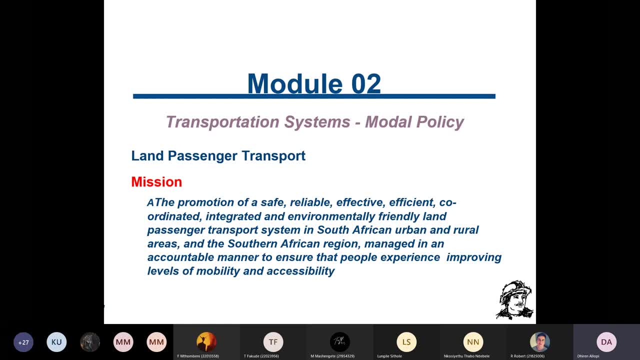 good enough. i think if you are registered, then you all should be linked now to moral ms team and email so you could expect communication from any of those sources. so there you have, land passenger transport and again the mission very similar to the module one that you looked at from your white paper. again, this is from your 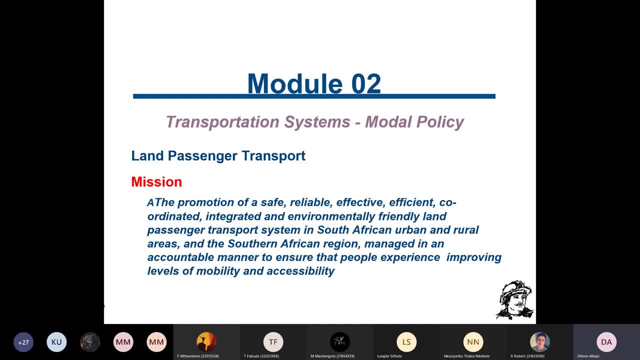 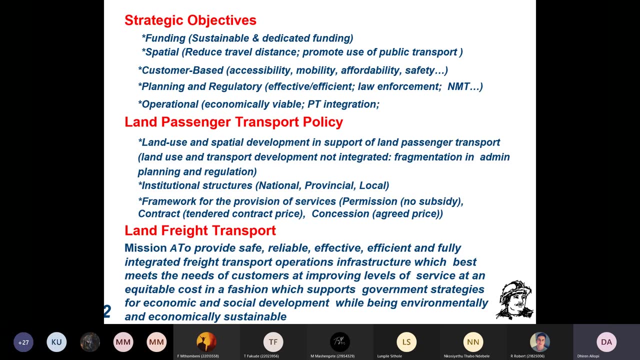 white paper also on national transport policy, promoting safe, reliable, if you effective, efficient court. so here we're looking at passenger transport, land passenger transport, and then you have various strategic objectives, ranging from funding, spatial, community, customer based planning to operational, and if you take each one, when we talk in terms of funding, yes, 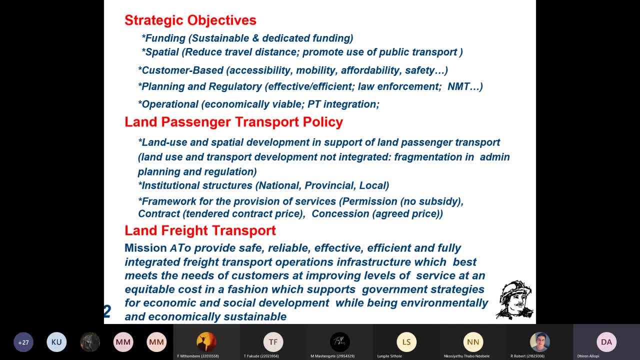 it has to be sustainable, should have dedicated funding. when we refer to spatial reducing travel distance, promoting use of public transport, you can see it comes up again: promoting the use of public transport. when we talk in terms of customer base, yes, how accessible is the mode of transport? affordability and again, if you look at the white paper that i was, 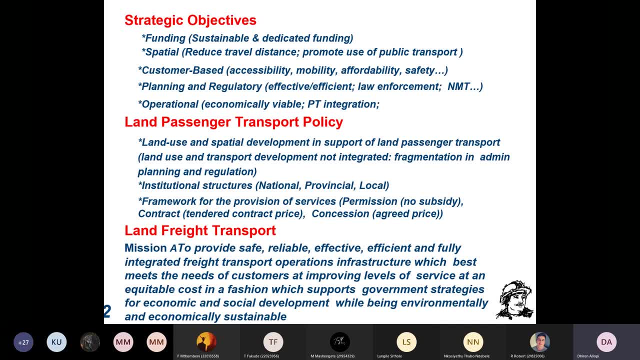 referring to you will see someone in the white paper mentions that should not be the. the cost of transport should not be more than 10 percent up to three percent sales tax account, which means you doesn't need a seemingly fool a Dae afraid you as well. it's a goodDING move to be able to ensure that. 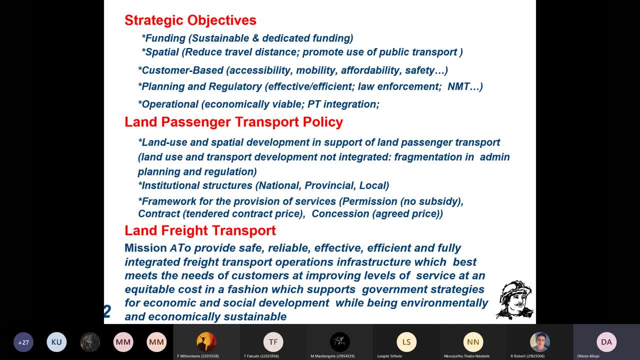 track personal integration during toward application. only does Santa California look like. that percent of monthly salary, that's your monthly cost of transport, should not be more than 10. you'll see the mention of 10 in the white paper. safety again comes up: providing a safe transport. 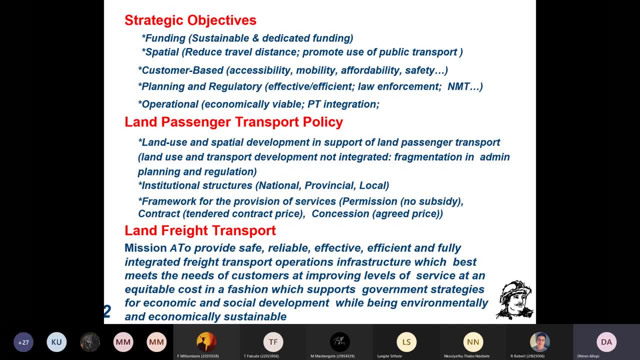 when it comes to planning and regulatory aspects. again, effectiveness, efficiency. law enforcement also comes up in terms of planning and regulating. uh, pointless having a system without a proper law enforcement, and one of the problems that you will find here in south africa when it comes to law enforcement is, for example, at traffic lights. 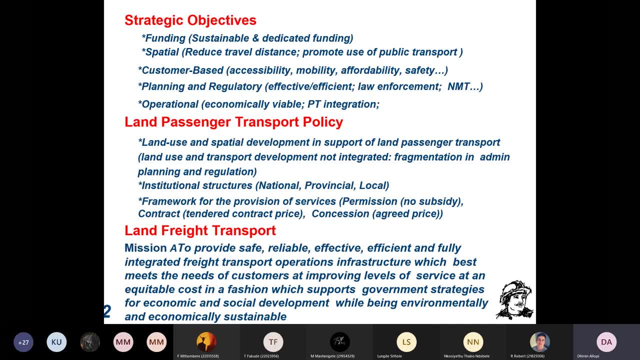 some drivers, some motors, only see a green light. they don't see a red light. red means stop nmd- non-motorized transport. again, the department of transport has made huge funds available for projects pertaining to nmt- non-motorized transport, providing proper pedestrian parts. 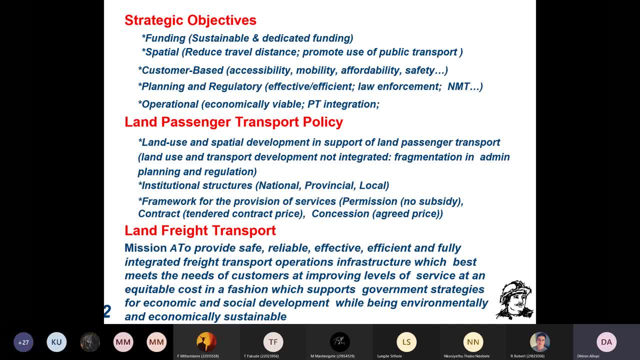 providing proper cycle parts where people get off the motor car and maybe get onto a skateboard and cycle and then skate from a to b or cycle or walk, so promoting healthy living as well by walking operational and with the operational you can see the mention of public transport integration again. 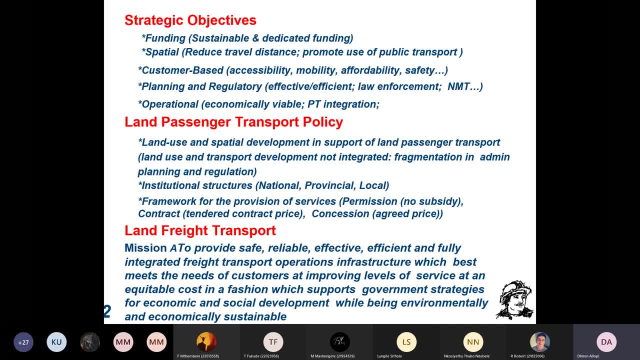 so land passenger transport policy. if one looks at the land passenger transport policy, you will see again the development and support of land passenger transport and you will find words like the planning and regulatory aspects coming in, the predatory. and then you will see the the various bodies that are involved, right from national level to local level, the different. 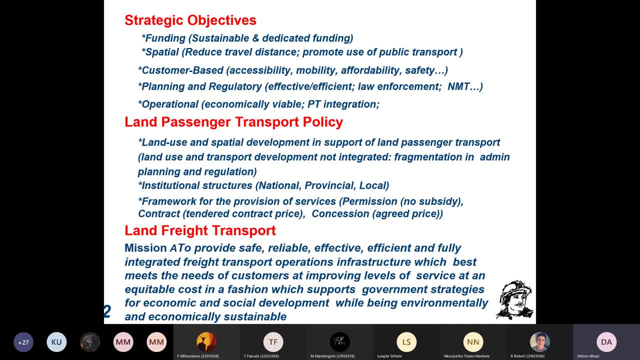 structures. you will see also the under land passenger transport policy, the mention of various types like permission, contract, concession, and one will then need to know what is the difference between permission, contract and concession, and you can see the keyword there in brackets. so if you were given the permission to operate on a particular route from a to b, 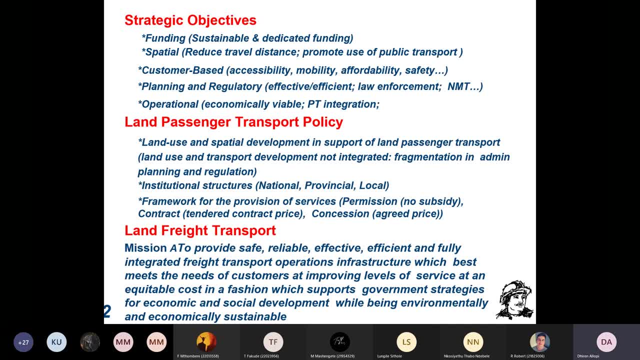 permission means with no subsidy, okay. contract means a tendered contract price. so you tender and depending on your tender price, not necessarily having the lowest price. very often, yes, it goes to the lowest tender that that pertains to be a contract. when we talk in terms of concession, 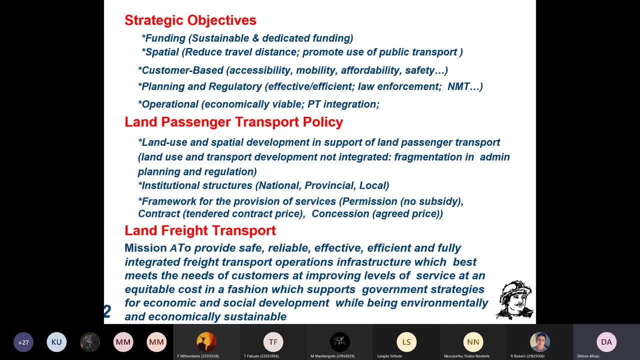 is where an agreed price, so what the uh authority and the greed price is decided and that then the terminology for that we use is concession, so that dealt with land passenger transport and similarly. you then have land freight transport, now freight with referring to your goods and so forth, and 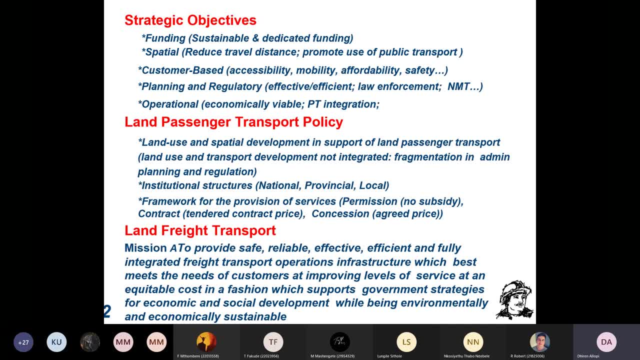 again the issue of safety, reliability, efficiency, effectiveness again comes in to provide a provision for freight transport, very importantly, if you can. you imagine now you are transporting um butter from turban to johannesburg and by the time the butter reaches johannesburg it's in liquid form. 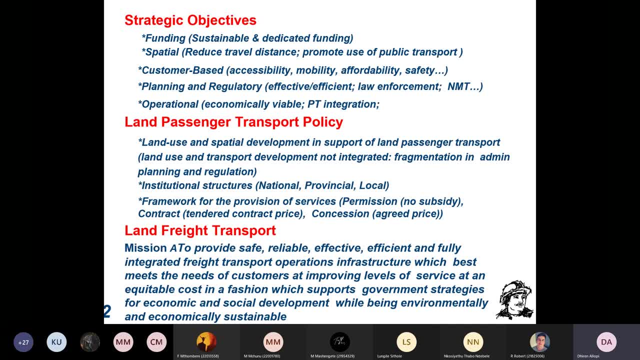 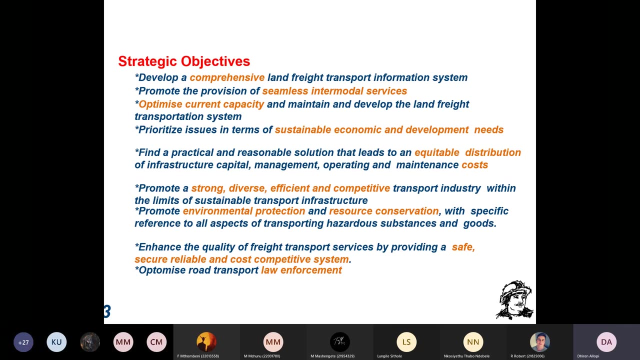 that's not the end result you wanted, isn't it? so you got to ensure that you have the proper container, proper refrigeration process in place to transport that item from a to b. so these are points that one will need to take into account in terms of strategic objectives. also, one needs to have a proper, comprehensive 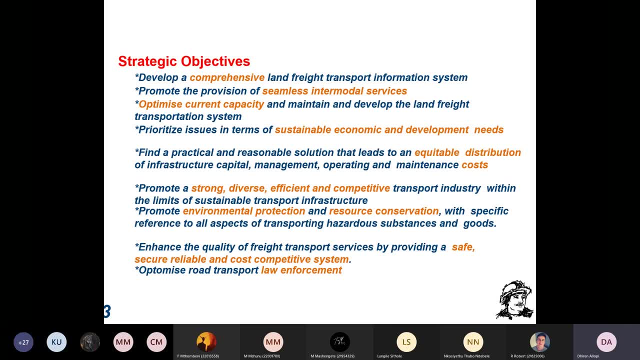 system in place. and again you can see the word seamless intermodal service from maybe road to a or road to water. and how often you notice these containers, for example, transported by road, sitting at the container terminal waiting to get onto a ship time factor. that's why we say provision of seamless. 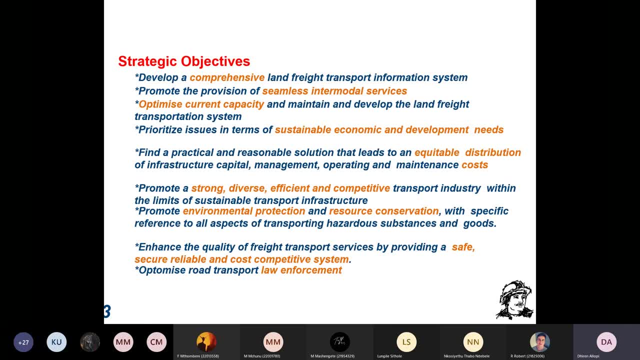 intermodal service. now, optimization of current capacity, and that's the point i raised a short while ago, where many of our rail systems, our trains, coaches, running under capacity, need to optimize the current capacity, make them more safe, efficient, effective, increase your frequency of service, work on the accessibility aspect. so these keywords are very self-explanatory and you can go. 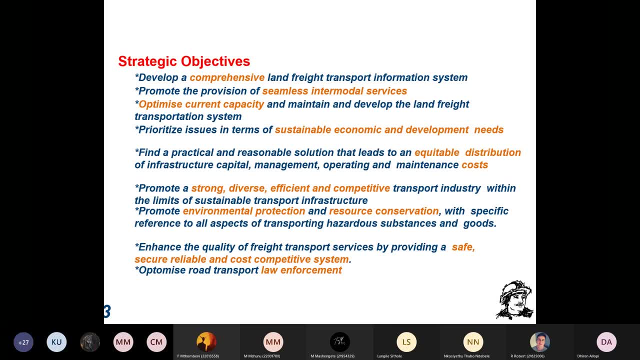 through them, read through them in your notes again. you can see cost factors come in: maintenance cost, trying to promote competition- very important. when you have competition in your industry, any industry- there's a need. then there's some goal or some drive to make it more efficient, make it more. 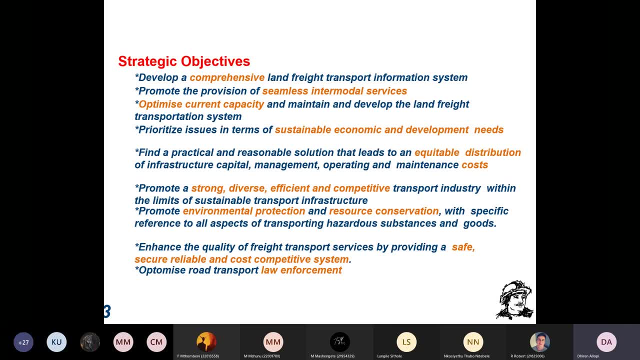 effective, otherwise people will move to the other system or the other organization or the other business or the other product. so competition is very important. that also implies, like i said, it could apply to any situation. you compare prices of coffee at pick and pay and checkers and 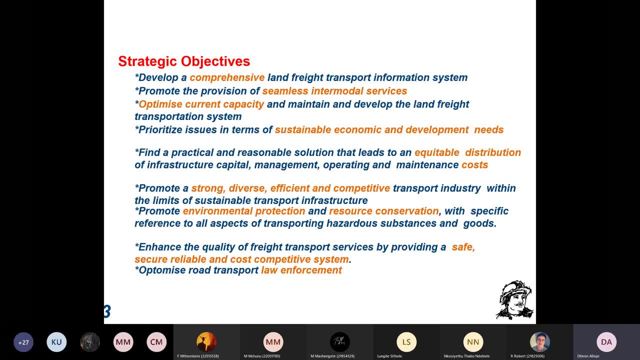 spa and that's where the issue comes in. where would you buy that product from? so competition is very important. obviously it's a positive spin-off for the customer. so environmental protection: i spoke about the issue of having a proper environmental impact assessment report with every tender, every project and you can see safety aspect again. 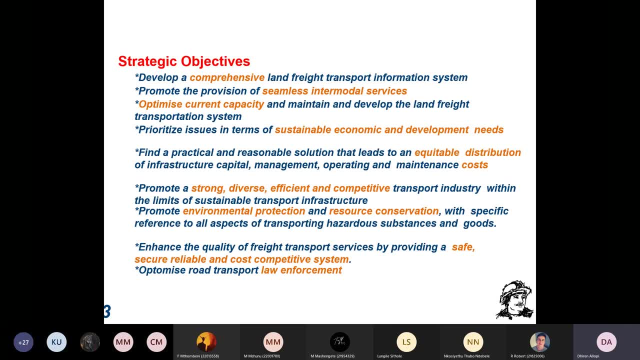 if you have a lot of infrastructure and you have a lot of construction, you do a lot of work. you, you do a lot of work with the company to make sure that they are reliable, optimizing your law enforcement. in some areas, overseas, they so hi-fi in terms of technology that if you are 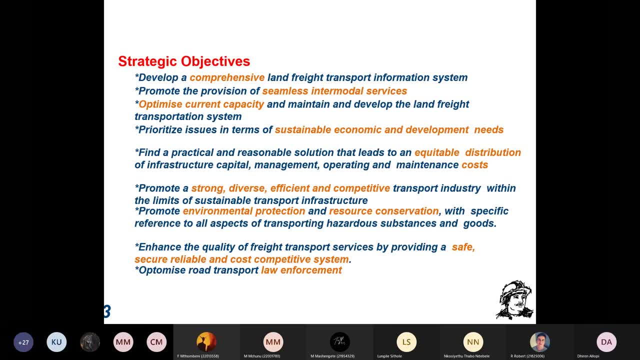 traveling on a particular highway and you exceed the speed limit, it actually comes up, gives you a warning that you're exceeding the speed limit. slow down so like, if you compare, for example, the very effective. that is why you'll find that their accident rates are very low compared to. 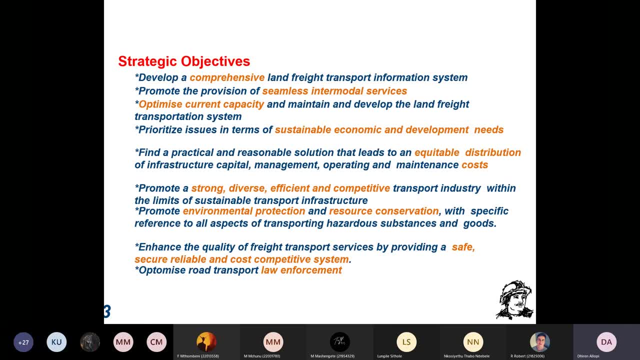 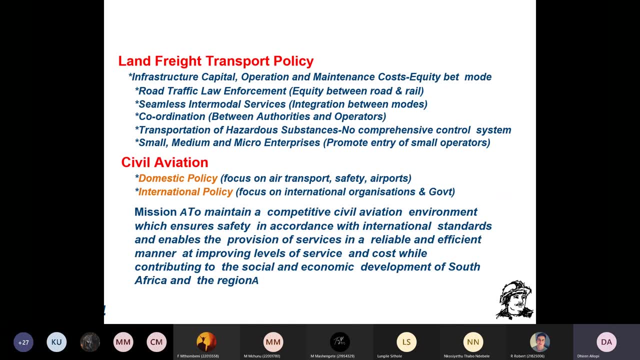 us. south africa is, i think, amongst the top three worst in terms of accident rates, and there was a time when the national department of transport made huge sums available for research in this particular area topic in terms of safety, okay, so land free transport policies- again you can. 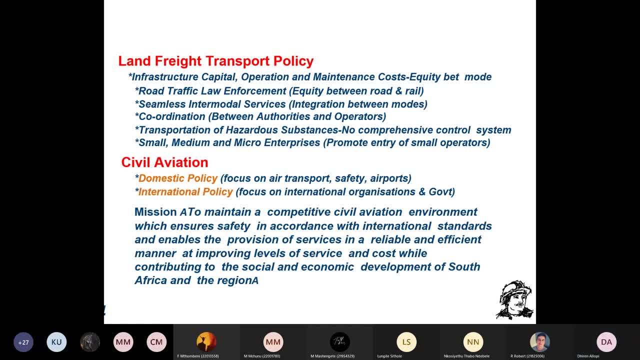 see the law enforcement aspect. equity- equity between road and rail. yes, this is something that has been going on- this debate has been going on for many years now- where a lot of the heavy freight was previously transported by rail and now a lot of that has been transported by road. how often you see these huge trucks? 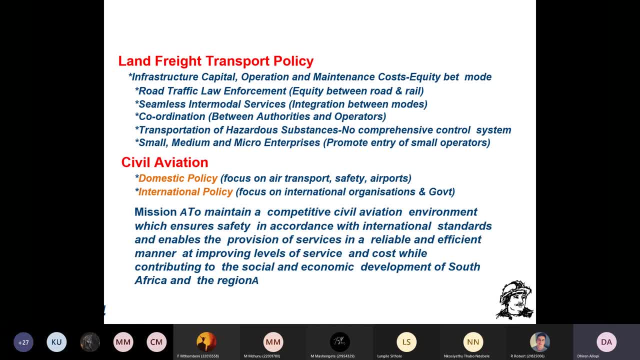 with huge containers, a huge equipment on them, transported by road. remember your road could last a lifetime if it catered for just certain class of vehicles in terms of e80s. e80s is your 80 kilo newton axle load on your road. so if your road was accommodating. 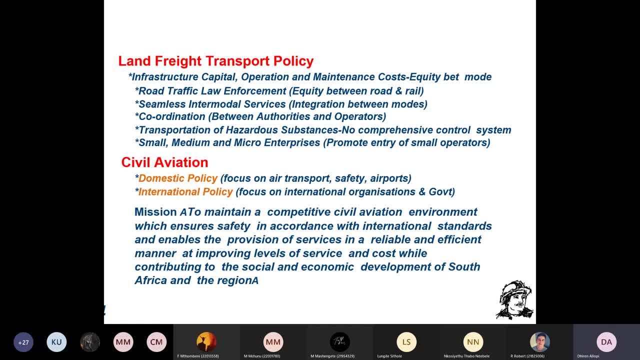 certain amounts of e80s within a certain class, it could last a lifetime. but the moment you bring your heavies onto your roads- high number of e80s- certainly your roads will not last and therefore you need to maintain your roads regularly. so lots of talks on this area, in terms of trying to move heavy's back to rail from road. 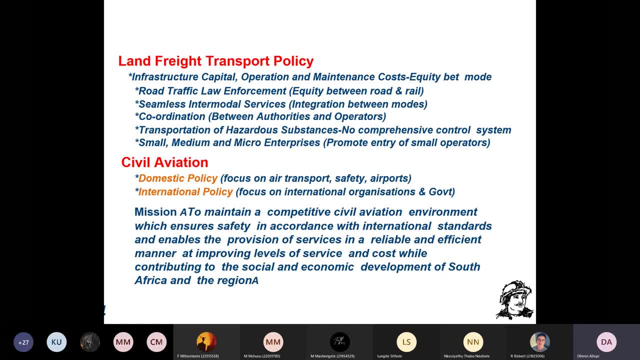 we spoke about again the intermodal services, integration between modes. there must be proper coordination, communication between the various authorities and this also has been a problem where, for example, the town planners don't talk to the transportation planners, they don't talk to the transportation planner, they don't talk to the transportation planner. 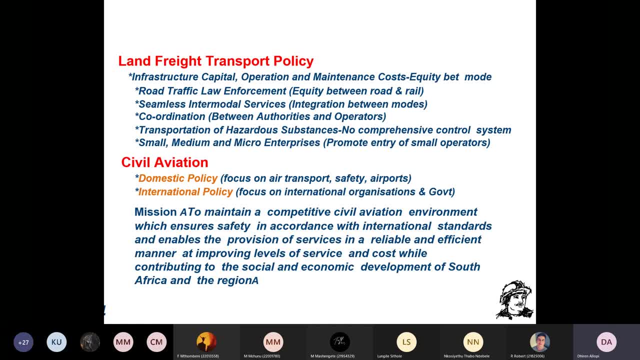 as a result, you don't get the proper road network, for example in a particular development or a new development. local authorities don't national, so monies are then allocated for a particular area for for provision of road network. the local authority thinks that the provincial authority is handling it. 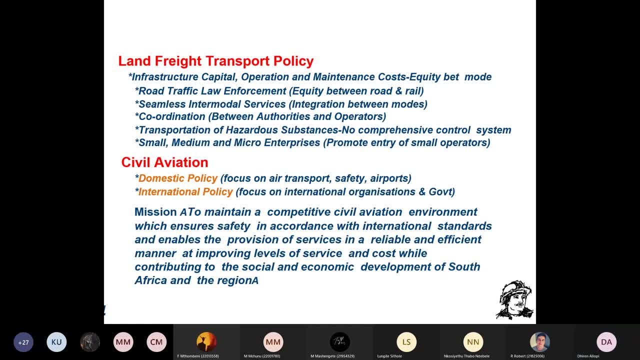 no one handles it and the money goes back to treasury, poor communities sitting waiting for the roads to be built. so you see why it's important to have proper coordination. again, transportation of materials, chemicals, all this one needs to take into account giving provision or allowing open the path for small operators, promoting small operators. so these are all covered in your land. 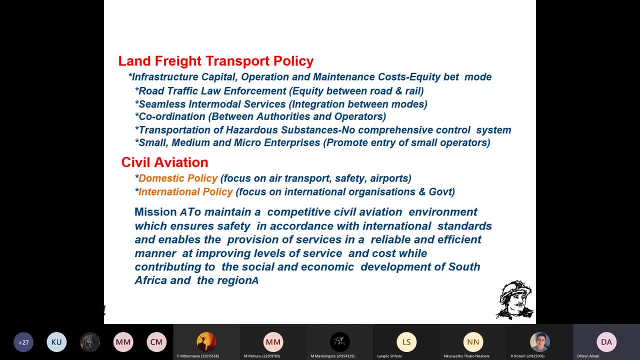 freight. so that's land transport policy, and then we come to a civil mission which is then divided into domestic and international and you can see again safety factors coming in, with international, trying to focus on international organization, and you can see the main factors are mission statement, therefore civil aviation, and again mention of safety, mention of international. 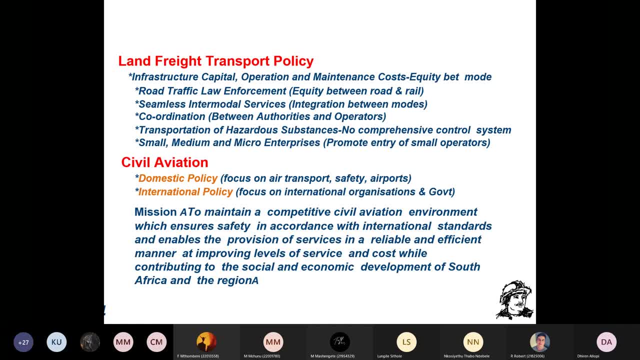 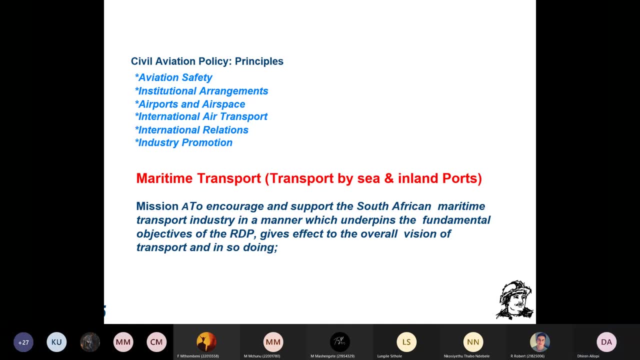 standards providing a reliable physician service. so all the keywords, and again here you can refer to on the safety aspect, the airports, is international relationships and so forth. so i've just highlighted the keyword. you do your notes on the few points on each one of those. so, and then we have relating to water or sea trans. 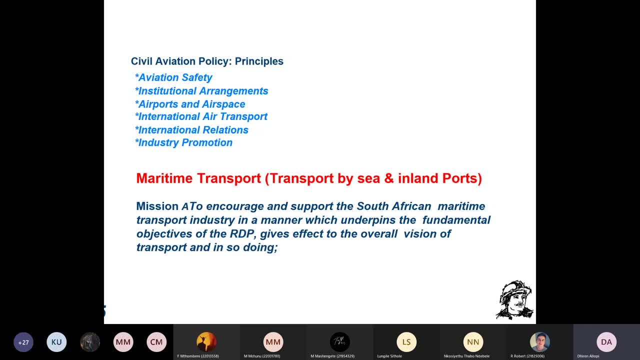 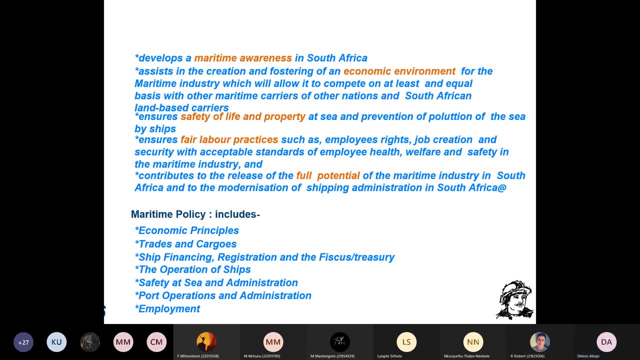 again with maritime, trying to fulfill the rdp program overall vision objectives. and with maritime you can see maritime when it comes to tourism, the awareness of maritime. and recently i've noticed that the national department of transport has made funds available to carry out projects, to carry out research in maritime, so they're now focusing quite a lot on maritime. so uh, 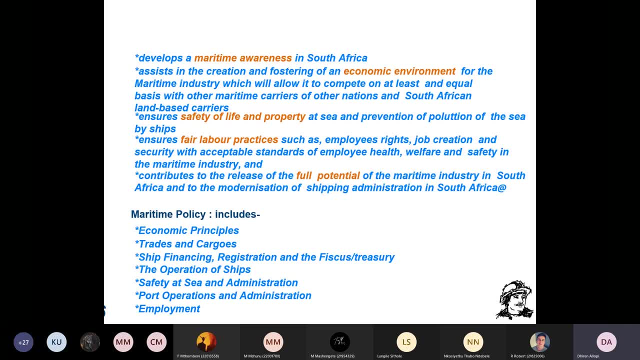 economic development of maritime, safety of maritime and the science. sign the full potential of your maritime industry. you will see that's covered under maritime. go to the through the policy, you will see that the policy does make reference to cargo's financing operation of ships. here see that is covered under the maritime. and again you can refer to the point too that's. 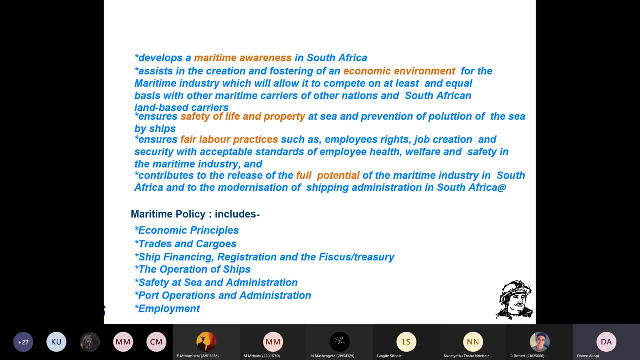 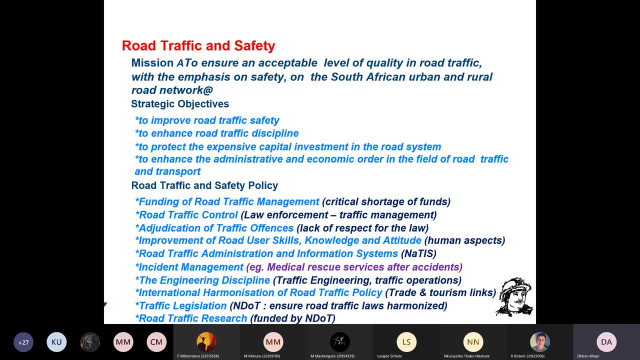 mentioned. and then finally, from the looking at the safety aspect and more road safety. again, a few years back, road safety, traffic safety, was a huge problem. national departments of transport list, priority list. they made monies available again for projects in this area and the main reason for that was due to the high accident rate in south africa. as i said, if you go and try and 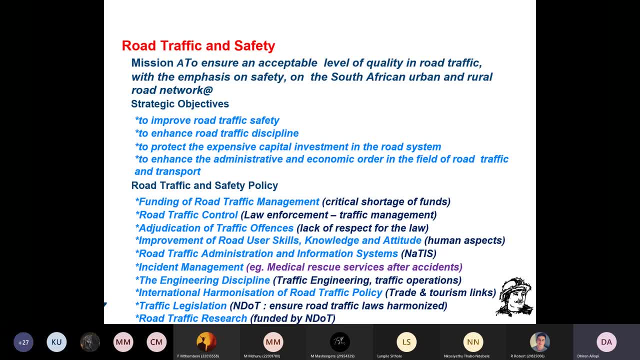 download some of the stats, you will see that one of the worst countries in terms of road safety, very high accident rate, and various initiatives were implemented by the national department of transport, by the provincial as well. do you know what's the national department of transport's road safety? 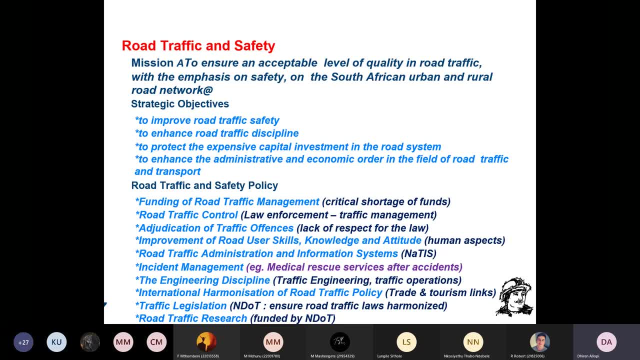 initiative called anyone. what's the national department of transport road safety initiative called? no, heard of the terminology arrive alive. so the arrival life campaign was devised, formulated by the national department of transport, and there are various aspects that they looked at to try and improve road safety, road safety, traffic safety. um province also came up with their own road safety initiative. 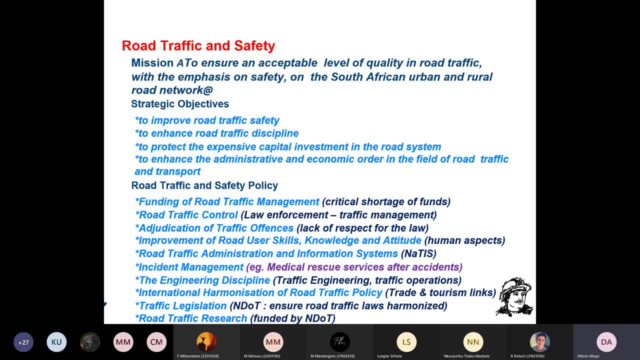 do you know the kzn province road safety initiative? what is it called? anyone came across kz in road safety initiative, heard of as a paper let us be safe. that's the kzn road safety initiative. so you see that the department of transport is trying to ensure that the acceptable level of quality on your roads and that's emphasis, of course being on. 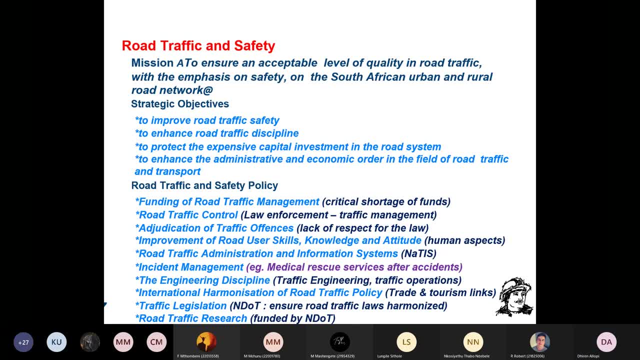 strategic objectives. discipline, you know. again, if i come back to the area of human and driver and vehicle characteristics which i spoke about, discipline comes in. there, comes under the psychological aspects, political aspect, behavior of driver, aggressiveness, drivers under the influence, fatigue, under drugs, so angry problems on your mind. how does it impact on your driving capabilities? 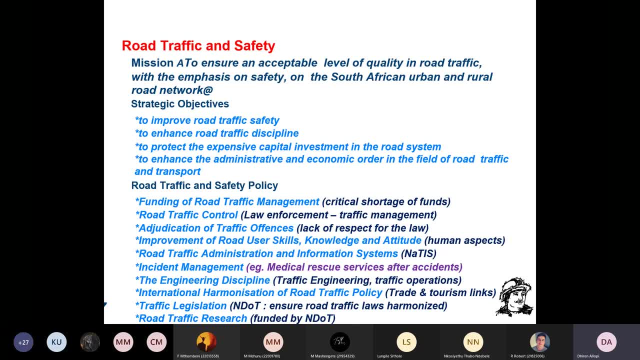 so all that comes. you can see the direct link. okay, so road safety policy, like i said, certainly funding, one needs to make monies available. there's always a shortage of funds. it's always a debate for national and how much to give for transport, for education, water, so forth. so you can see there's only 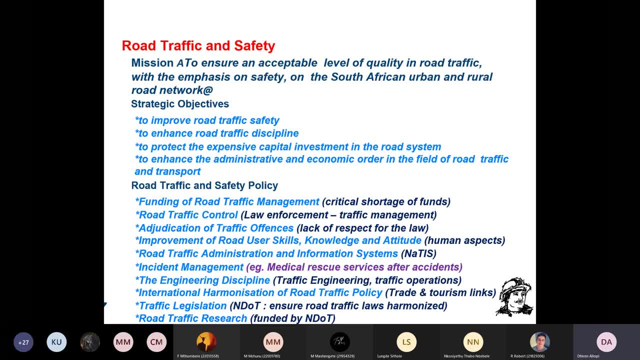 critical techniques, proper law enforcement methods and you can see traffic offenses, lack of respect for human aspects that i spoke about. attitude in terms of administration, the system for administration, administering our road traffic management systems- again, you see the various rescue services that we have in place. engineering discipline: we have various. 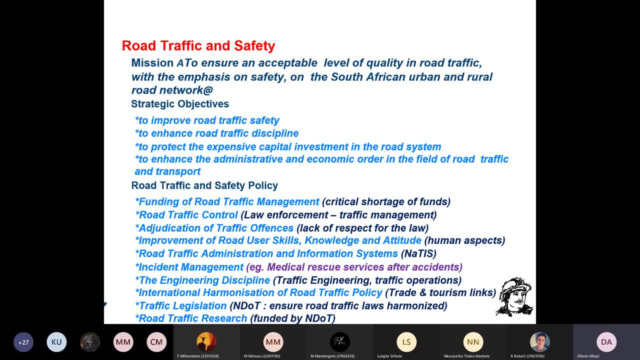 engineering disciplines in place, track place, linking it then to trade and tool in terms of legislation. we have thought to ensure that your road traffic laws are harmful and they of course then pass down to the provincial and then finally at the municipal level and we come to road traffic research. yes, 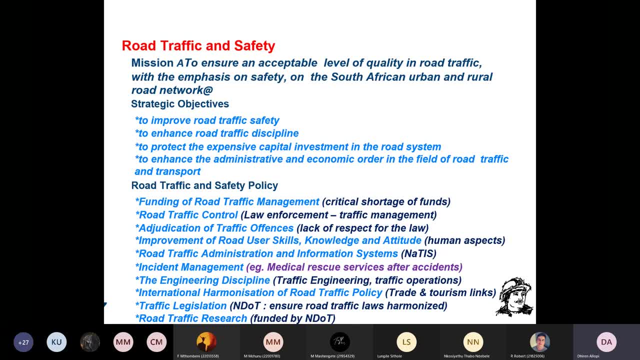 a lot of the funding is by the national department of transport, and you do have other funding agencies also that provide funding for road traffic research. so, yes, that's in a nutshell, then that brings us to the end of module two. so you can see we've covered transportation planning. 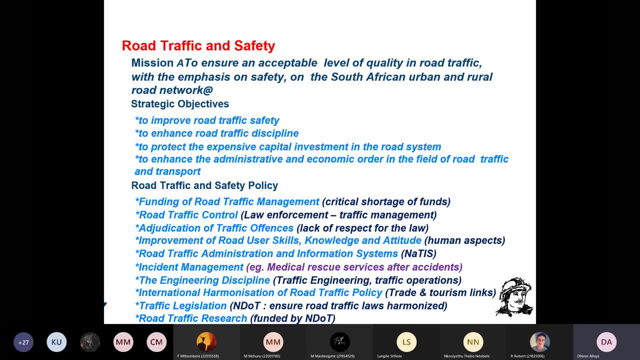 and we've covered module one and two of transportation systems. so we've covered a fair amount of the theory aspect. but, like I said that, the onus is on you to go and refer to Moodle and do a recap, a cross tab between what I have done and what's there in your notes, so you know. 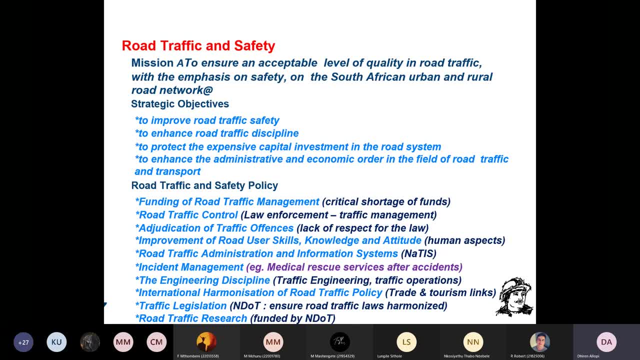 what to highlight. get yourself a highlighter pen and highlight the keywords, the important points, on your notes. in your notes and also perhaps for the next lecture on keep handy writing pad, your calculators. maybe some calculation required that you can do online. so in other words, during lectures it's nice to have some interaction. so 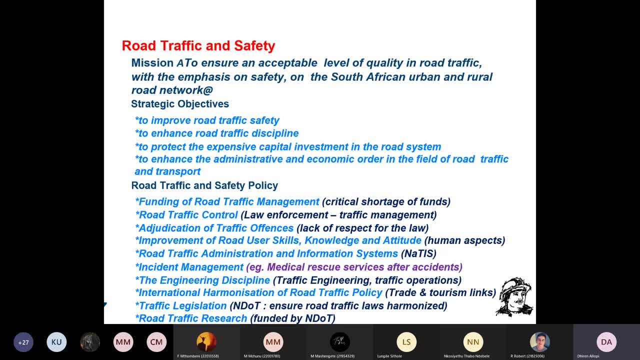 I could pose a calculation and give you five, ten minutes to do the calculation. and when it comes to calculations, I want to emphasize this: please do the calculation. a lot of the calculations, the model answers, the memo are posted on Moodle. but by simply looking at the model answer, looking at the memo, you're not achieving anything. really you're not achieving. 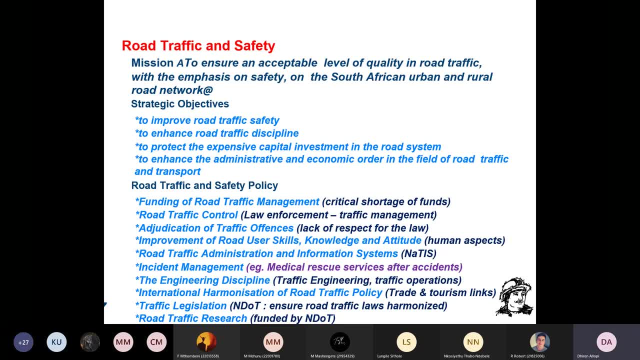 anything, it would certainly be in your best interest to handle the problem. do the calculation on your own. get it wrong. get it wrong, not a problem. then look at the solution and I guarantee you you will not make that mistake, seeing you know, use the right choice after you accept. 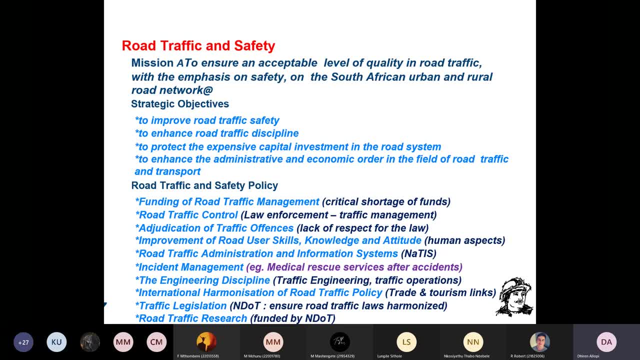 think: what have I got in the tests of my test or the examination? questions in tutorial 1,, 2, and 3 have been covered, So go through the theory questions that's covered in tutorial 1,, 2, and 3.. Look at them. 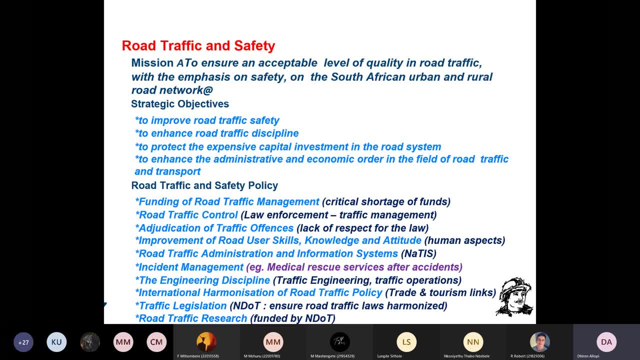 Walk through them. Try and find the solution in your notes first, before referring to the model answer. Like I said, most of the tutorials, the model answers, are posted on Modelo, So I think we've done more than enough for the very first lecture. 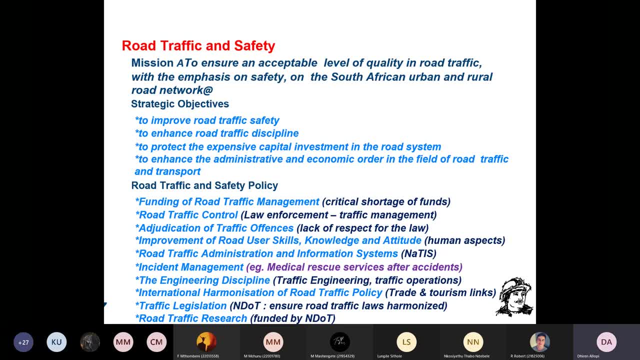 So, before you know it, you will be writing your first test. I have given you the proposed test dates, So please diarize the test dates: test 1 and test 2.. And, like I said at this stage, it will be on-campus tests and it will be during. 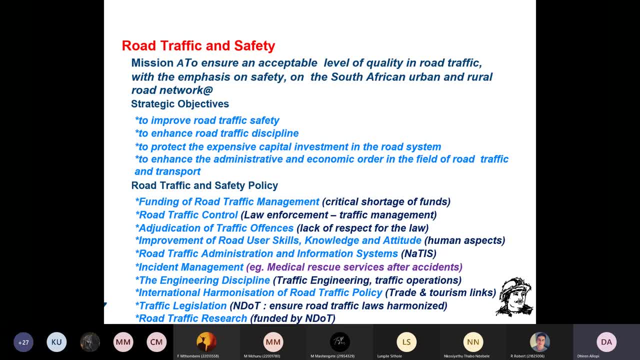 your scheduled lecture time so we don't clash with other tests or with other lectures. That was the reason for scheduling it during your lecture time. So do some work on your own whenever you have some free time, and we will then meet on Thursday. I know your timetable initially showed. 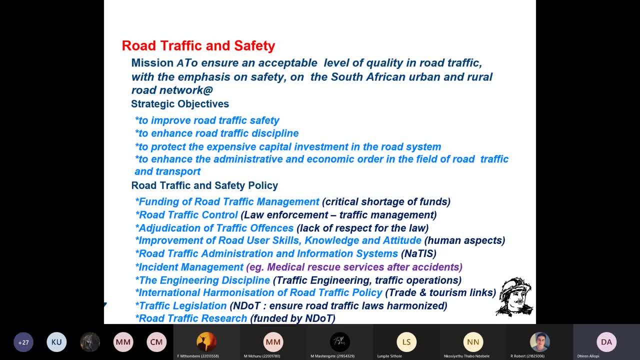 a touch and then a lecture, which I did bring to the attention of the timetable coordinator and he did swap it. You can't have a tutorial before a lecture, so the first period will be a lecture and then the tutorial follows. The tutorial continues, So that could be given to you to do in your own time. 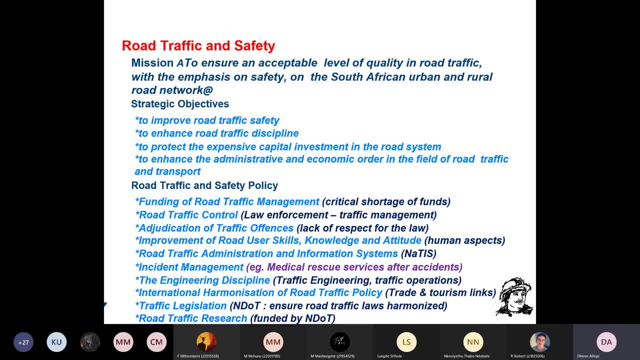 the second period, But in the first period we will cover some work. Okay, I think I've said enough for today. Are there any burning issues, any questions? Whether it's transport related, whether it's department related, If I can answer, I will certainly will. 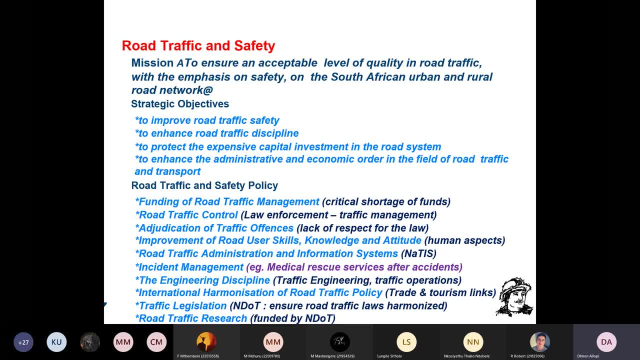 Otherwise I will need to do some research, research and then give you an answer at a later stage if it's beyond my means. any questions, speaking of owners, I know there will be urban structures and water, but what about transport? well, a lot of the transport information is. 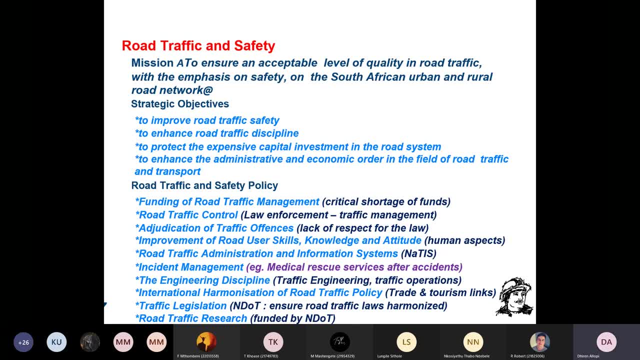 covered under urban. so if you look at the syllabus for urban, you will find a fair amount of transport info covered there under urban. ok, thanks, any other questions? it's also bear in mind that with the owners program it was not really possible to give you every. 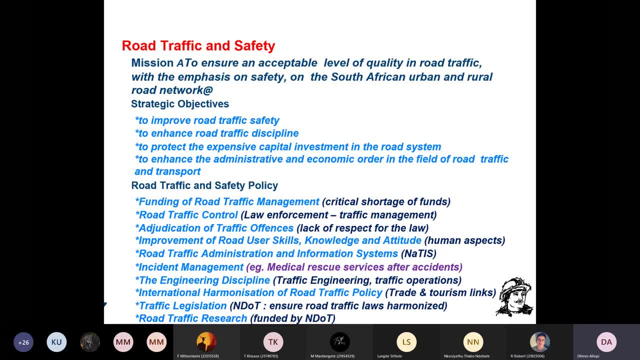 option. when I say every option, every area of discipline, remember the moment you add an additional discipline to this suite. it then means lecturing implications, it means staffing implications. so I think the department has looked at various options and you may find that initially maybe only one option may. 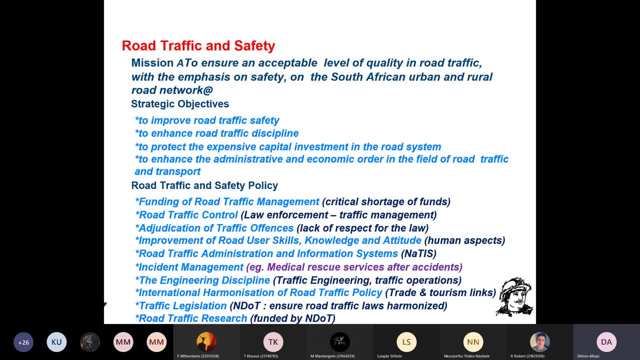 or two options may be offered, and then it could increase at a later stage, depending, as I said, on the staffing capacity of the department. sorry Robert, sorry Robert, you have a question, you had something to say, sorry, so I just wanted to ask: is there no assignments or any work that needs to be handed in? 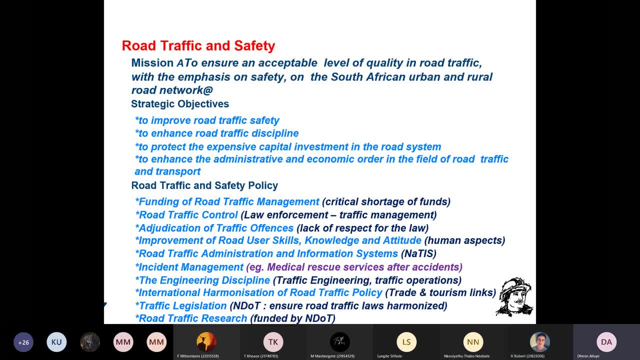 for this module not to be handed in, but you need to now go back to Moodle and do the tutorial one, two and three, the relevant questions that have been covered in these three modules. so you need to go. that that's your basically assignment or homework. you need to go. 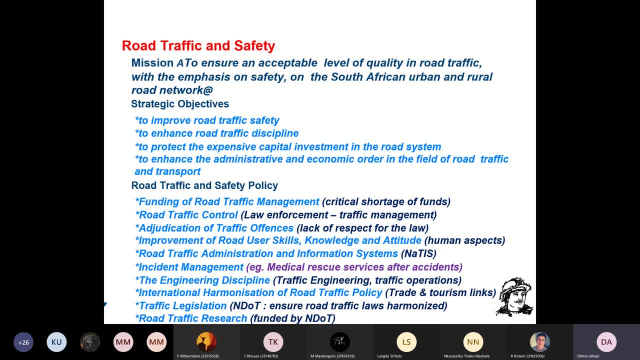 through that and try and find the the solution to it, first in your notes and then perhaps make reference to the memorandum if the memorandum is posted. okay, okay, any other guys? thank you sure, yes, so there is a question. sure, go for it, but it's not related to the modulation. 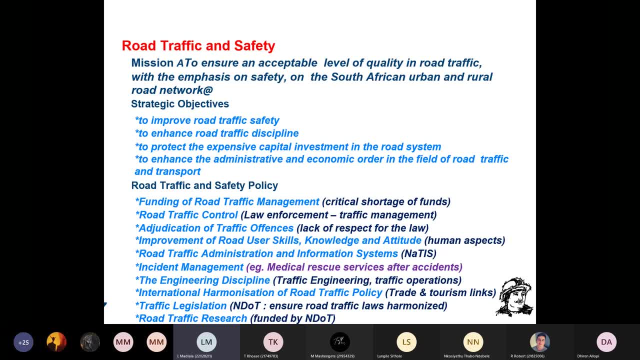 so, um, about the test, yeah, the test one. uh, so we haven't been allocated to our residents or our proper accommodations. so what's going to happen when, at the time for the test comes, and we are still, um, not allocated, well, I'm not sure. but then where are you? 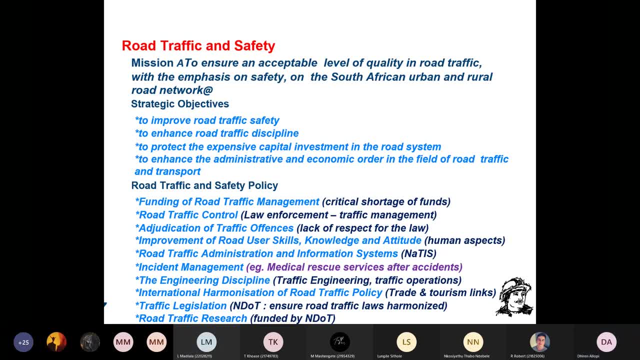 at present? where are you residing at present? oh, um, ladies made so you, you're now currently in ladies man. until I'm allocated, then I'll be at Durban. okay, let's, let's hope that the res issue is sorted out by then. you may need to make some provision, okay. 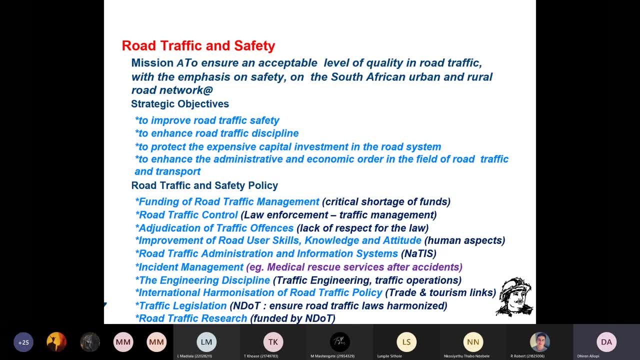 then tell me- I know I am aware that some lectures are face to face on campus. how are you addressing that? at least would transport you to the campus. I know I am aware that some lectures are face-to-face and some are face-to-face, so I'm not sure what you know. 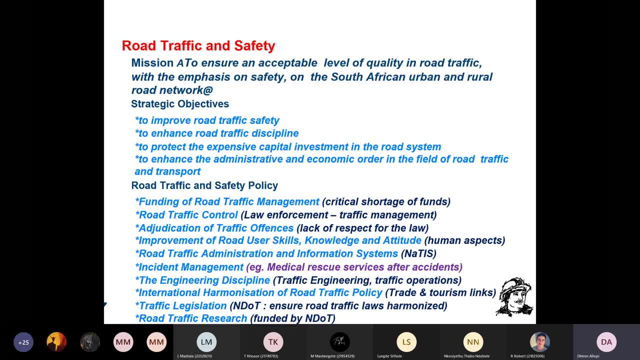 you only have to worry about the assessment on campus lectures. yes, quite, it's obviously convenient for you, since you're a distance away, to attend your lectures online, but I know that there are some subjects that will be having, uh, face-to-face lectures, so you do have a challenge and you, you will. 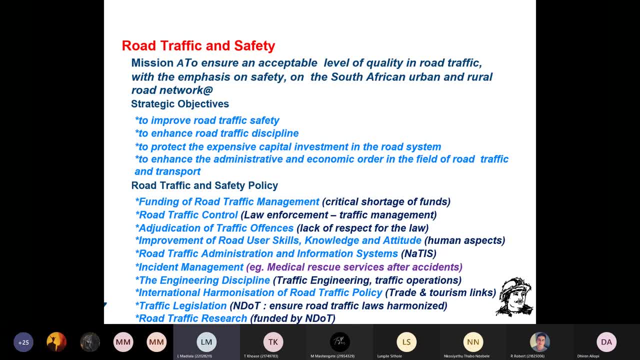 then need to address that as well. yes, I will address it when the when the one has told us that we are going to be on campus. yeah, no, agree, but all the other subjects as well. the assessments will be face-to-face on campus, so, uh, you will then need to to work out. 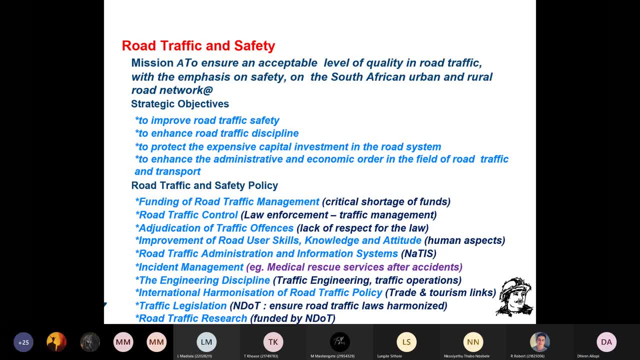 on some program that, yes, near campus, and I just wanted for the face-to-face would have maybe sympathy or something, because right now there's nothing I can do or the other students who are facing one of the same problem really can do. so yeah, like I said, let's see what happens. 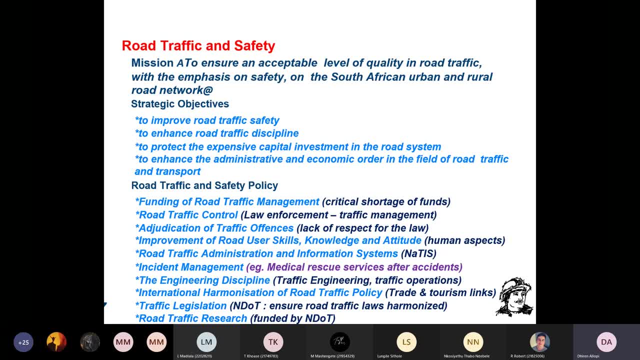 when you're getting closer to that date, you certainly, if there's still an issue with the res, you will have to make some alternative plan. so you will be near campus because bear in mind that it's not only transport assessment tests that will be on campus, it's all the other exit level. 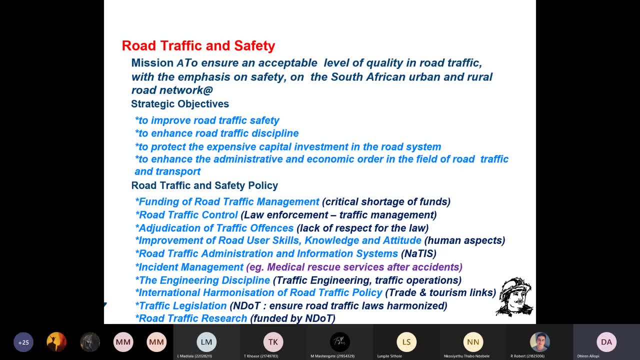 subjects as well where the test will be on campus, some plan that you'll have to make from your side to be able to address that. bear in mind that dut is not a correspondence university. you all know that it's because of the current situation that these specific 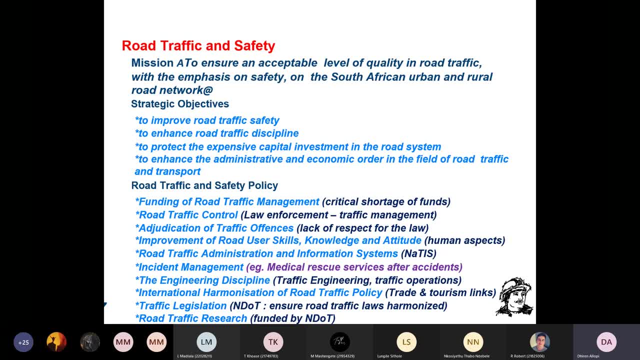 plans had to be put into place, where you now have a fair amount of it, maybe online, but, like I said again, that varies from subject to subject. some- I know this- some lectures that are that have maybe commenced with online and then we'll go to face-to-face lectures. I know there's 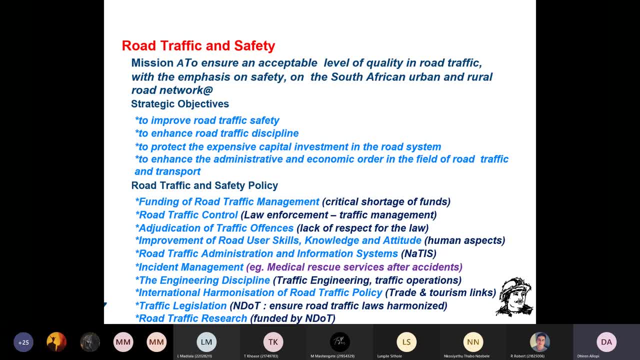 various at the at your exit level. now the onus was on the lecturer, the examiner or subject coordinator to come up with a lecturing and assessment plan, which obviously had to be approved by the department and the office of the team. sir, yes, so do you is your initial plan is. 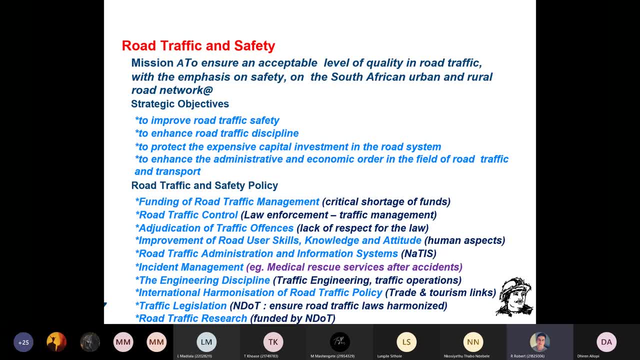 your initial plan, um that we carry on this way until it's possible to get to and campus lectures, or is your plan just online? I think for now I'm leaving it online and perhaps it will stay online and, like I said, some of the major issues relating or factors relating to 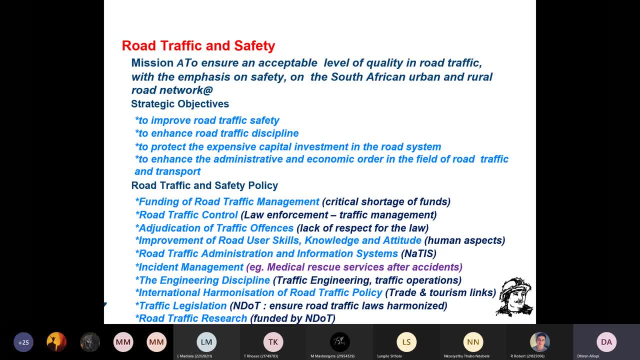 online. certainly one. I'm not sure when the vaccine situation will be fully at risk. 100, but certainly the venue is going to be a big one for us. certainly the venue is going to be a big one for us. the venue issue is also quite a critical issue in terms of satisfying covert requirements, that is. 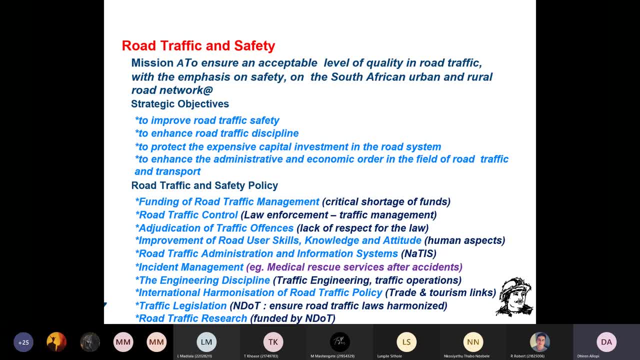 the 50 venue capacity. that is quite an issue and certainly you don't want to go against that. you found that you're packing your venue to capacity and not abiding by the 50 rule. then you can run into serious trouble for that. okay, thank you. okay, if there's no more questions in.